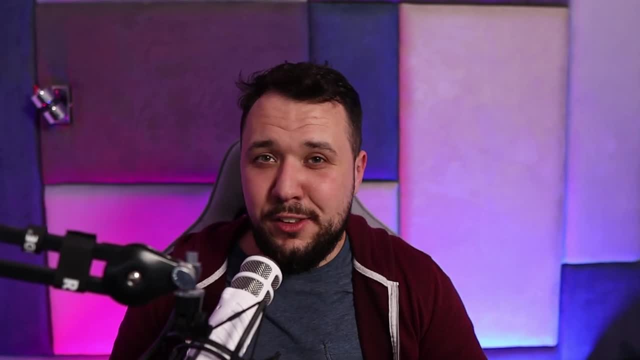 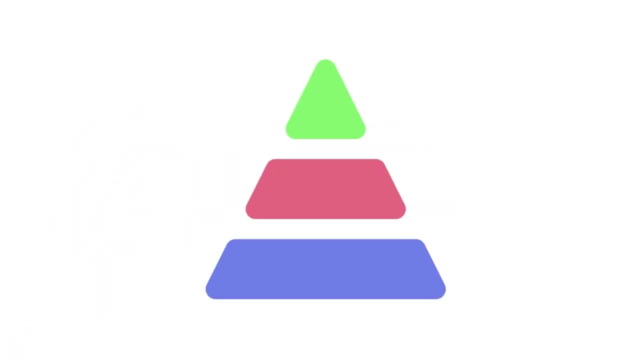 the best testing strategy And for the longer answer, let's take a look at the visualization of the testing strategy. Let's start with the testing parameter first. This one is a typical testing parameter that consists of unit tests, integration tests and end-to-end testing. The tests are ordered: 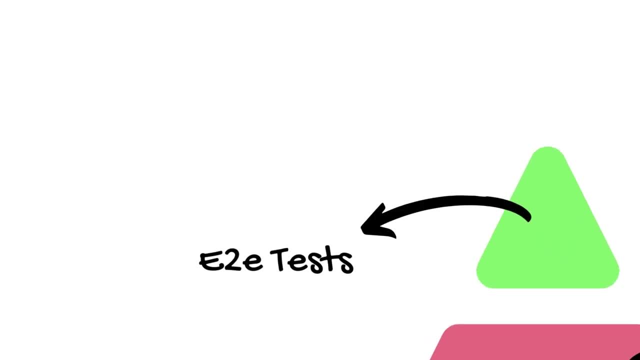 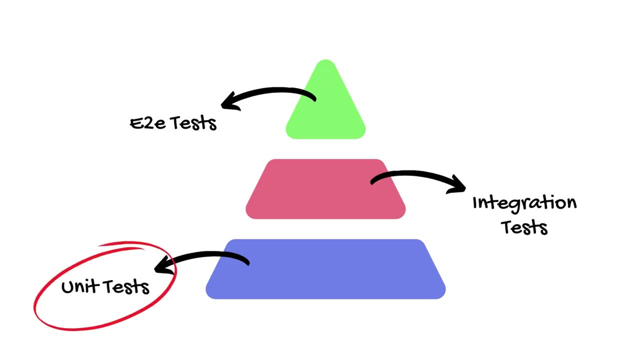 based on their scope and execution time. The closer we are to the top, the longer the tests take. but they also give us more confidence. Unit tests form the base, as they are quick to run and pinpoint specific code issues. Integration tests come next, validating the 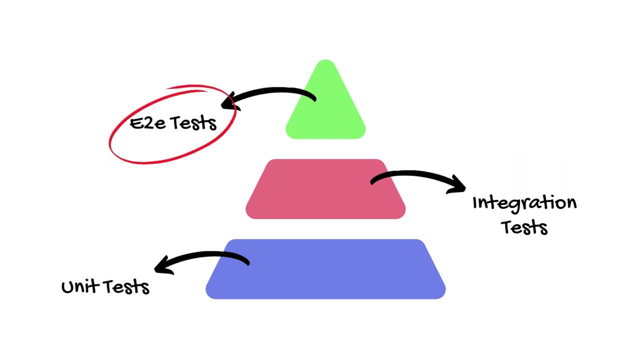 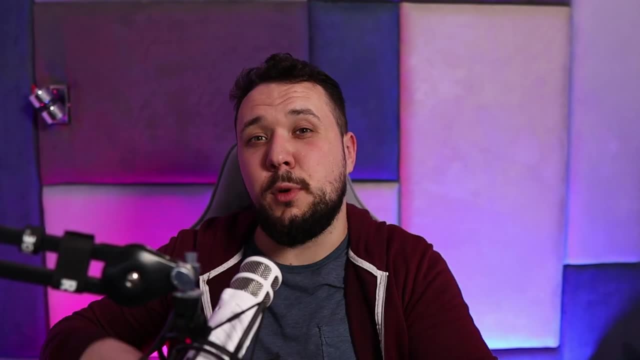 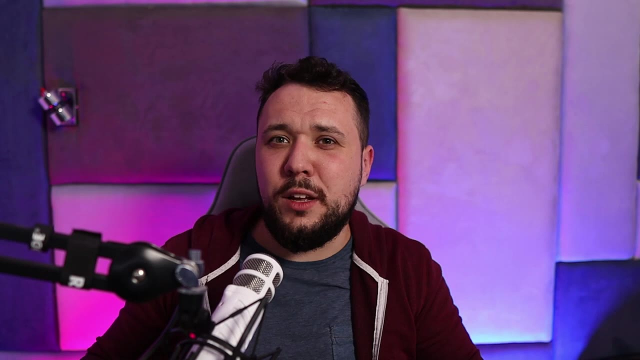 interactions between units. End-to-end tests with a broader scope are placed at the top. So long story short. end-to-end tests give us the most confidence, but we cannot fully rely on them because the feedback loop would take way too long And this would affect the 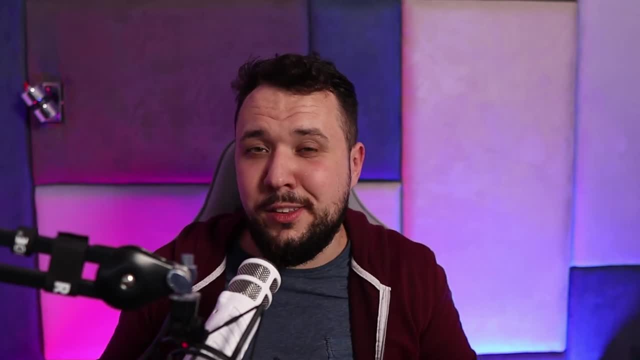 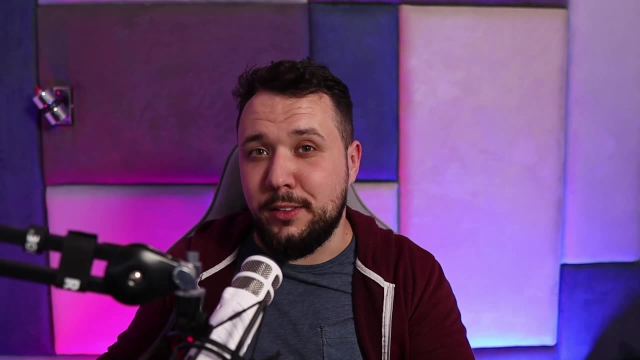 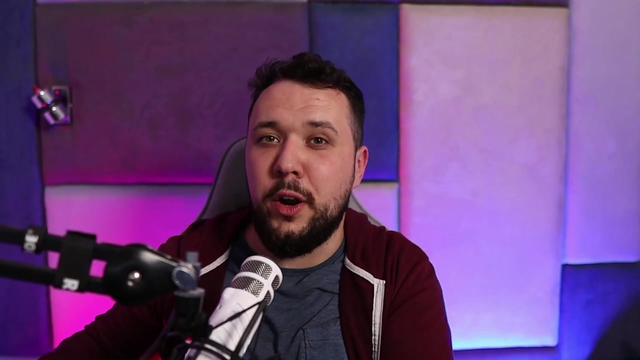 development process. so we usually make concessions and add more integration and unit tests. Ok, but finally, which of these two should we pick for Web Client? In my opinion, integration tests, Integration tests- Whenever we are talking about the logic responsible for querying external API, we need to make 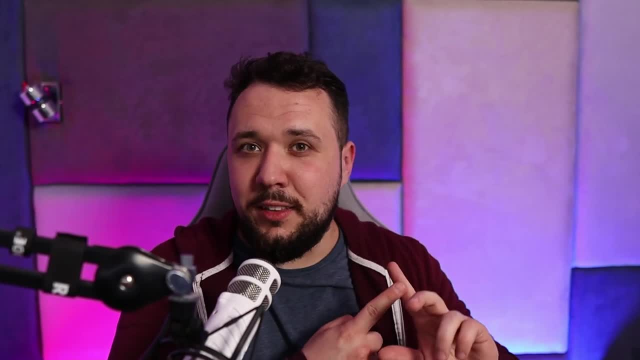 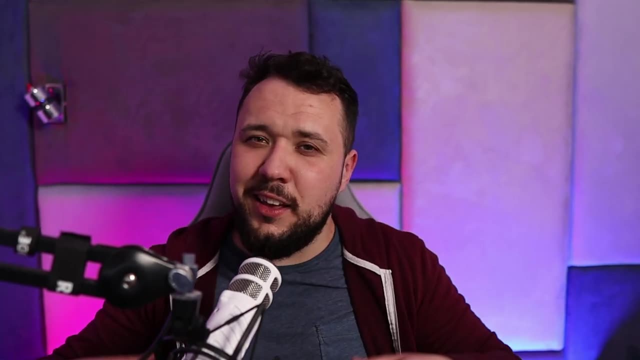 sure that we query the appropriate URL, the appropriate headers are sent and query parameters as well, request response bodies are properly serialized and deserialized, and many, many more, And in my humble opinion, with unit testing the amount of mocking would be so significant. 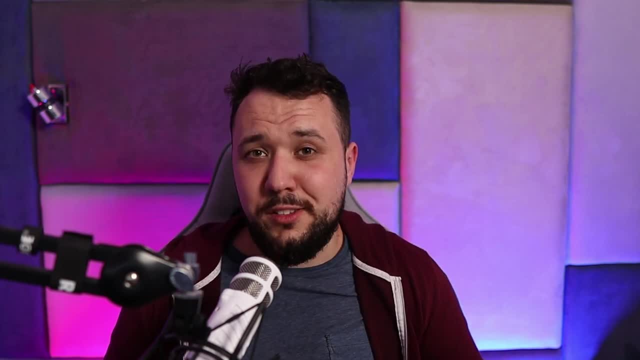 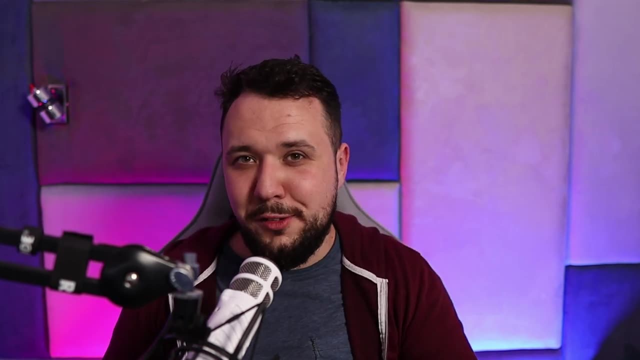 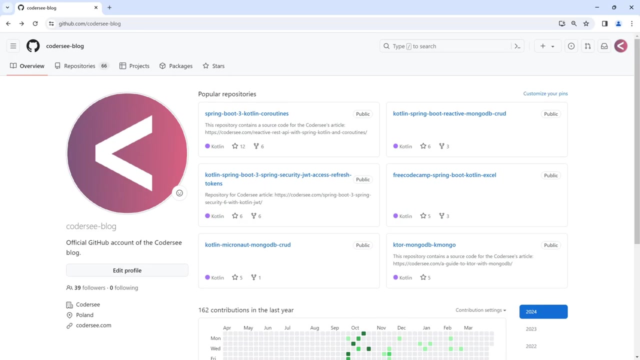 that I would personally question whether we need such a test. Moreover, in Spring we can write integration tests for Web Client with Wiremock at almost no cost, But of course, this is my personal opinion and I will be happy to hear your thoughts about that in the comment section below. With that said, let's set up the 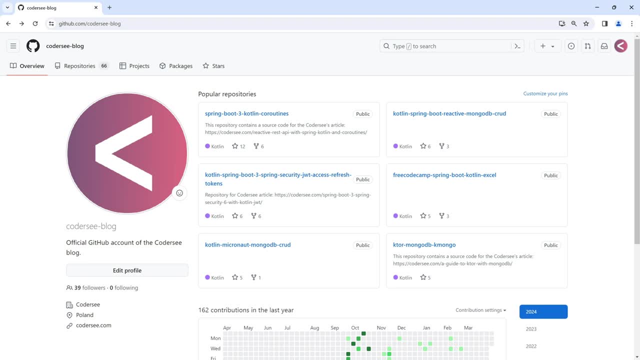 API key we'll use to query the GitHub API. Technically, the endpoint we'll use does not require any token. However, for the learning purposes, I want to show you how to deal with passing better tokens too. So, as the first step, let's navigate to the tokens tab. So let's click. 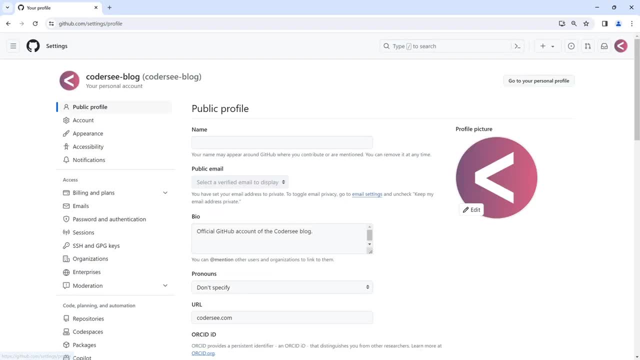 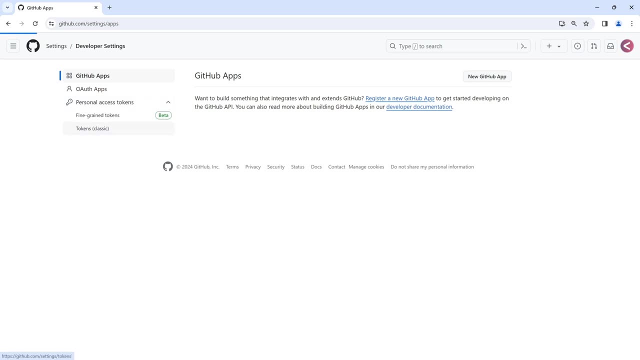 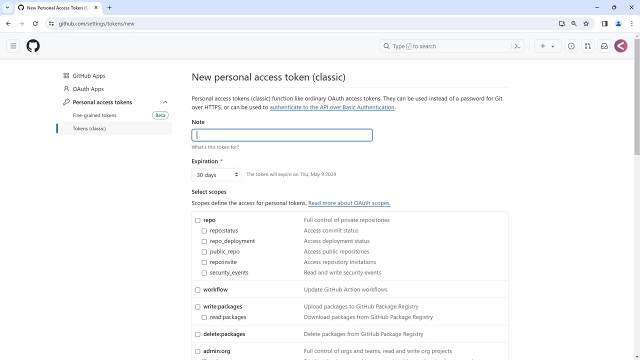 on the logo. right here, Settings. Scroll down a bit to developer settings. Click on the personal access tokens: Tokens- classic And right here, generate new token. We'll use the classic token As a note. let's call it whatever. Expiration I will set to 30 days and I will not select any. 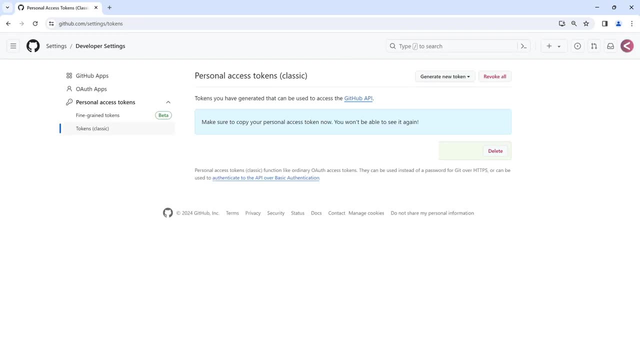 scope. So let me generate the token And right now you can see the value right here. Please note that the value is set to 30 days And right now you can see the value right here. Please note that the value is set to 30 days And right now you can see the value right here. Please note. 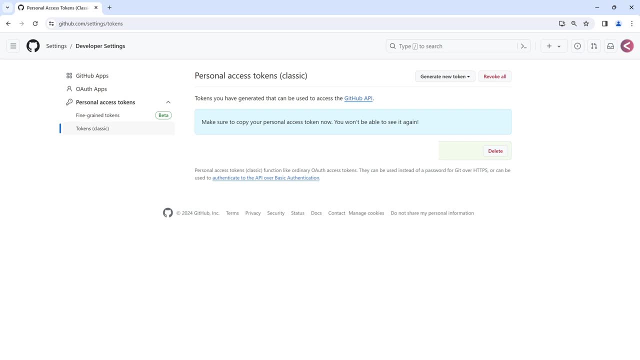 it down, because we will need this later. Of course, do not share this value with anyone. Regarding the scopes: if you don't know what scopes you will need, always follow the principle of lowest privilege. At the end of the day, we can generate a new token at some point in the future. 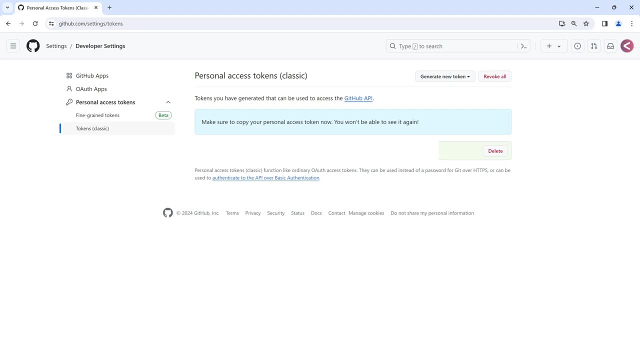 when the requirements change. Excellent. as the next step, let's prepare a simple project responsible for querying the GitHub API. Long story short, we'll implement WebClient with coroutines that will query the list repositories for a user endpoint. Let's check out the GitHub API documentation for more details. 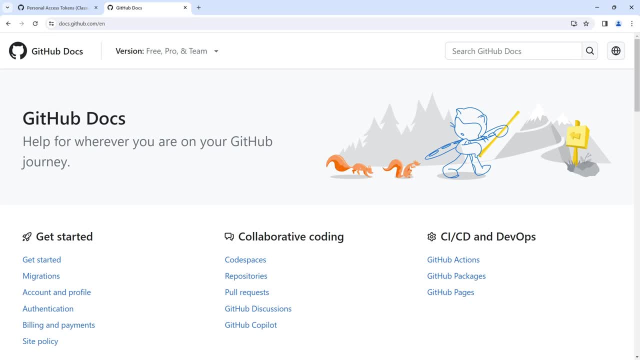 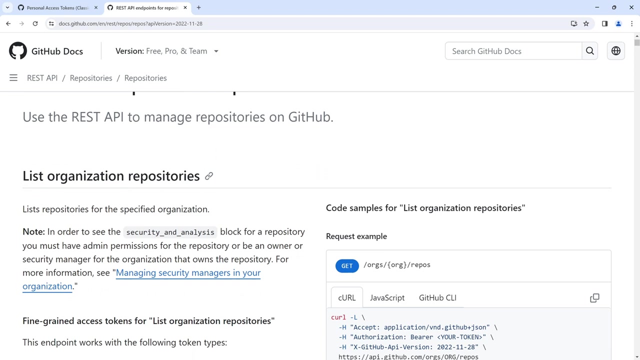 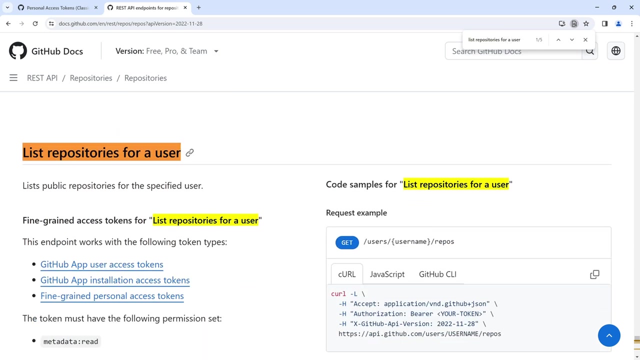 And right here in the search bar, let's search for list repositories for a user. List repositories for a user. Let's hit enter and let's click on the first one. Wonderful, Now control plus F list repositories for a user. So right here we can see the endpoint. 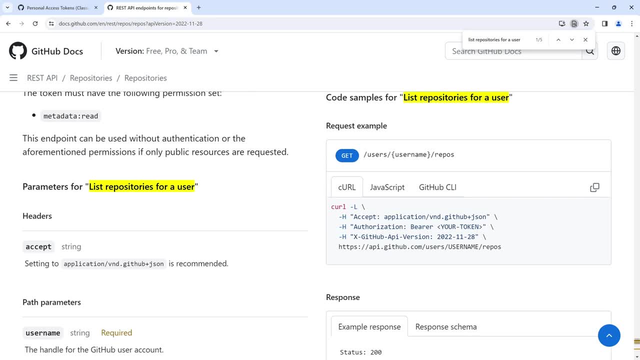 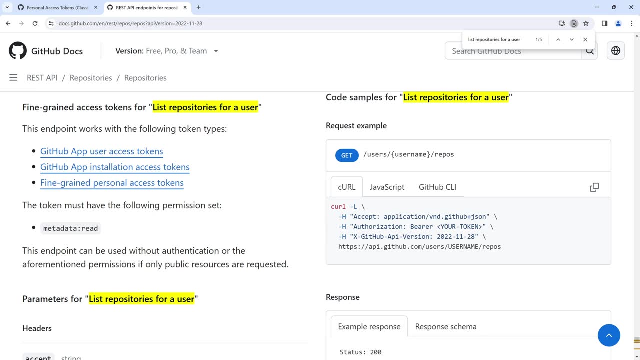 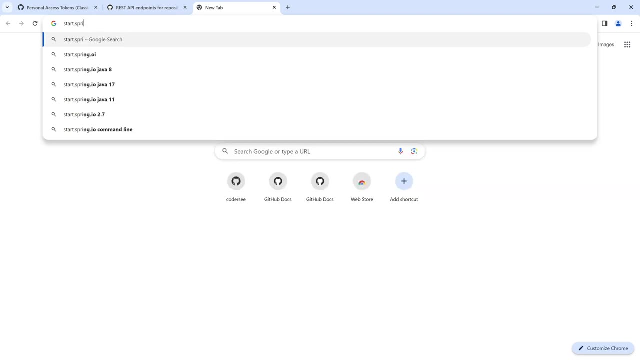 that we are about to query. If you are interested in more details, you can find them right here. Anyway, let's generate a new project, Spring project. So, in order to do that, let's navigate to startspringio page. Start Spring. 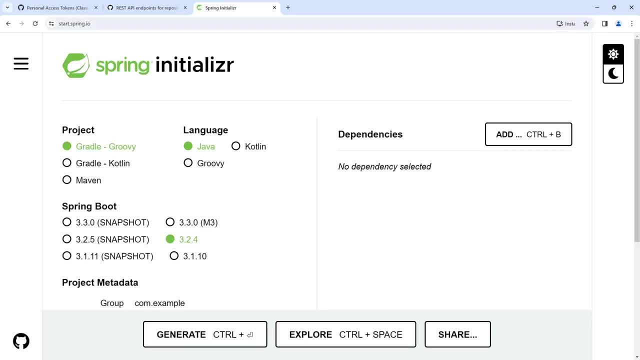 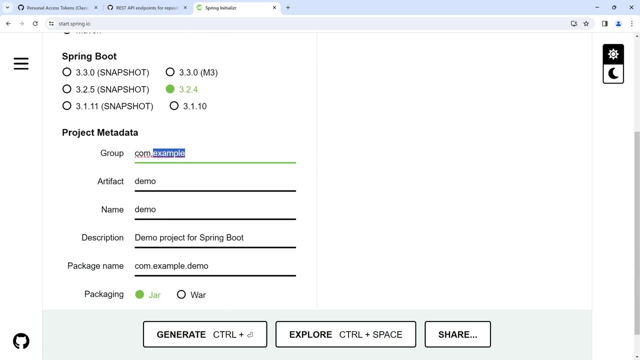 And on this page. this will be a Kotlin project, of course, So let's select this one right here. Language will be Kotlin. Spring Boot version will go with 3.2.4.. When it comes to the group, I will change to concodrc. 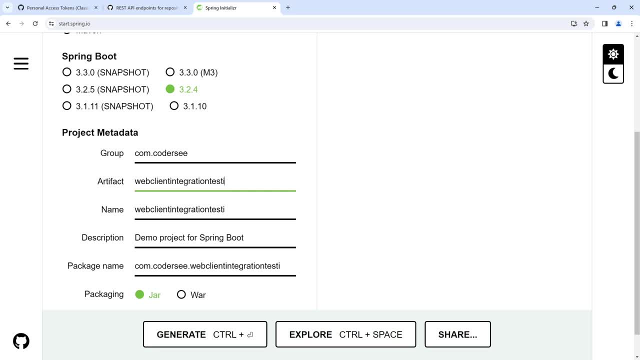 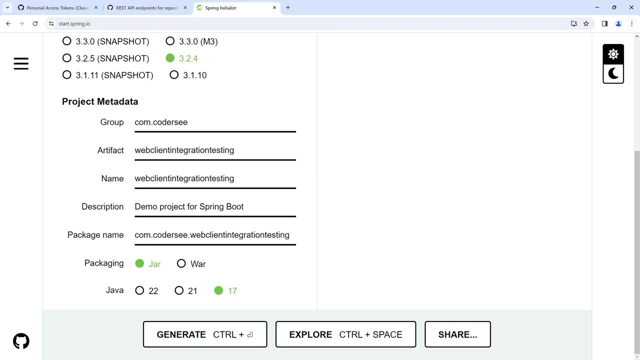 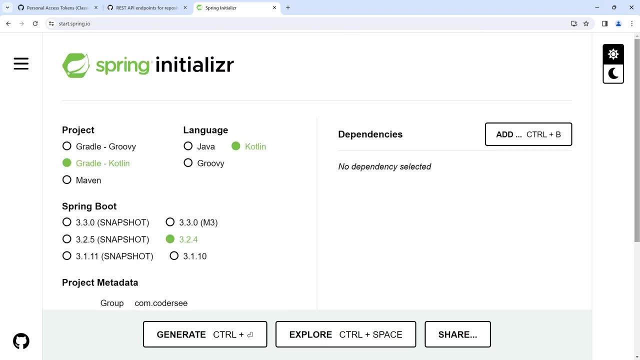 WebClient integration testing, for example. You can put whatever you want right here: Description: let's leave it as it is. Packaging will be jar And Java version: let's go with 17.. Lastly, let's add the dependency. We'll add Spring Reactive Web That will need to work with. 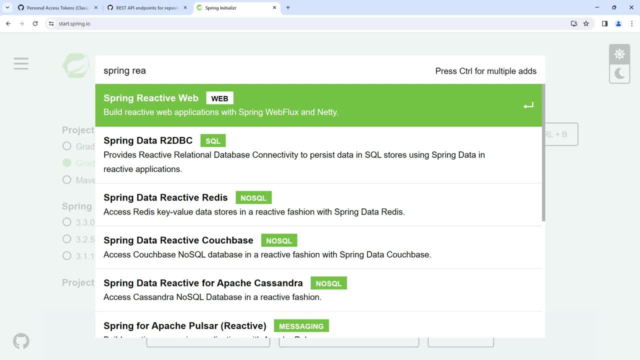 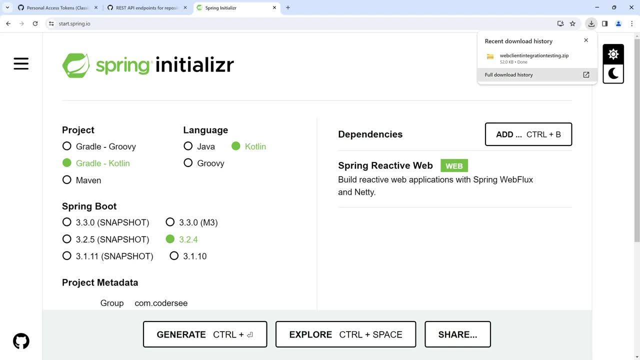 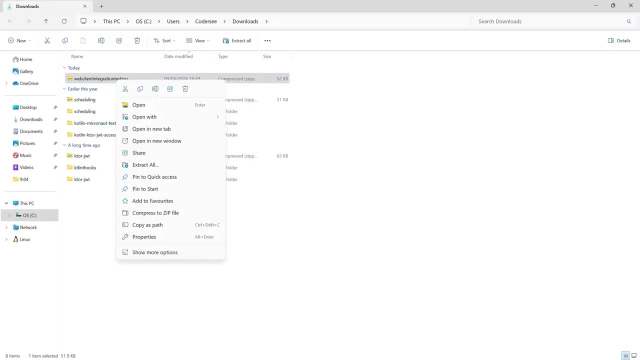 coroutines I mentioned in the beginning. Spring Reactive Web: Wonderful. Let's hit generate And zip package will be downloaded which right now we would like to extract. Let's navigate to the folder: Excellent. Let's click right mouse button: extract- all extract. 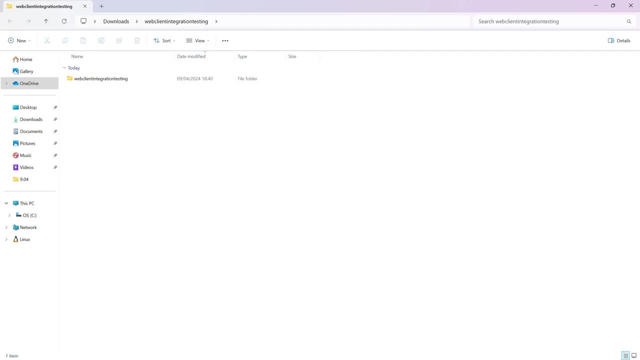 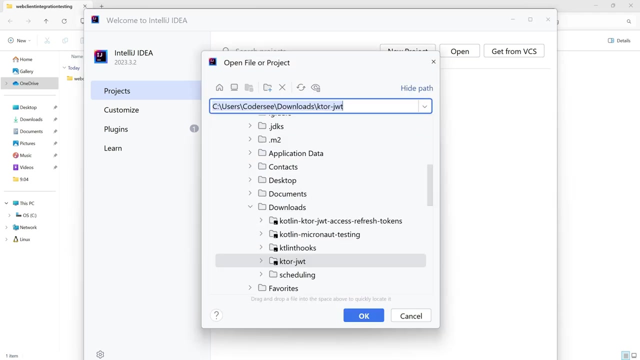 Wonderful And as the next step, let's open up our favorite IDE. I will be using IntelliJ IDEA Community Edition, So let me search for IntelliJ IDEA And right here I will have a chance to open up the project. Let's hit open downloads. Let me refresh that action. 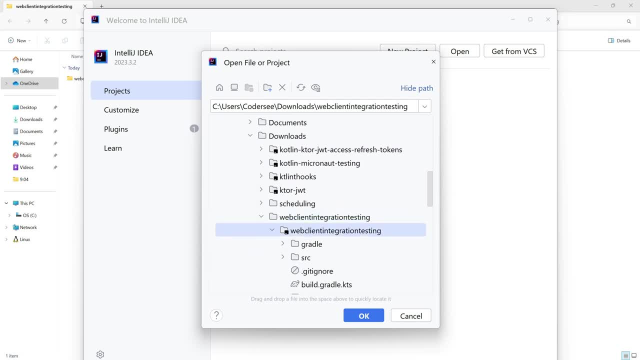 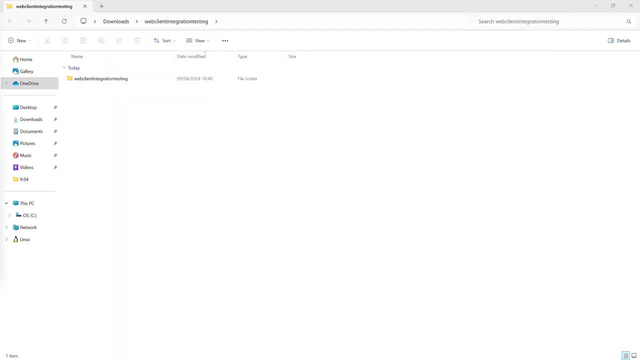 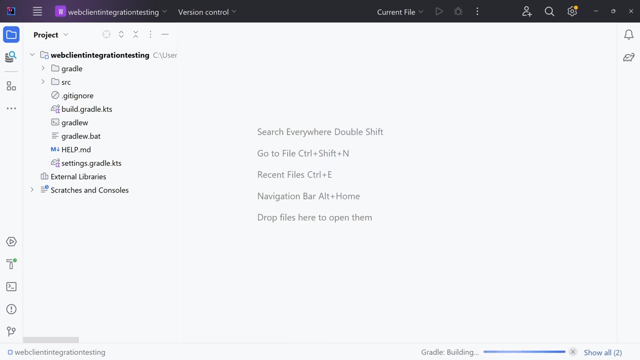 web client integration testing. Let's click on the folder with this black icon. Let me hit OK And IntelliJ will open up the project. Right now the project will sync. Gradle will try to fetch the necessary dependencies. Right here in the bottom we can see the progress bar. 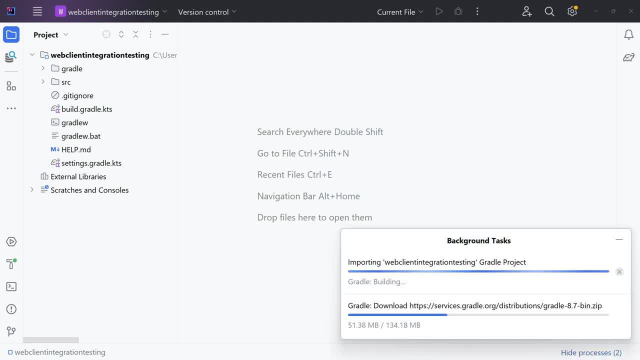 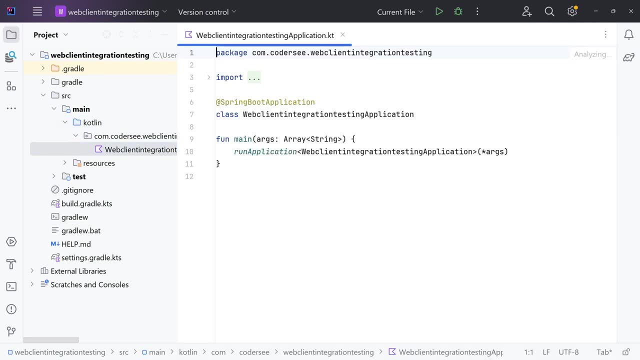 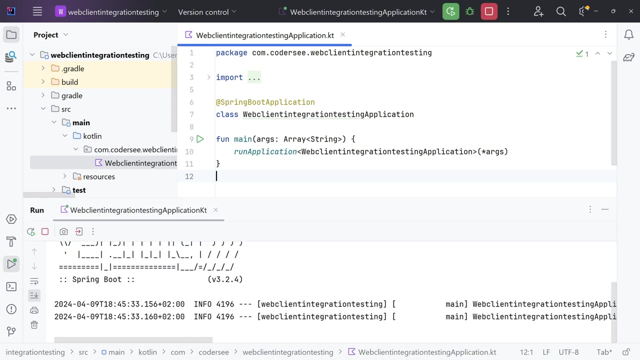 If everything finishes successfully, we will proceed. so When the project is synced successfully, let's navigate to the main Kotlin and let's open up the web client integration testing application. Let's run it to verify that this is working. fine, Wonderful. We can see right here that. 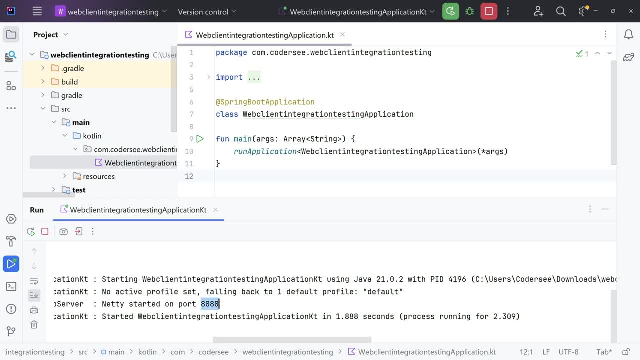 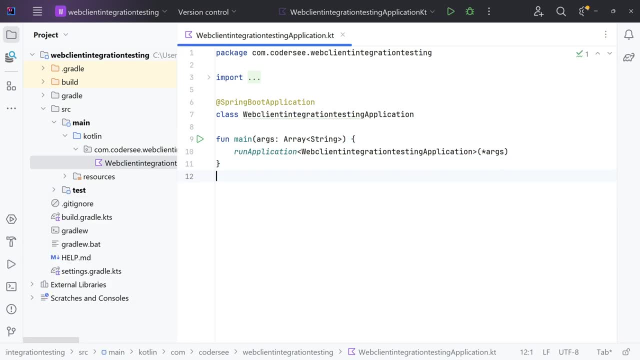 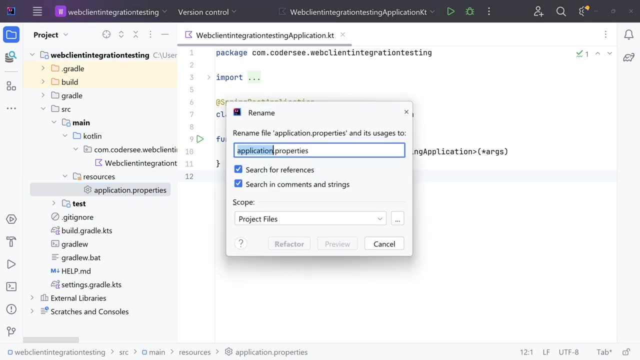 the application started and NetEase started on port 8080, which is the default one. Wonderful, Let's click this one. Let's stop the application And, as the next step, let's navigate to the resources and let's convert the application properties into the YAML. This is my personal preference. 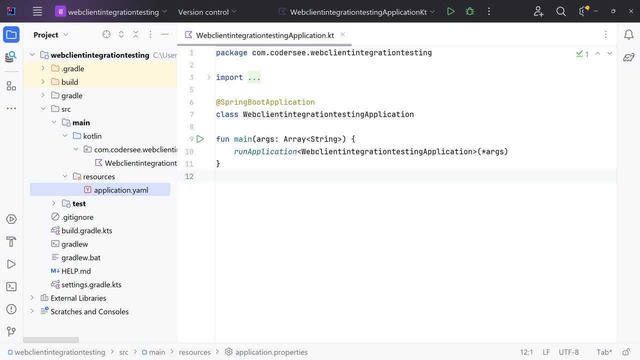 Instead of working with the properties file, I prefer YAML files. Firstly, let's convert this one to the YAML Spring Application Name and right now we'll add three properties for Github key url and version API. Github key url and version. 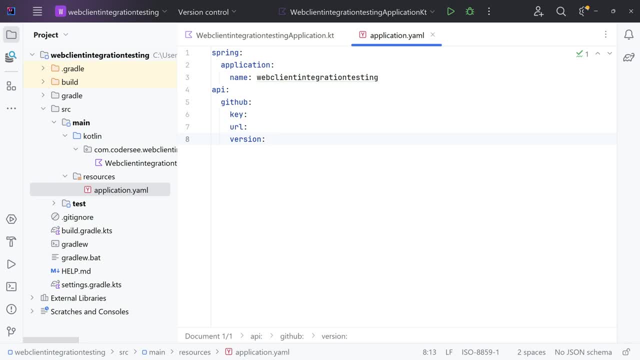 For all of these values. I would like them to be sourced from an environment variable and will provide a default version. Let's get started. Let's go to the application and let's start by value. so let's start with key and let's call it, for example, github API token. 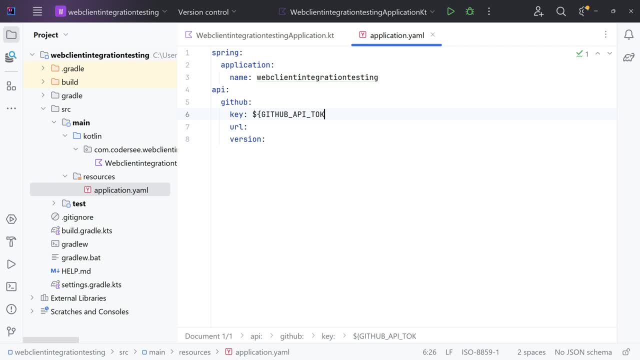 github API token and the default value: 1, 2, 3. similarly for URL: github API base URL and I'll default that to localhost 8090, HTTP. localhost port 8090. lastly, let's provide the version for github API: github API version and the. 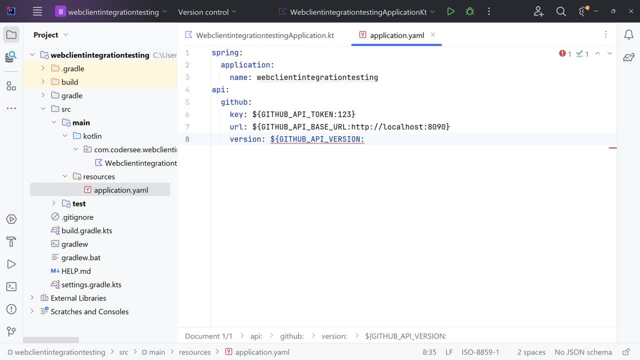 default value. I would like to be 28th of November of 2022, 2022, November of 2022, November 28th- wonderful. so basically, this approach is not only secure because hard coding the key with token value would be the worst thing we could. 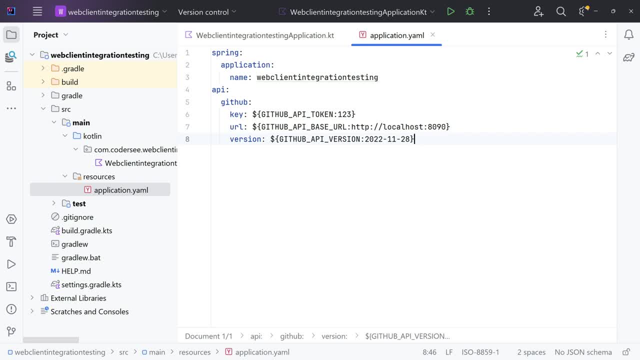 possibly do, but also flexible. we can pass different values depending on the environment that we are writing our app in, whether this will be tests, UAT or production, we can provide that as environment variables. wonderful following: let's configure a web client bin that will use the github API, github API version and the default value 1, 2, 3. similarly for 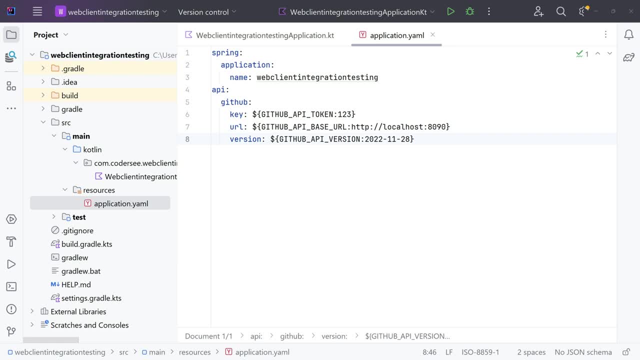 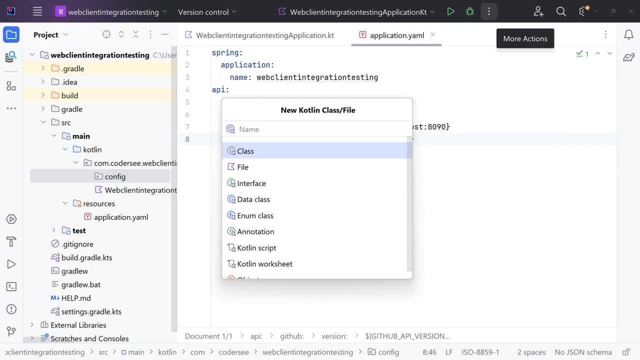 vertical storage. let's call it 824. soon we'll specify event aprender, which we are going to use whenever we want to call the github API. so let's add the config package. let's click right here, right mouse button, meal package called chic. again right mouse button on the config package, you cutting class and 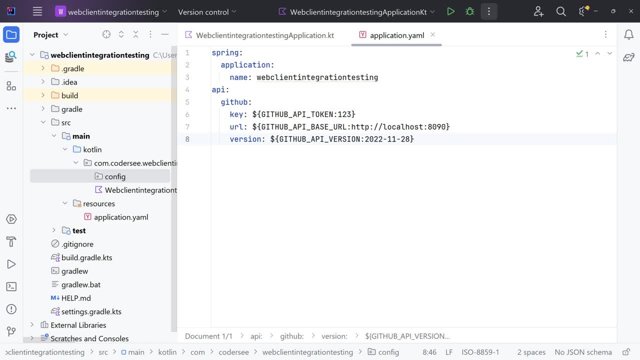 let's call it github api properties: gii'd have up. sorry, I've api properties, wonderful, and now we should be able to boot back. remains: we actually haveита quick and it's okay to use this. wouldn't 의� персонLife lue? i am okay, and I'm neighboring, we will. so we need the highlights to use whenever we want to call the github Cookie. so let's add the journey packet. so let's click right here, right most button, your package called config. right here right mouse button, your package call config. again right mouse button on the config package, your cutting Los. and let's call it github API properties: github up, sorry για. 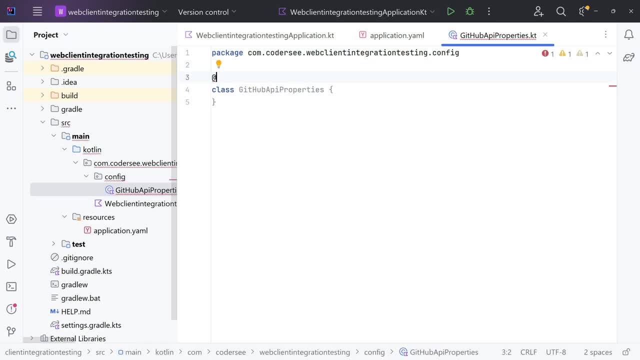 And let's annotate this class with configuration properties- annotation, Configuration properties- and right here we'll provide the path that we'd like to reference in the application YAML. In my opinion, this is the cleanest way to inject values from properties and, as we can. 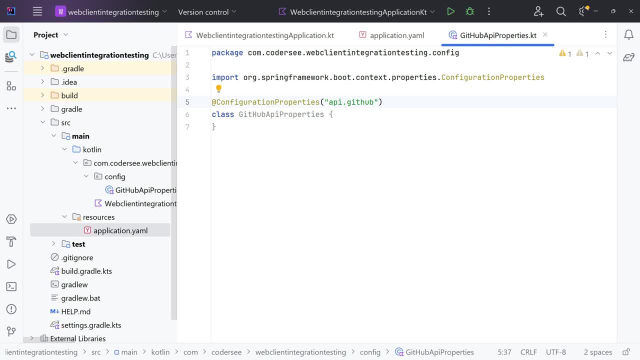 see above, we simply provide the prefix and field names simply will be later mapped to the particular fields. Nevertheless, the next thing we need to do, let's convert that to Kotlin data class And let's provide the names for properties: val, url, string, value. key will be the string. 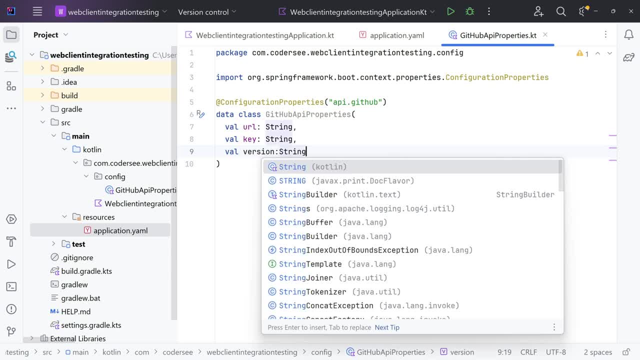 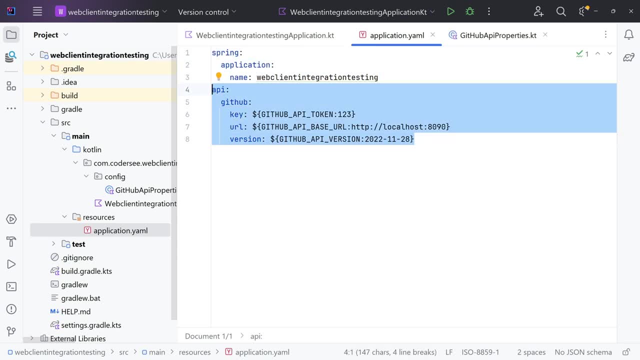 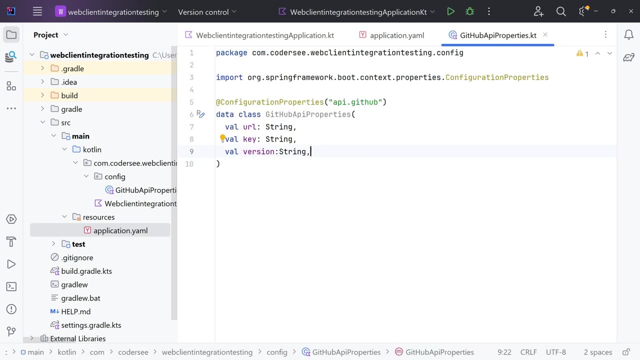 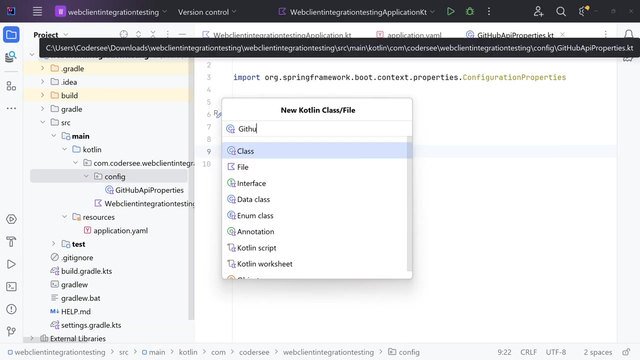 value as well, and version will be string value too. So again, As you can see that this will be mapped to the values from our API, from our application YAML file, As the next step, let's add the GitHub API config class- Config right mouse button Kotlin class- GitHub API config class. 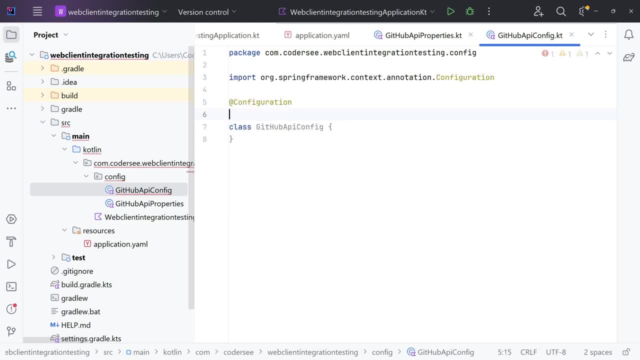 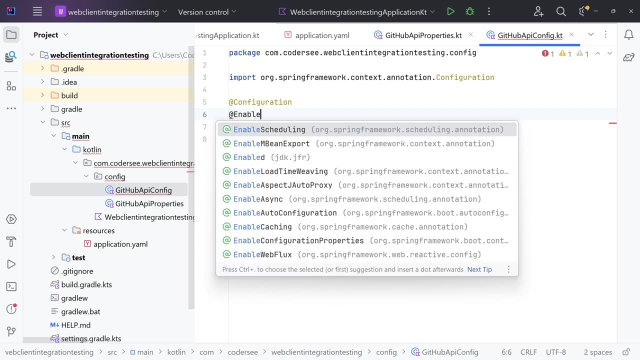 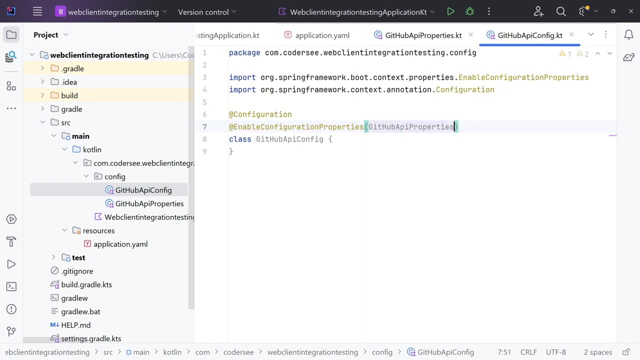 Let's annotate that with configuration. first And secondly, let's enable configuration properties. The previous class will be working, Enable configuration properties, and we need to provide the name of our class, so GitHub API properties class- Excellent. Next, let's introduce the web client bin. 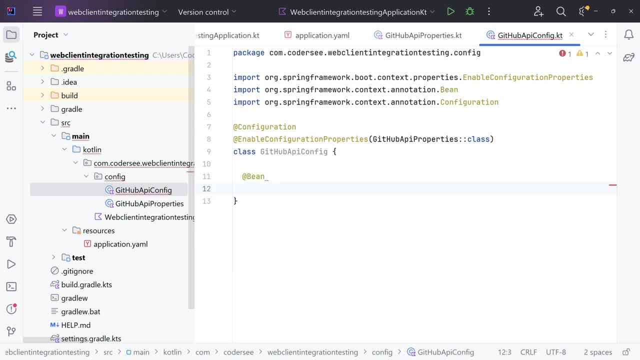 So, firstly, let's use the bin annotation and let's add a new function called web client. This one will take one parameter: builder. Let's add it, And this will be web clientbuilder type. Let's import, Alt plus enter. Let's import the class, and I would like this function to return a web client instance. 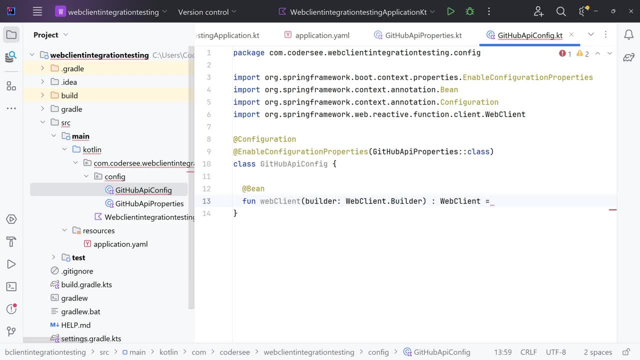 Web client instance, as the next step equals control alt plus l to format the code. And next we would like to instantiate our web client. So I would like to provide the base URL from GitHub API properties And I would like to create a web client. 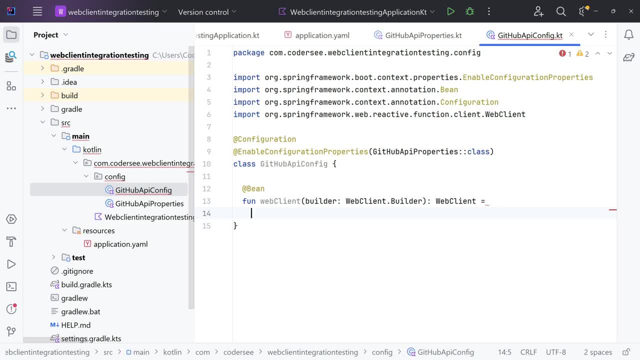 So we need to inject them. Let's add a constructor Private vault GitHub API properties. This way, we'll inject those values. We'll be able to reference them. So builder dot base URL. As a base URL, let's provide a value from the properties dot URL. 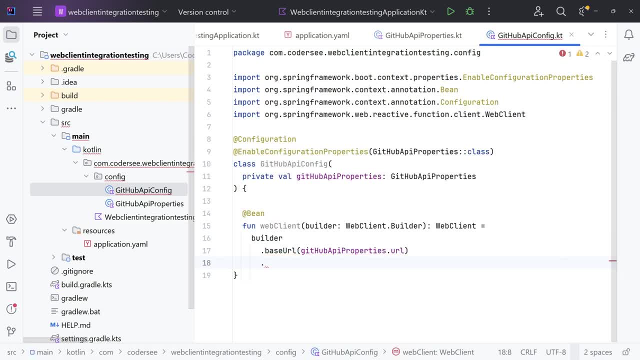 Next see, We'll add the authorization. So we'll add the authorization Header, will pass the bearer token And again this value will be sourced from the properties as well. Default header: The header name will be authorization And the value will be bearer. 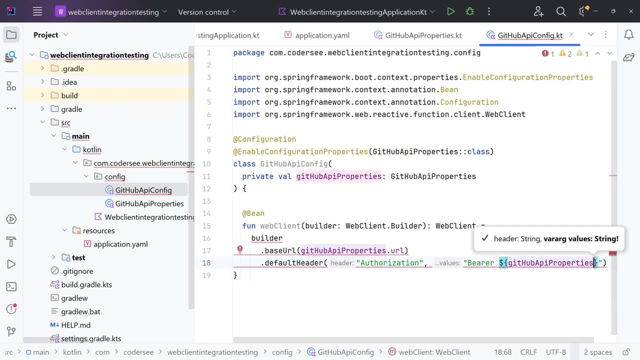 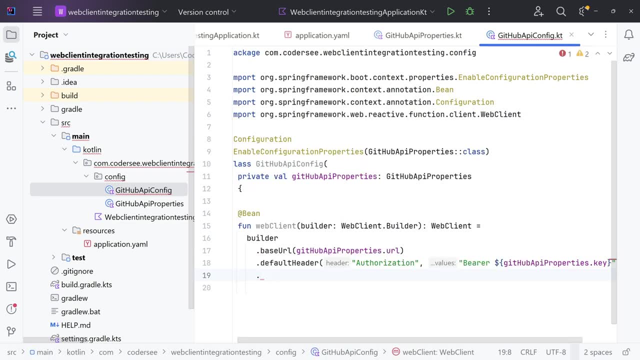 And right now, let's use string interpolation and access the value from GitHub API properties. We'll use the key. Nextly, I would like to provide the API version Default header X- GitHub API version And as the version: GitHub API properties- dot version. 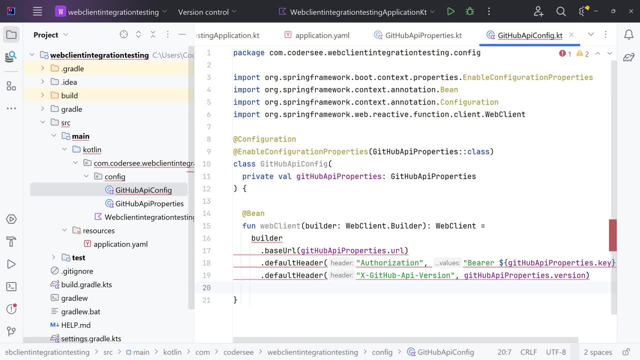 Lastly, let's add the accept headers And we'll provide the default headers: Default header. Default header. Default header: sedan-tv-login. Accept And application: slash vnd, Github plus JSON. And if you see this value for the first time, don't worry. 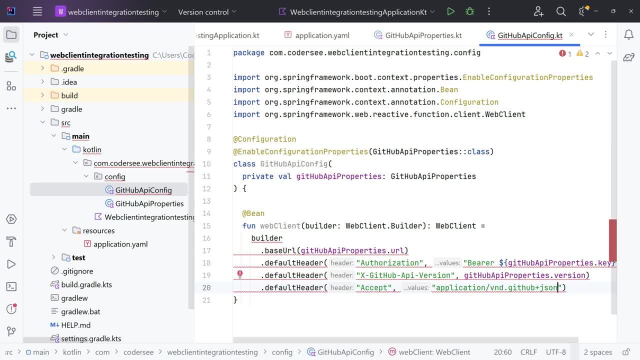 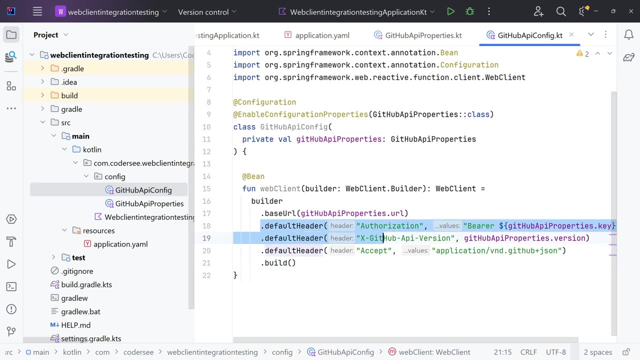 This is the custom GitHub accept header. Lastly, we need to hit build, dot build And right now the code will compile Control alt plus L to format the code Default header And basically we can see that those headers will be added to every request we'll be making. 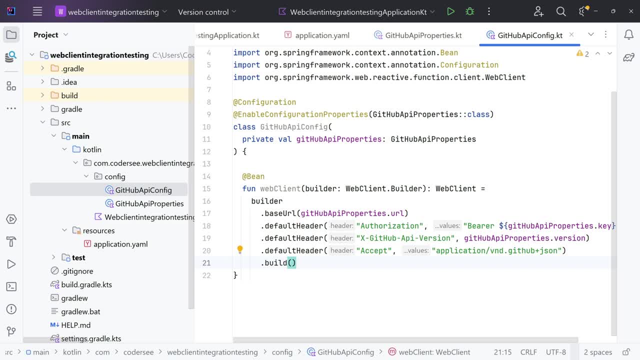 to using this web client. So, thanks to that, later we don't need to provide this every time we are using web client. Excellent. With that done, let's prepare a bunch of data classes that will need to deserialize JSON responses from the API, plus one exception class. 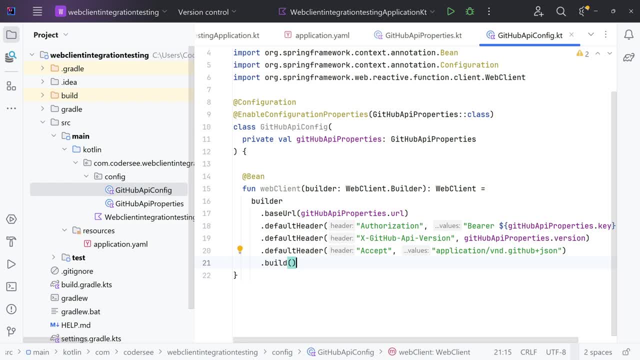 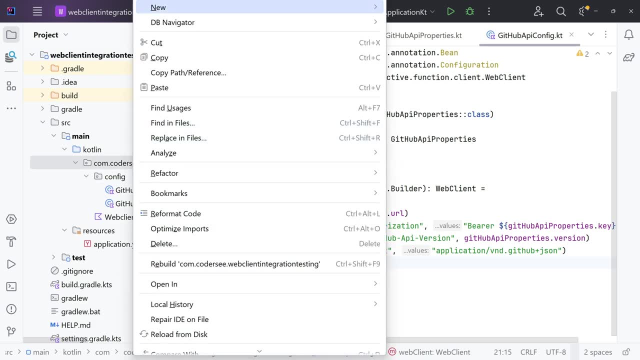 Of course, if you would like to add other fields, please check out the documentation link that I will share with you in the description for this video. So, again, as the first step, let's add a new package, new package and let's call it model. 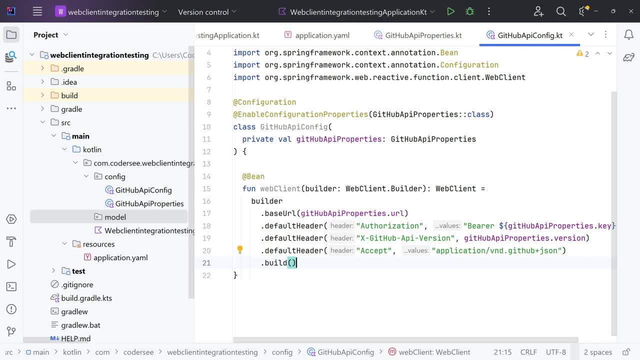 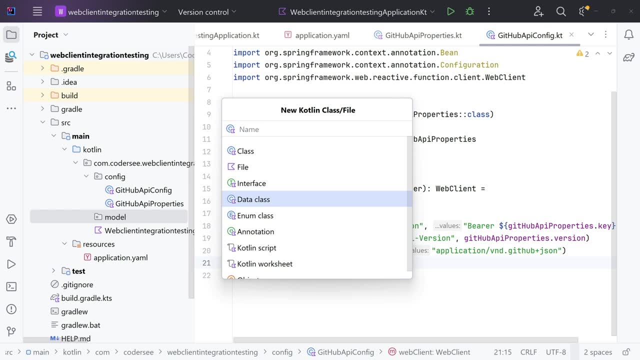 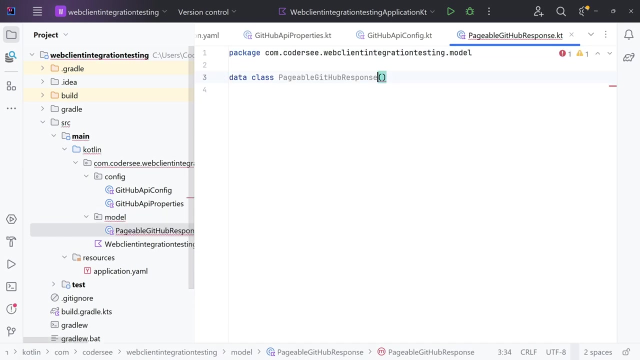 Following: let's add the pageable GitHub response: Right mouse button- new Kotlin class. And right here let's use the data class this time, so that later we don't need to convert that Pageable GitHub response. GitHub response- wonderful. 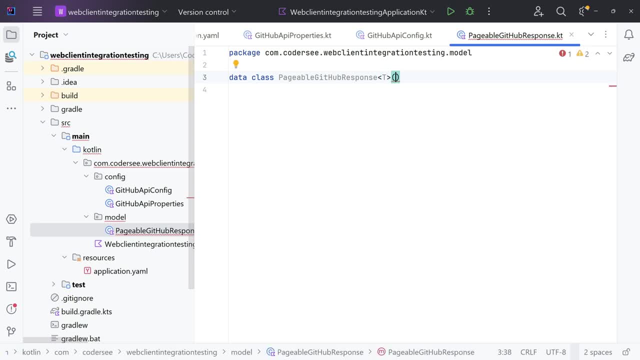 And I would like this one to take generic. So, basically, the API endpoints allow us to get only a chunk of data using the page and per page parameters, And thanks to this class we'll be able to wrap the response. So we need two fields. 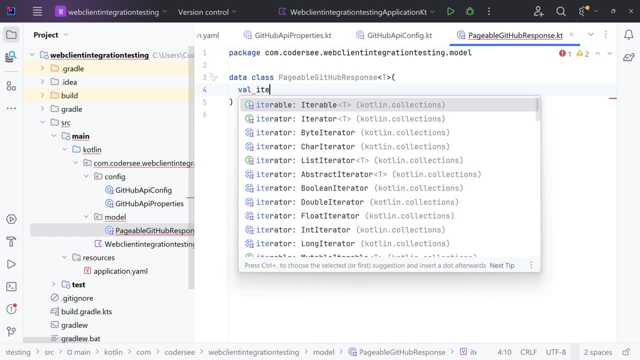 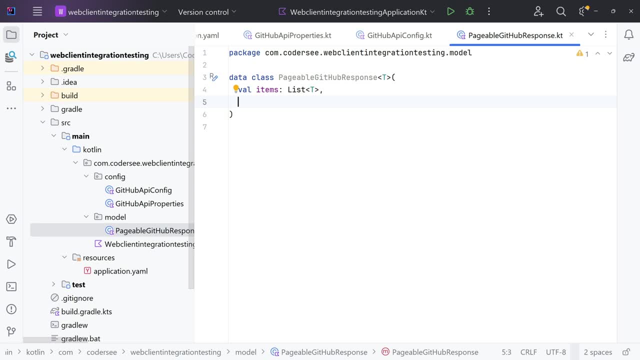 The first one items, val items, And this will be a list of the type T. The second one will be a boolean. flag has more items. that will populate with information whether there are more items or not. Val has more items and this will be a boolean. 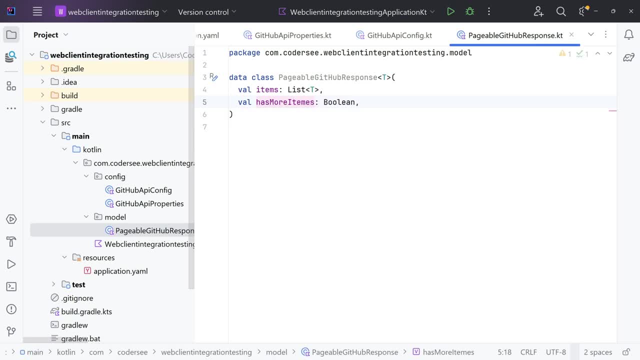 Sorry, let me items. let me fix the typo right now. Wonderful Following: let's implement the GitHub repo response Along with GitHub response, Along with GitHub owner response. So again, new Kotlin class, data class, GitHub repo response: wonderful. 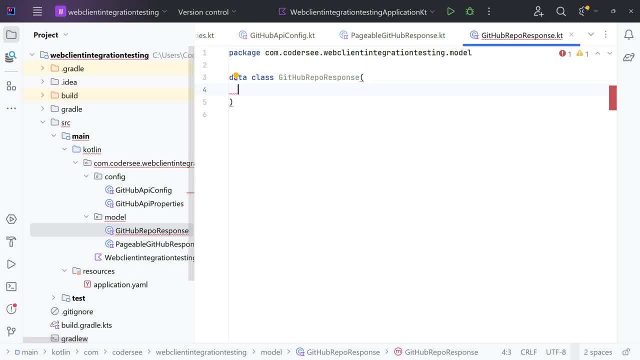 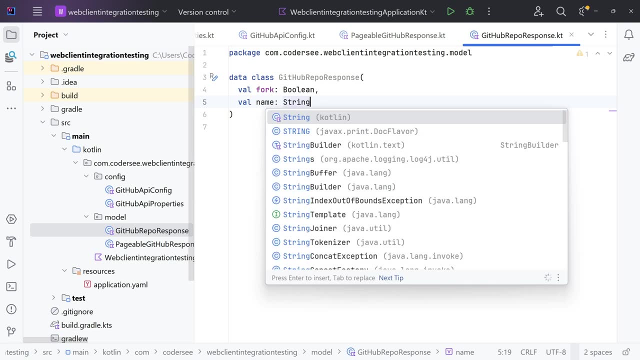 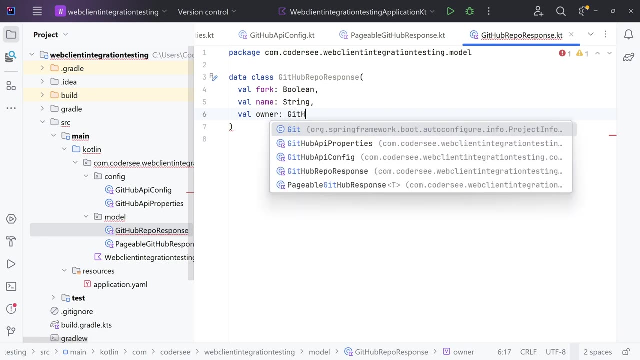 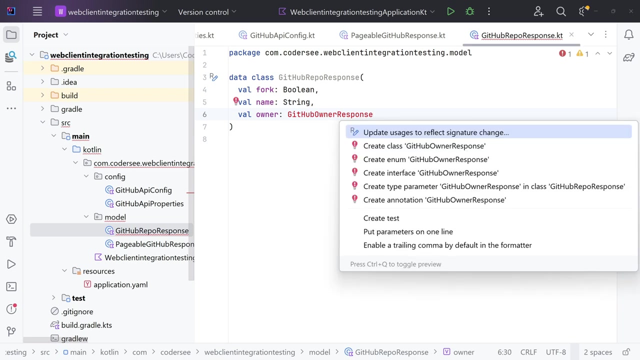 And let's add three fields: fork, name and owner val. fork will be a boolean value, name will be a string value And owner will be of type: GitHub owner response. Wonderful GitHub owner response. Of course, we need to add this class: protip, alt plus enter. 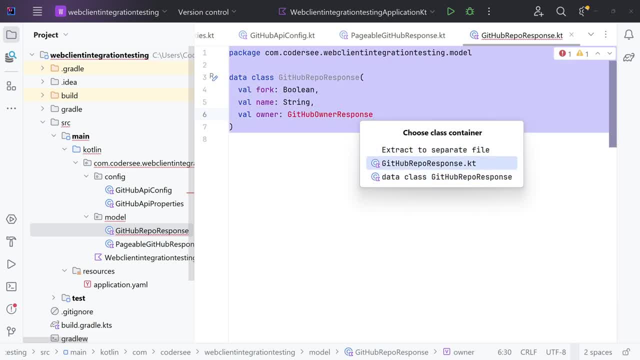 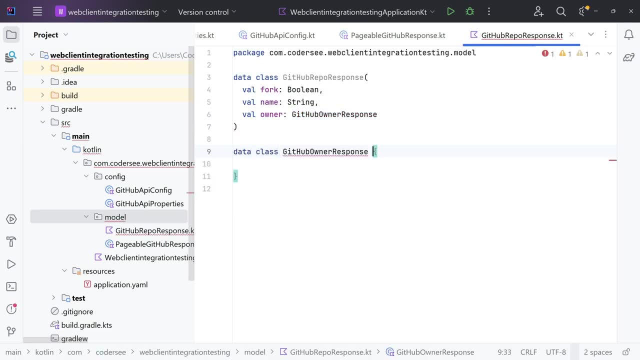 And right here we can create a class. Let's keep it in this the same file: GitHub owner response. Nevertheless, we need to convert that to data class For the owner. I would like to know the login of the particular owner. 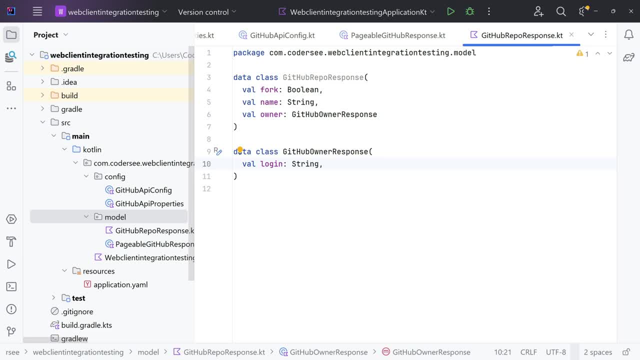 Val login. Val login- This will be a string value. Lastly, let's add the upstream API exception. This way, we'll be able to throw custom exceptions, and such an exception could be handled later, for example, with rest controller advice. And if you'd like to learn how to use risk controller advice, then I highly encourage. 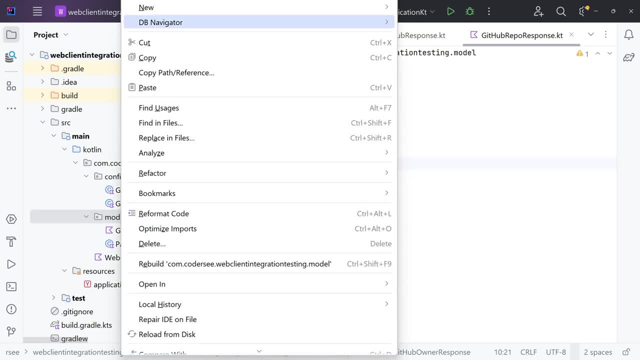 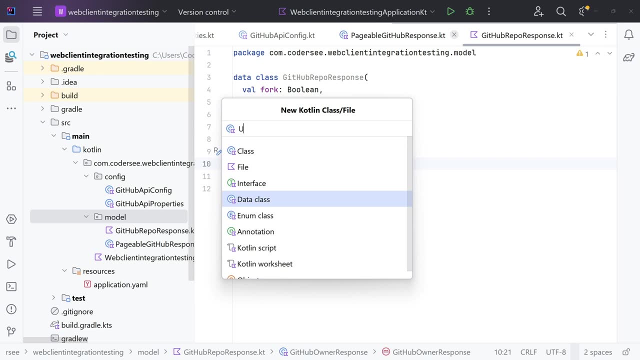 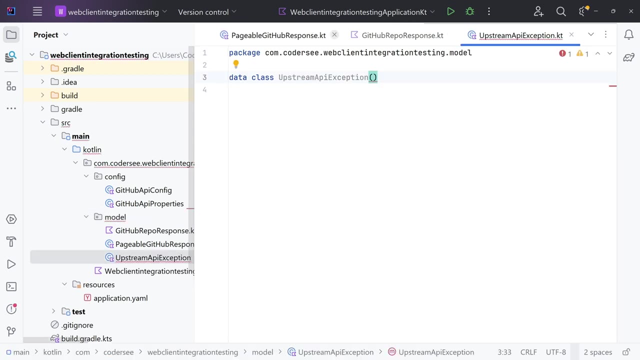 you to check out my blog Right mouse button. new Kotlin class and this data class will be called upstream API exception- upstream api exception- upstream api exception, and this will have two fields. the first will be message msg in shortcut and the second one will be status code of type http status code. so 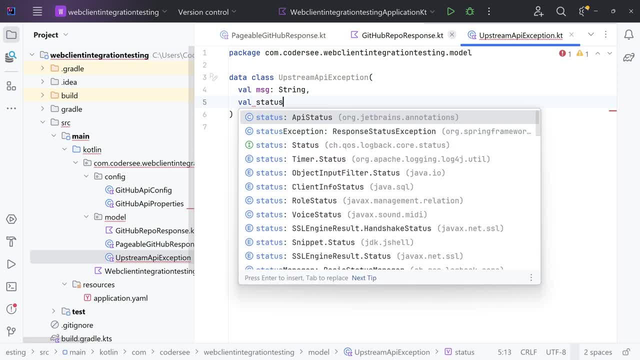 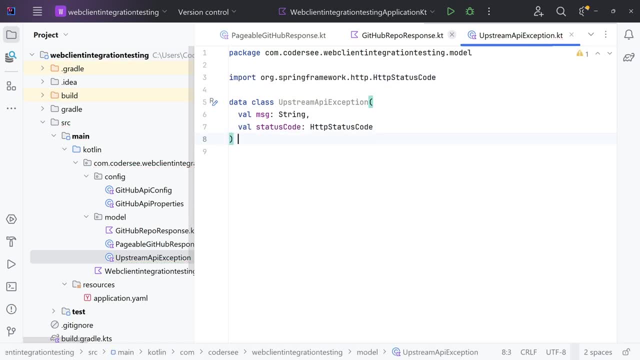 msg of string val status code- http status code- wonderful. i would like this class to extend runtime exception so that this will be exception runtime exception from kotlin and this will be msg- ctrl, alt plus l to format the code. wonderful. so finally, let's combine all of that together and let's introduce the github api class. 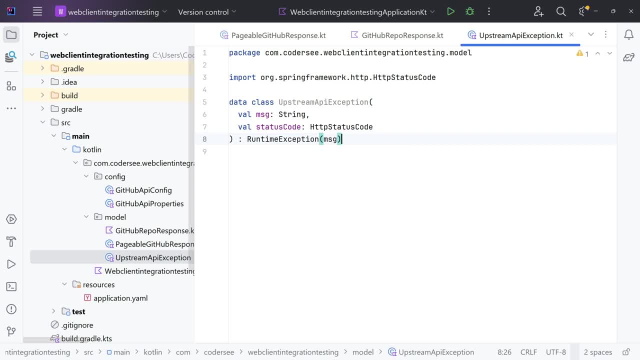 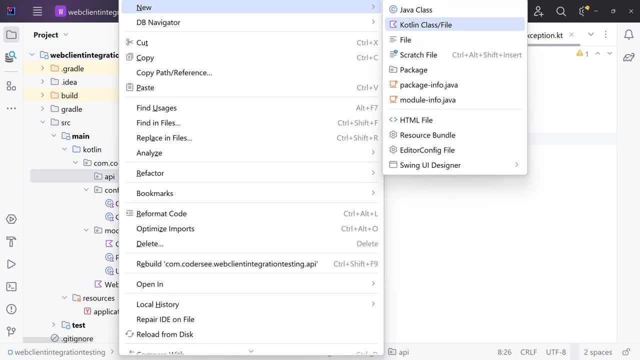 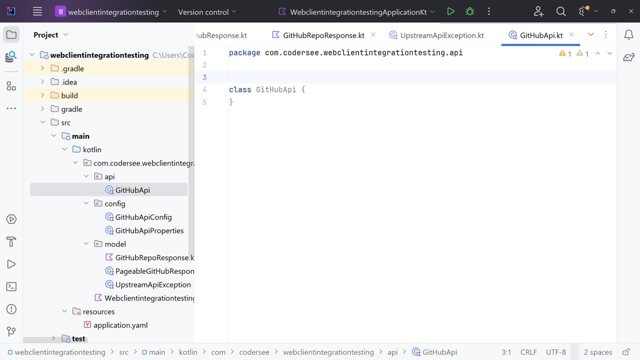 responsible for querying the api. let's click on the package, new package- and call it github api again. right mouse button- new kotlin class- github api. i would like this to be a spring component, so i'll only take that as a component with component annotation. nextly, i would like to 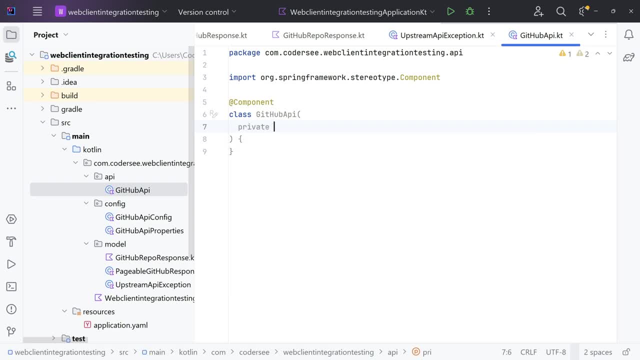 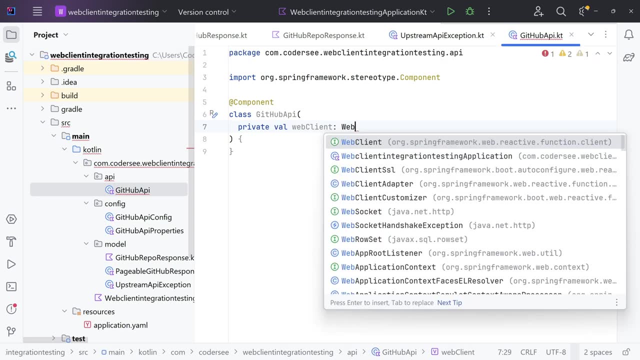 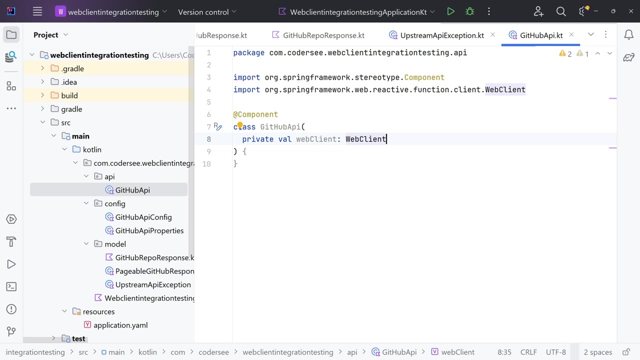 inject the web client that we will use to query the api. so private, well, web client, client of type web client. well, web client of type web client, wonderful. so in our case we have only one web client been in our project. usually in most of the production ready projects we'll have multiple ones, so we'll use, for example, 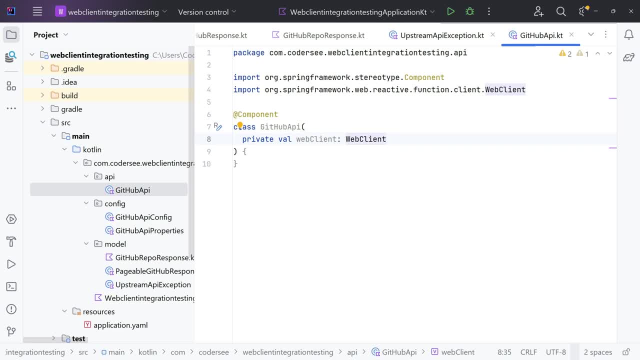 resource annotation or or or qualifier to identify which web client we would like to use, or binding by name, whatever. following: let's add a new function: list repositories by username, and this will be a suspend function because, as i mentioned, we will be using kotlin coroutines. suspend function list repositories by username. 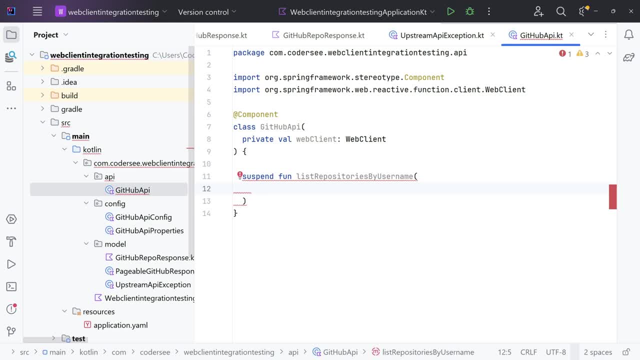 i would like this function to have three parameters: the username of string, type, page and PerPage key, so that we will be able to link not only the web machine but also these dataWORK functions to replied page and console. so, for instance, if we want to set policies to be back to normal, 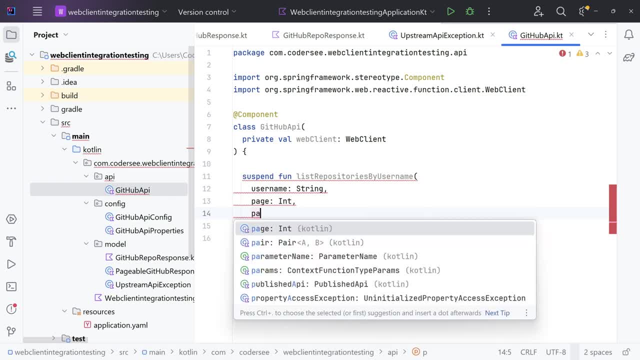 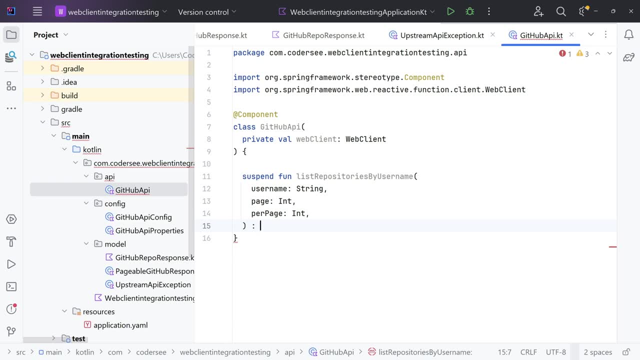 4-step1 file type field list repositories call as methodow Type: strnType, Page настrct fields. all of this by name I should keep into my memory. because I mentioned we will be using Kotlin coroutines system per page, again int type, and as a result we'll return pageable github response. pageable github. 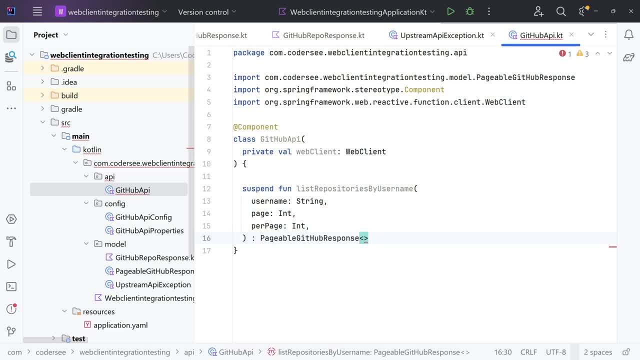 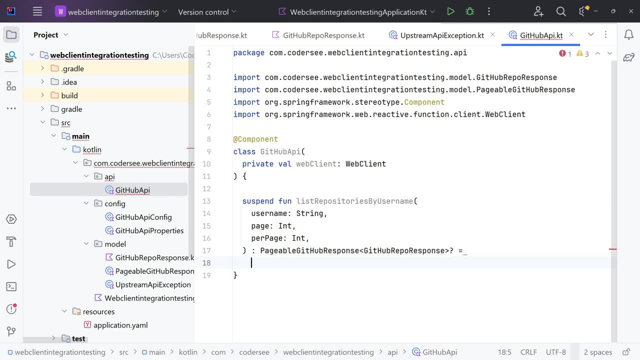 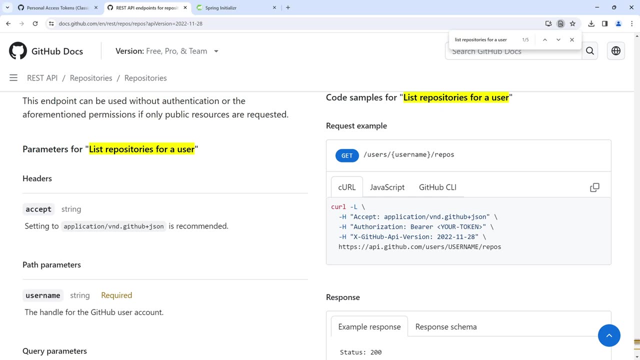 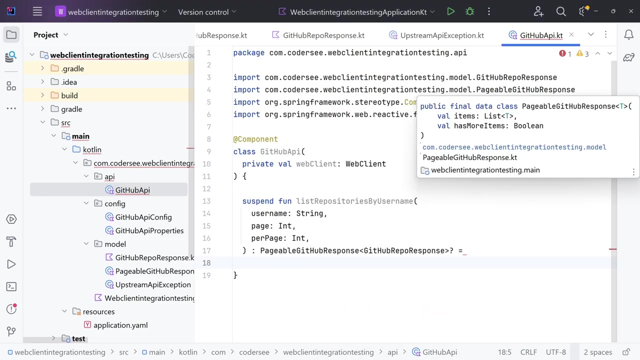 response, and this was a generic, so we'll provide github response. github response type: wonderful equals, and right now we would like to fetch the data from the endpoint. so let's get back to the documentation. this is slash users, slash usernames, slash repos. let's get back to intellij, first of all. 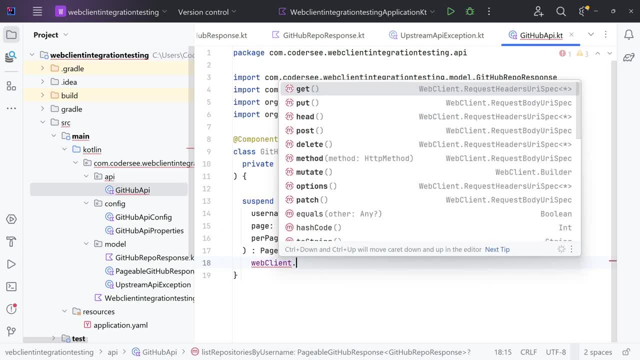 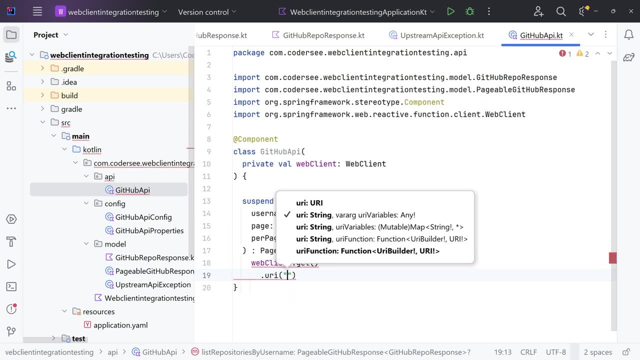 let's invoke the get method: web client dot. get method. nextly, let's provide the uri and i would like to provide that as a string value. slash, users slash. we need to provide the username. so again, string interpolation, slash, repos. so at this point we would use the default page and per page values and i would like to make: 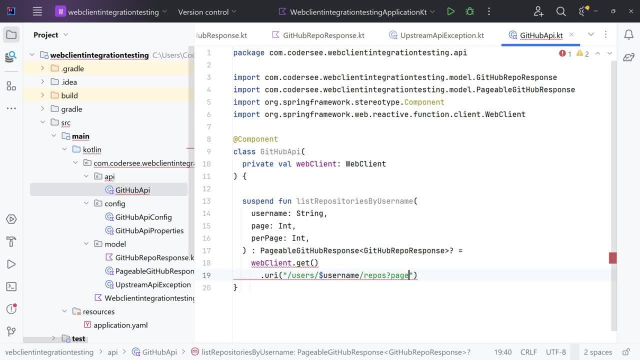 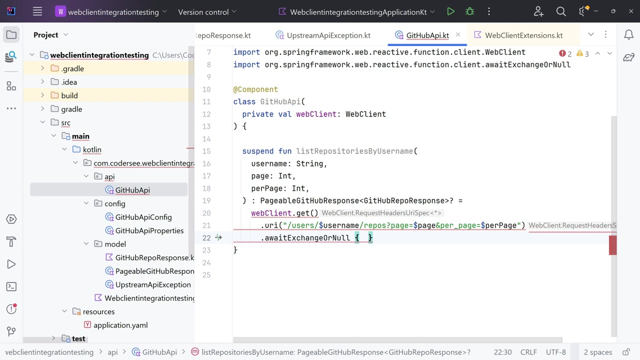 that specific. so, first, query parameter: page equals, and let's specify the page. and to provide another query parameter per dash- sorry underscore- page equals and let's provide the value: perfect. lastly, dot await exchange or null. and i would like to introduce a new function: map to pageable response and, as an argument, provides to: 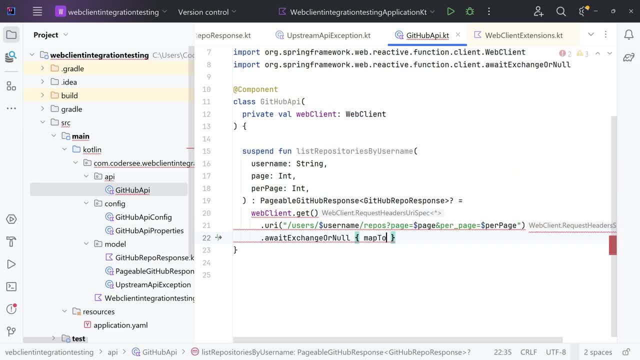 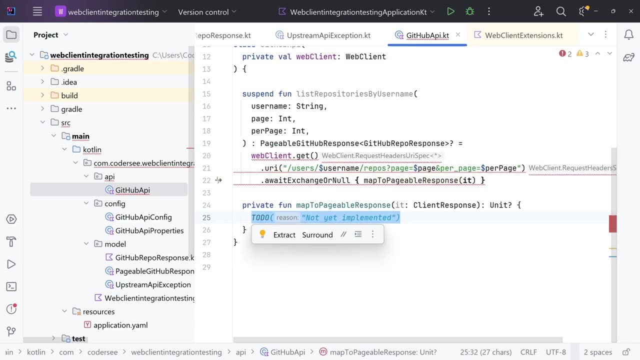 it the client response. so map to pageable response and let's forward it. alt plus enter to introduce the function and let's create a function. we'll implement this in a moment, but in the meantime let's summarize: we make this function a suspend function and we're going to create a new function. 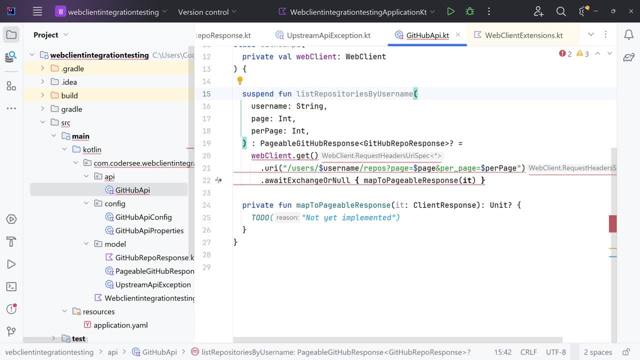 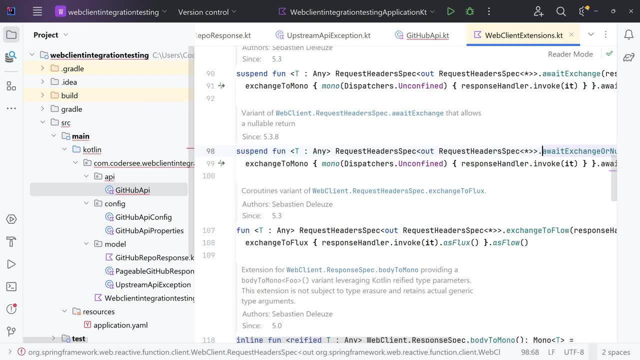 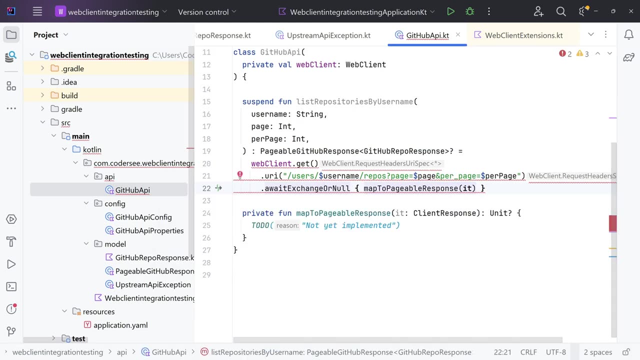 because await exchange or null is a suspend function too. i can hit control, keep it pressed and click left mouse button on the function to see that right here, this is a suspend function too. if you would like to learn more about that, i have a separate video in which i am explaining. 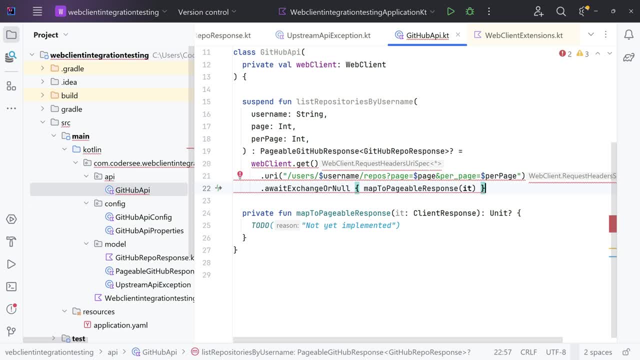 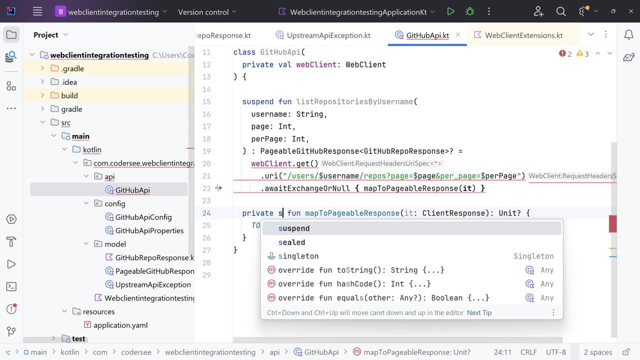 how to use web client with coroutines. nevertheless, let's add the missing code. so i would like this function to first of all be suspended, to be blamed in order to access the type t, so private softspend inline font, and i would like this to reify. 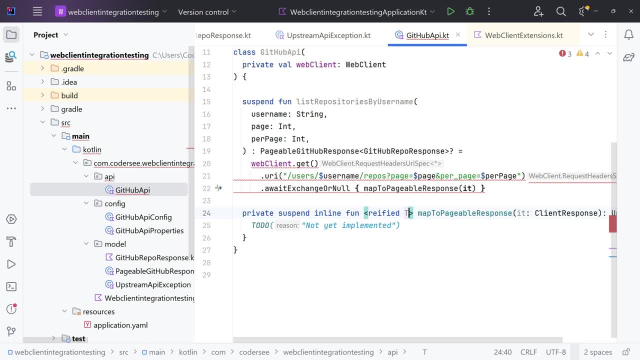 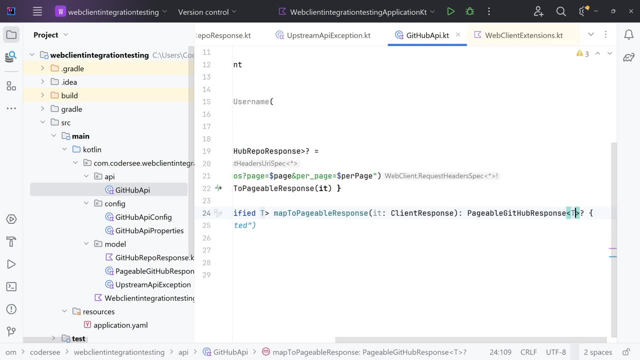 as a response, i would like to return the pageable github response of type t. pageable github response of type t. and this will be nullable. wonderful, right now you can see that the current language is called a, Perché. that is wiresiod ako okay. next, but not least, we will import all the commands to inspire our model. i would like to create demands on 그대로 the program and running it. as a result, we have removed the code from licens ethernet. That's pretty easy because etc is just a Nova basic for us here and of course, you can download it. 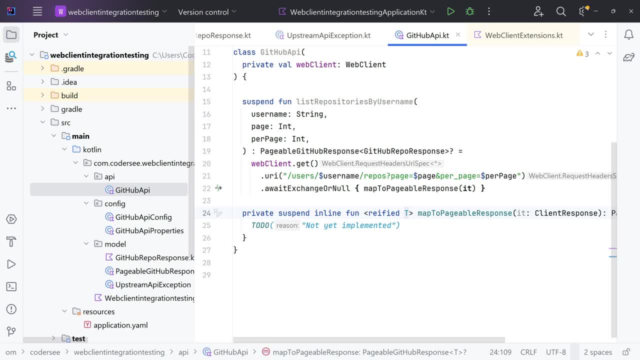 call this compiling, so not that bad. Next, let's rename the parameter here, the argument, client response. wonderful, And as the first step I would like to check if there are more pages to fetch, How we can do that. So let's get back to the documentation. 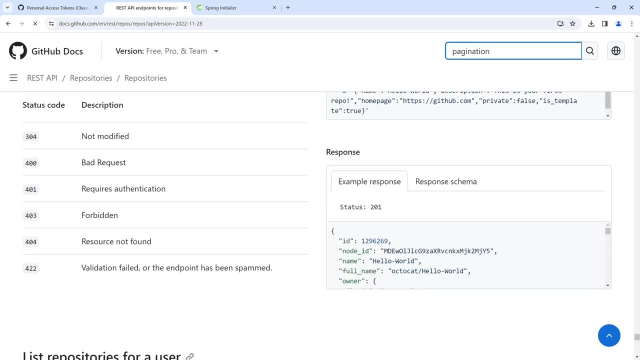 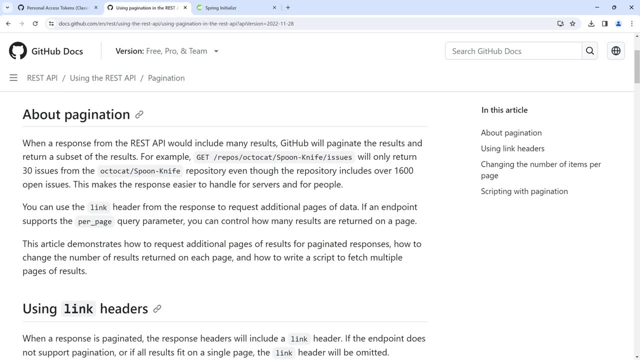 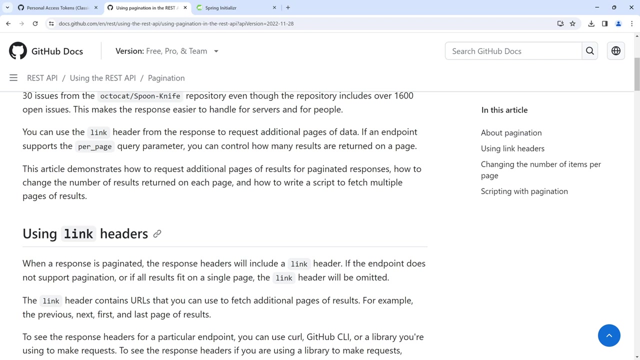 Actually, let's search for pagination. hit enter and there is this article using pagination in the REST API. I highly encourage you to check out it. but long story short, GitHub API returns the link header And if its value contains the rel="next". 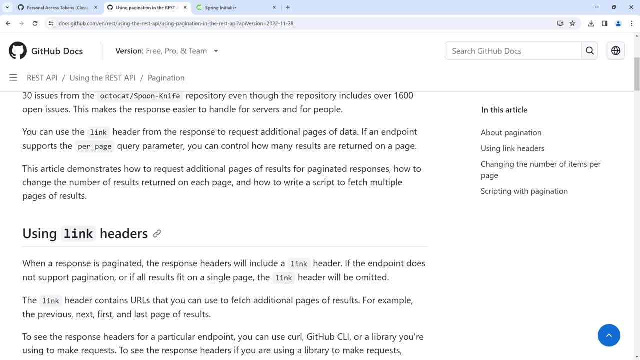 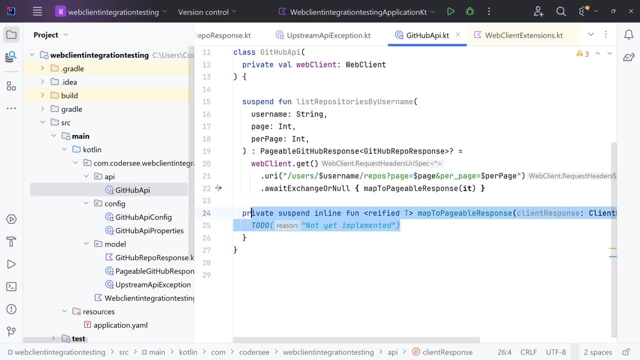 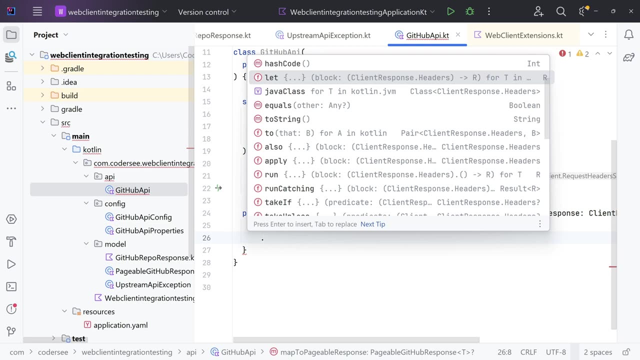 it means that there are more pages to fetch and we'll use this property in our code base. So let me get back to IntelliJ and we'll see that in action. So, as I mentioned, first thing, client-responseheaders- In order to read the headers. 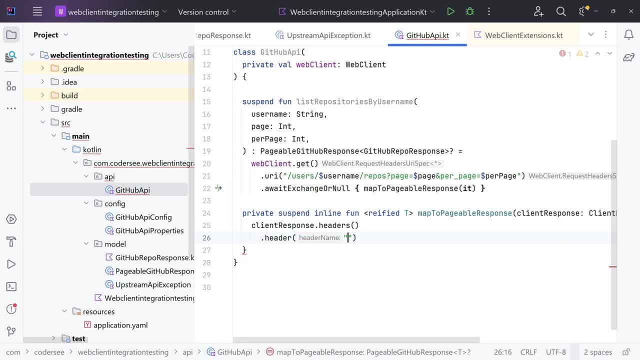 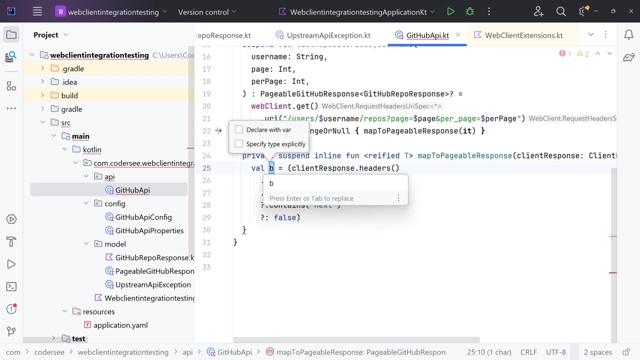 let's search for the link: header, Link nextly first, or null contains next as a false. Alt plus enter, introduce local variable and I will call it hasMorePagesToFetch. HasMorePagesToFetch. Moreover, we can enclose that. 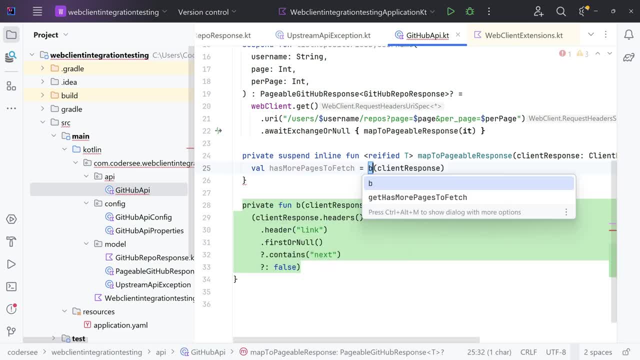 control plus, alt plus m and extract that to a separate function. Check if more pages to fetch- wonderful, We can click on that alt plus enter. specify the return type explicitly. I know that this is optional, but that's how I usually proceed. 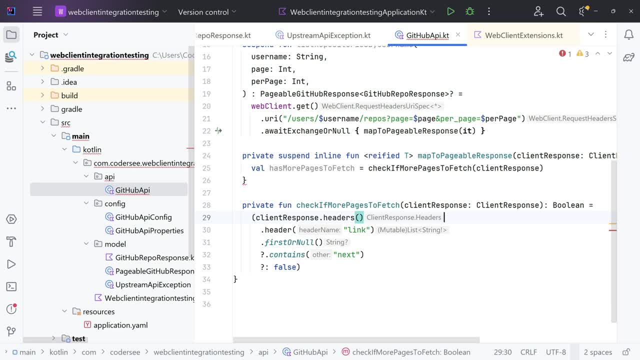 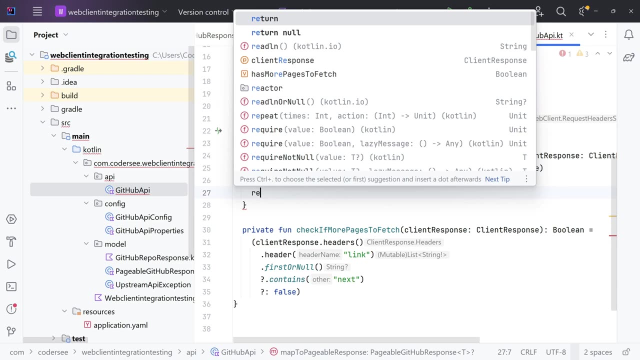 Okay, so hasMorePagesToFetch. as you might have guessed, we'll use that in our pageable GitHub response to indicate that there are more items. Nextly, let's process the response. So I would like to return, And right now let's add when val status code. 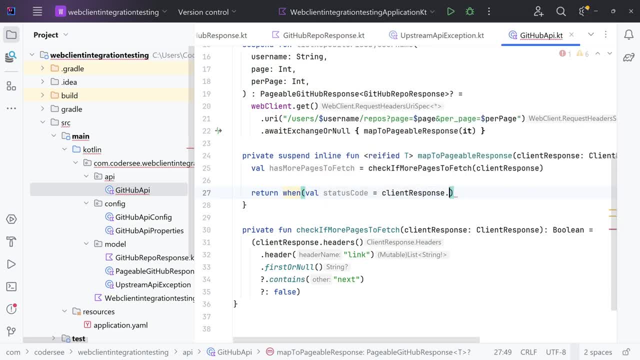 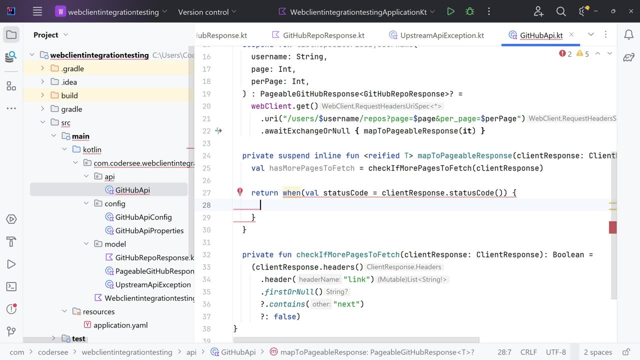 Let's read the status code: client-responsestatusCode. Let's open up the brackets. So, if this is okay, I would like to deserialize the JSON payload to the body, to the list. So in our case, we would like to do that to GitHub repo-response. 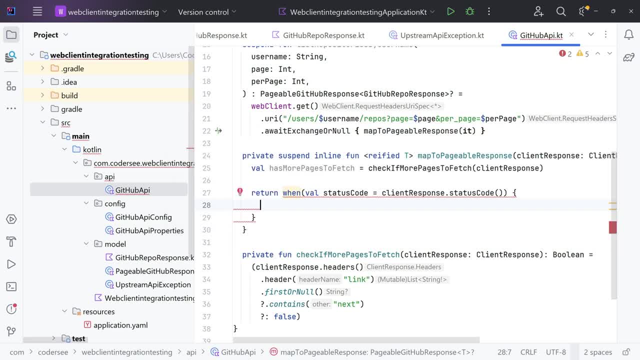 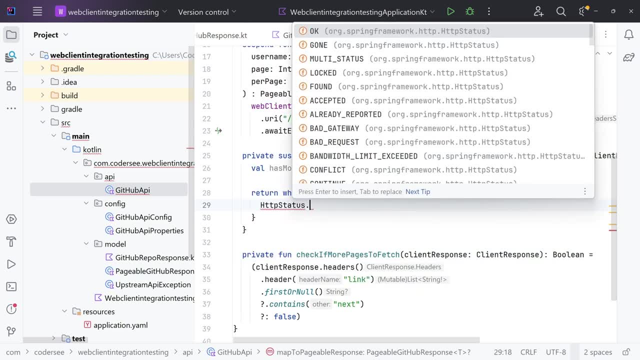 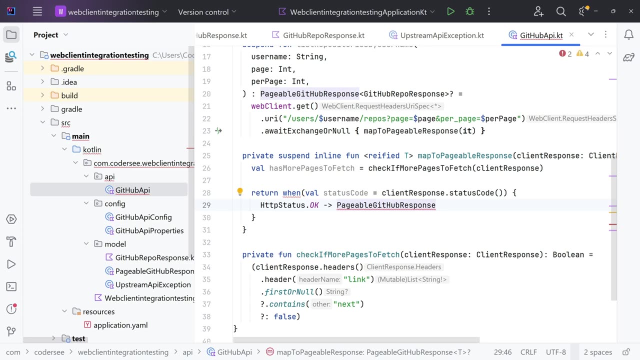 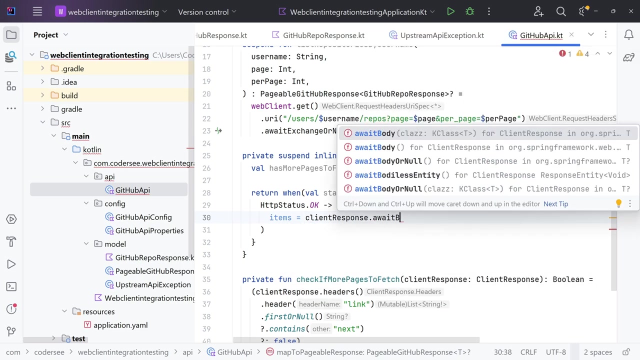 Anyway, let's keep this function as generic, As generic as possible, So httpstatus dot. okay, If that's the case, let's return pageable GitHub-response with items equals client-responseawait-body, And we need to provide the type list of type T. 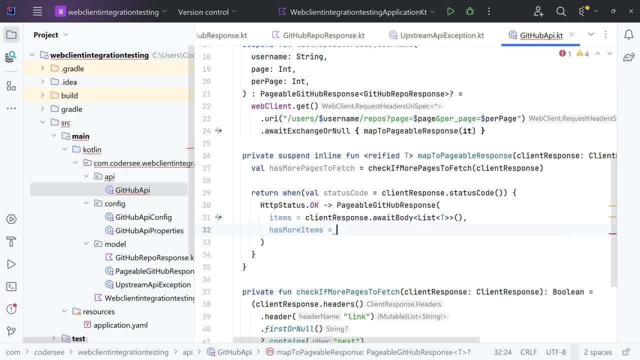 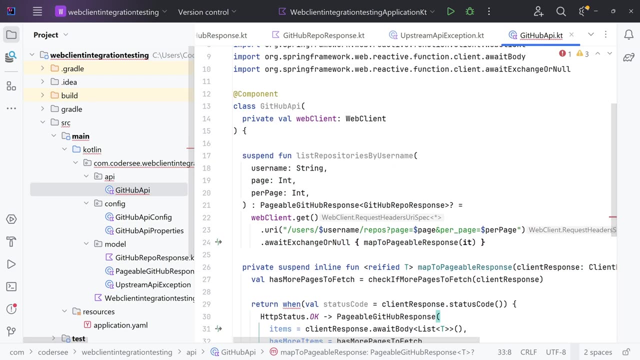 Wonderful HasMoreItems, Let's hasMorePages to fetch. One of other status codes that we can get will be 404, not found, And in this case I would like to convert that to simply null, because we are returning a nullable type from our function. 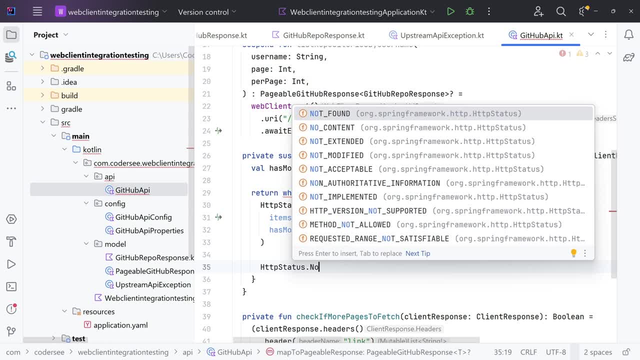 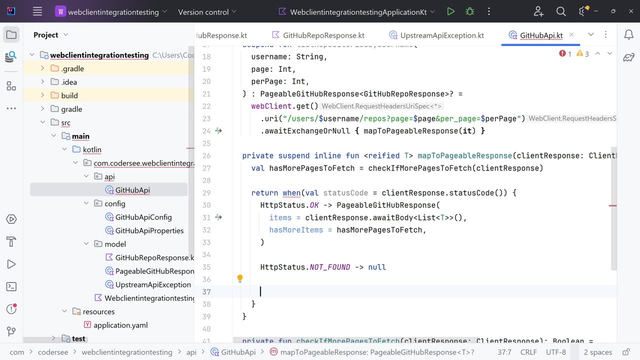 So httpstatusnotFound, And if this is the case, I would like to return null And otherwise, if we are getting any other code, any 500, or something like that, let's go with else. Throw Upstream API exception. 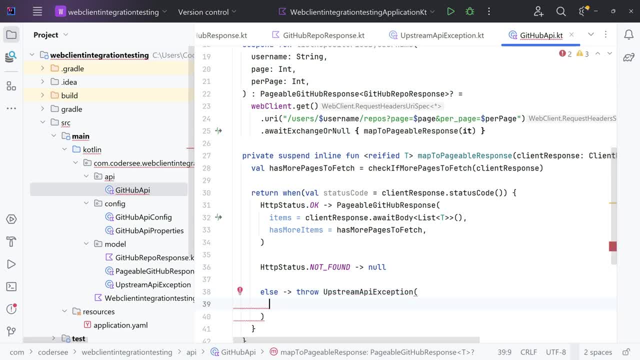 And as a message, I will provide github-apirequest-failed- M-s-g. github-apirequest-failed- That's on the dot colon, and let's provide the status code as the status code. Excellent easter egg. I would like to show you how we can use the reference instead. so this is a synthetic. 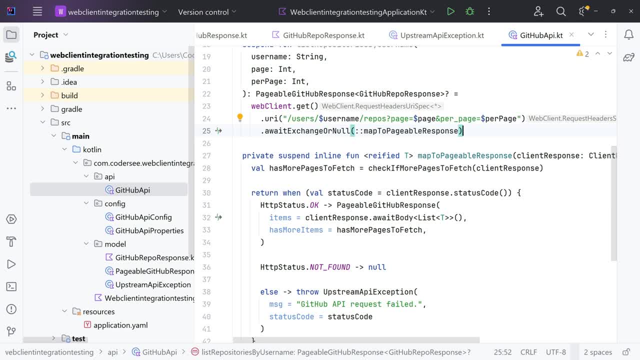 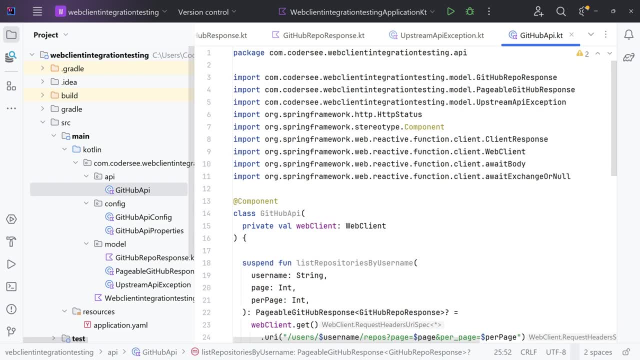 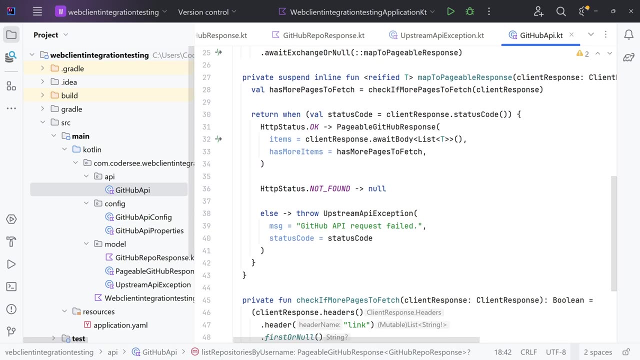 sugar that we can use right here. at this point, we have almost everything we need to test our web client implementation with wiremock. right now we have the github api and the function that will be responsible for calling the github endpoint, so I would like to show you only a few example. 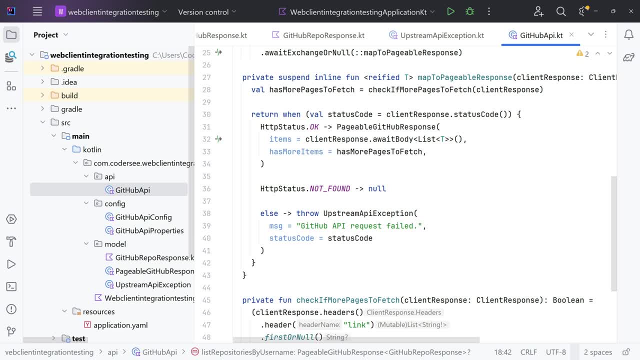 test cases that you will be able to easily adapt according to your needs. so we'll implement 200 ok response with an empty list, 200 ok with items and more pages. and 200 ok with items and no more pages to fetch. apart from that, 404 not found and 401 unauthorized. when you will be implementing? 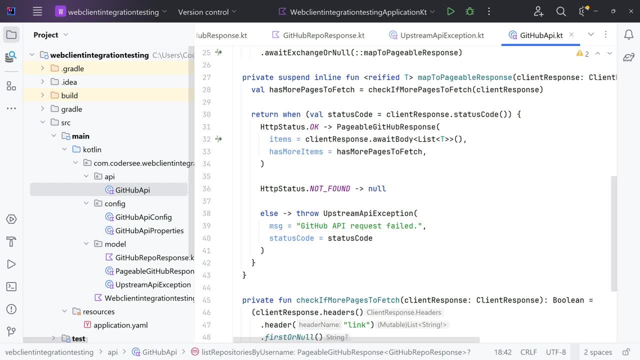 your own integration test. this is the moment when you should do the homework and analyze the api you are working with. so what are the possible happy paths? How should your code behave in case of any error status code? what if we add some latency and many, many more cases that you can figure out? 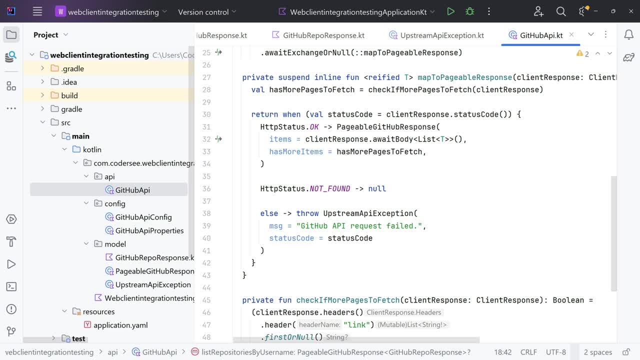 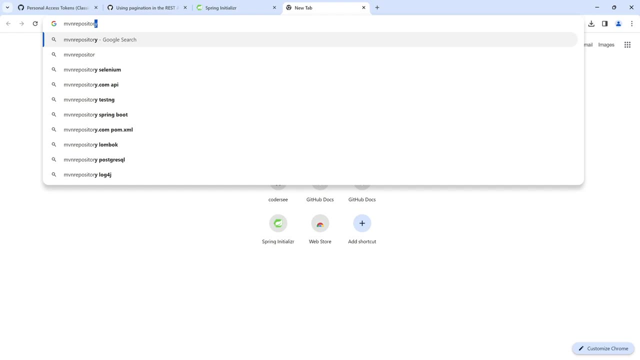 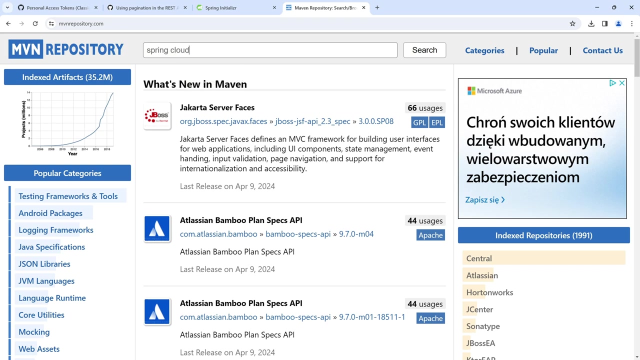 As the next step, we need to add the necessary dependencies. We'll need WireMock and Kotlinx coroutines for tests. So let's open up our browser once again and let's navigate to maven repository And let's search for contract wiremock- Spring cloud contract wiremock. 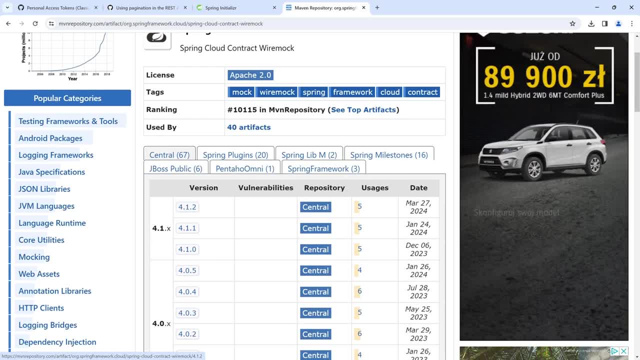 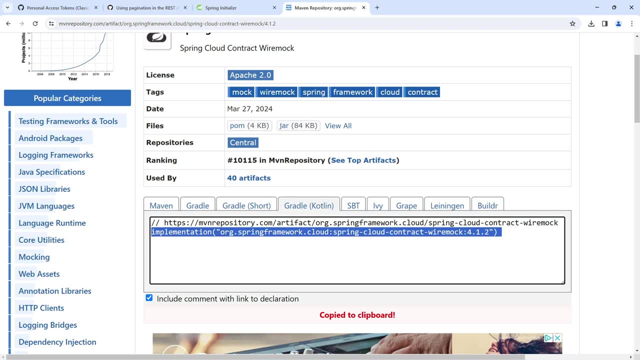 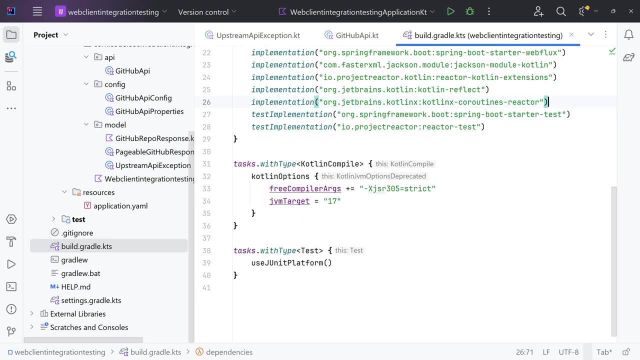 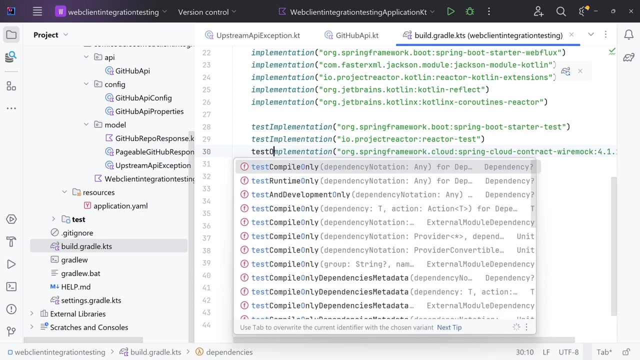 Let's hit enter. This is that one that we're looking for. I'll use 3.1.2.. Let's specify the Gradle Kotlin Control plus C And let's get back to IntelliJ Build Gradle, And I'll add this right here as the test implementation: Test implementation. 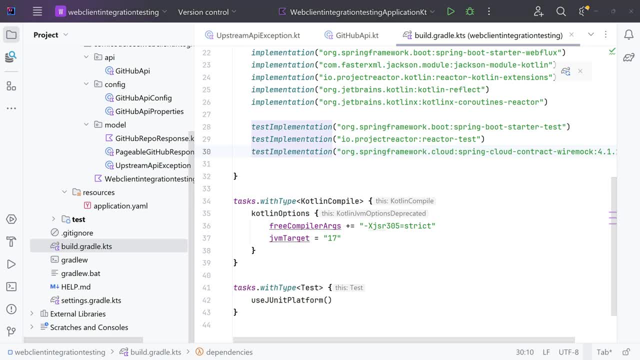 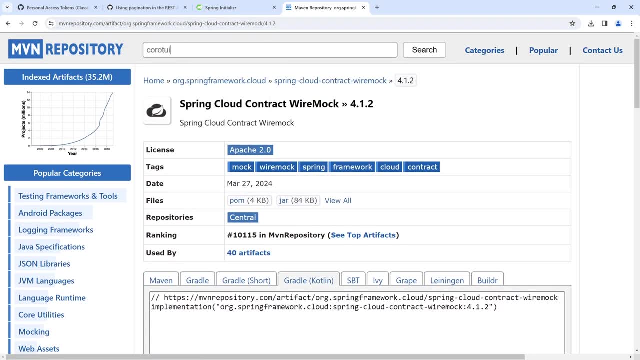 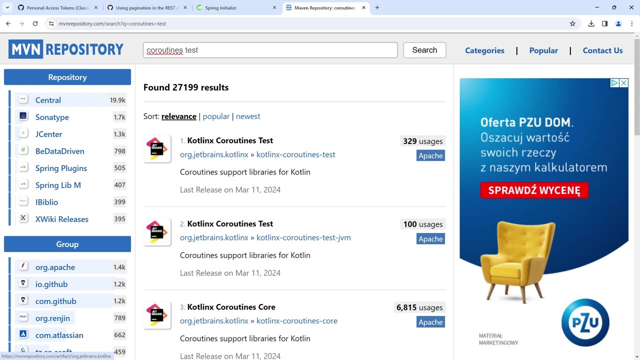 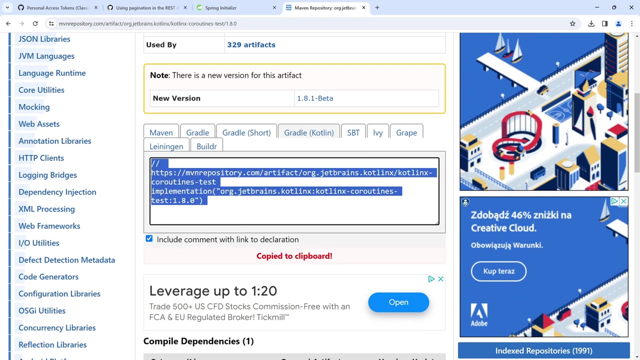 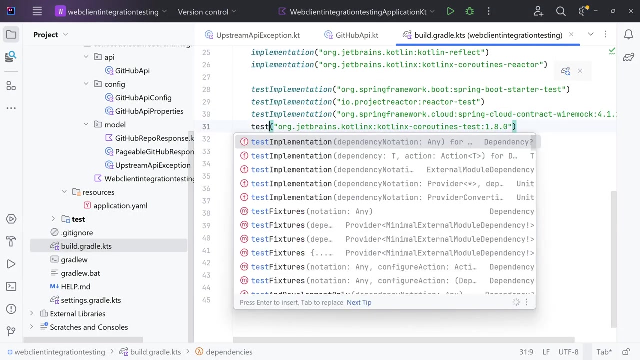 tool Wonderful. Let's get back to the maven repository and let's search for Kotlinx, coroutines, test Coroutines, Coroutines, Test This one Or the JetBrainsKotlinx, And let's use the 1.8.0. Control plus C, IntelliJ. again, We'll need that for test implementation. 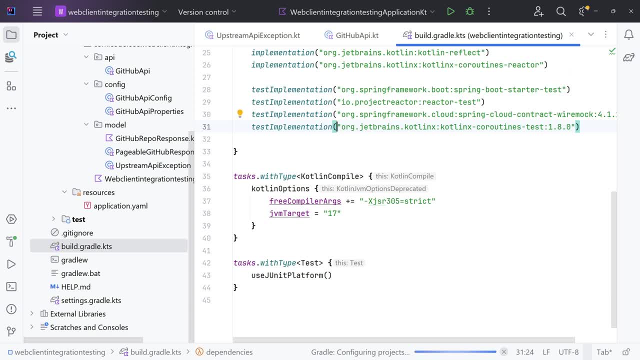 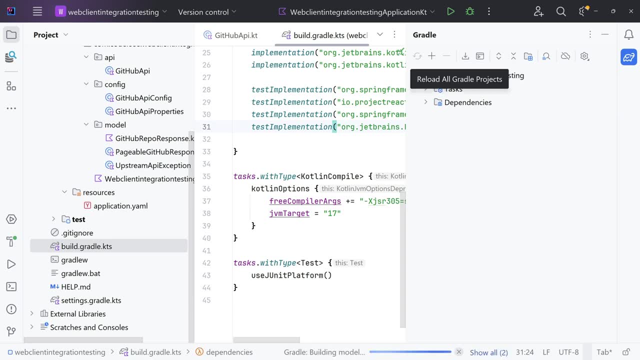 Following. let's hit this icon right here to sync the project. If this does not pop up in your case, you can click always on Gradle And use this icon to reload all Gradle projects. So when all of the necessary dependencies are added, you can see that the project is. 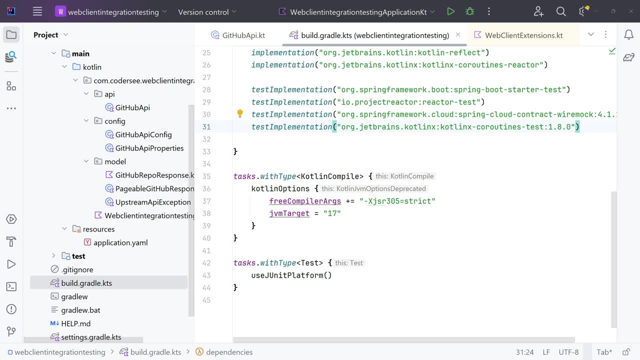 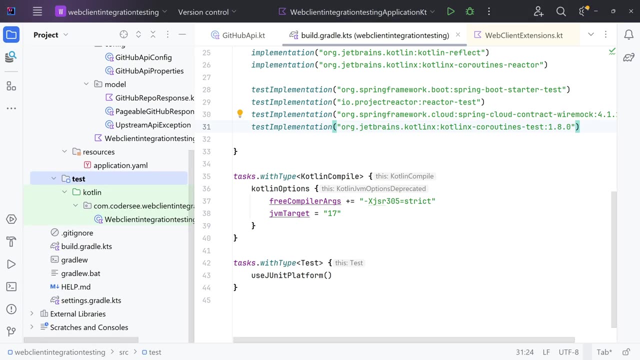 fetched, We can add the expected JSON files. So personally, whenever working with WireMock, I am a big fan of externalizing the expected JSON files. So simply we put them inside the test resources- Test. We don't have something like that, So we can click new Directory. 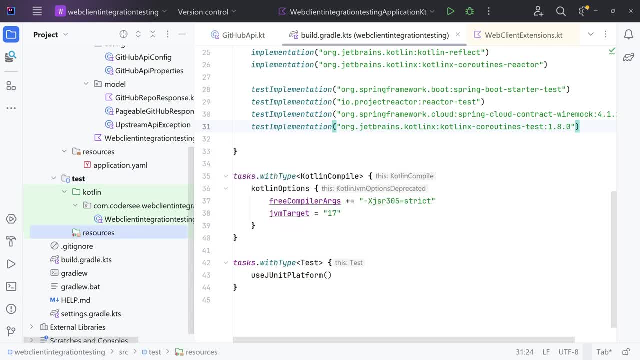 And we can see right here that this is already provided. Let's hit enter And we can see that we have the test resources. How can we fetch them? Well, in this case I will use the ones that I have already in my GitHub repository. However, in a real life scenario, I encourage you to simply query. 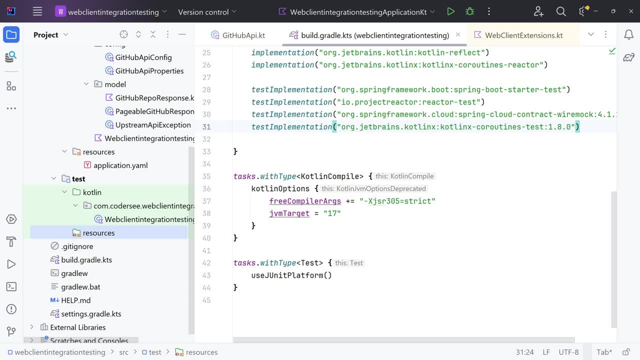 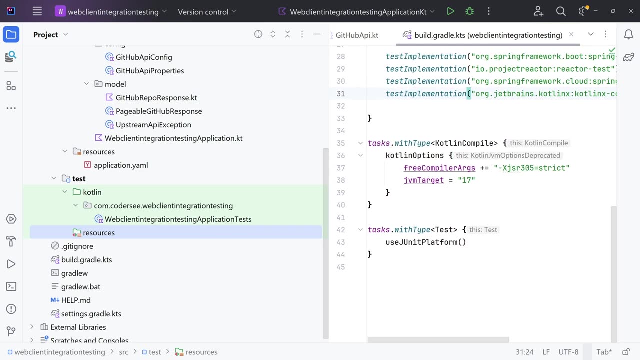 the API and see what are the difference cases that you can encounter, Because this will be the closest to a real life scenario And we would like to go for that. Nevertheless, before fetching them, let's add new packages in the resources, A new directory. 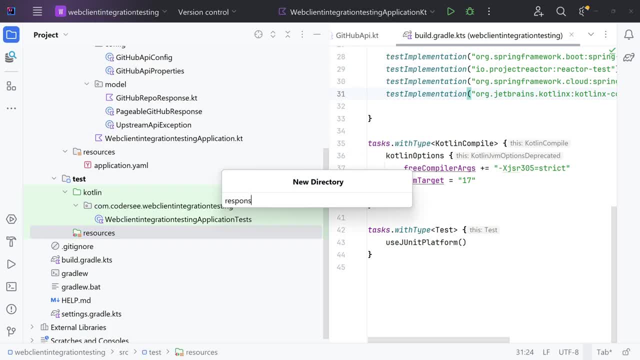 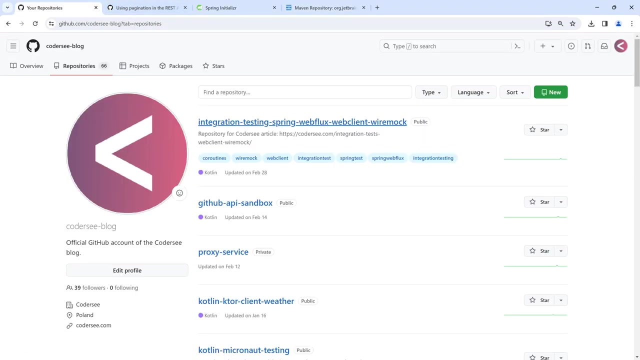 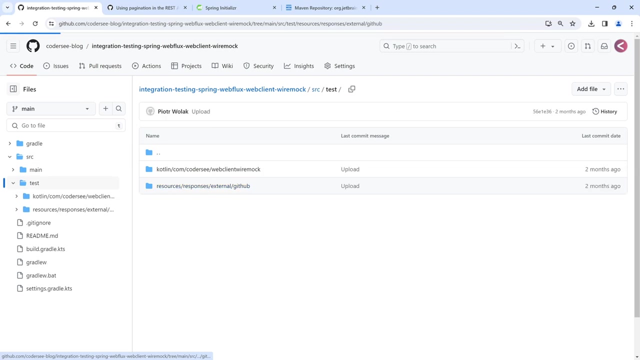 New directory, Let's call it responses. New directory, Again external. And lastly, GitHub. New directory, GitHub, Wonderful Following. Let me navigate to my GitHub page. Let me find the integration testing SRC. Let's see Tests, Resources, Again, we can see Resources, responses, external slash GitHub. 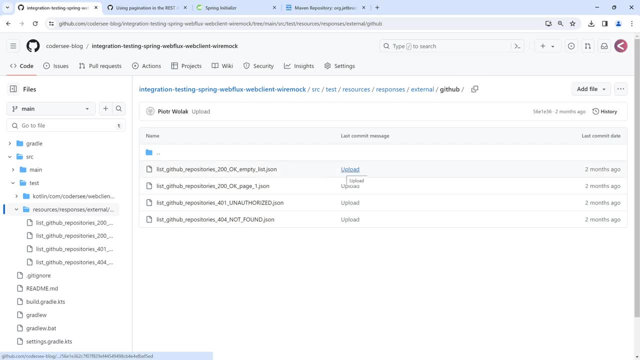 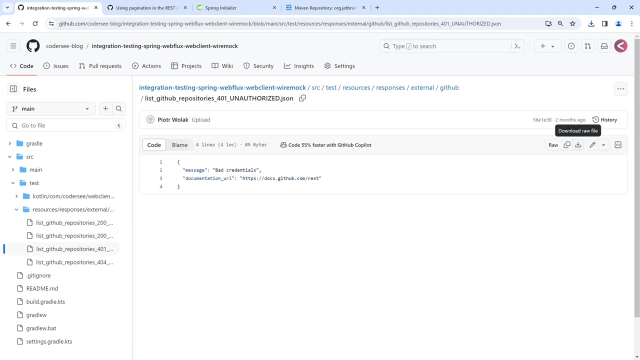 I will provide a link for this repository in the description for this video. So don't worry, Let's go for the first one. Right here we can download raw file. We have first one pager. Again, Download the file. Let's do exactly the same for. 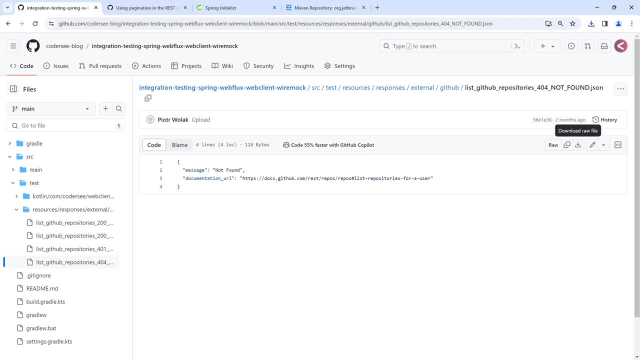 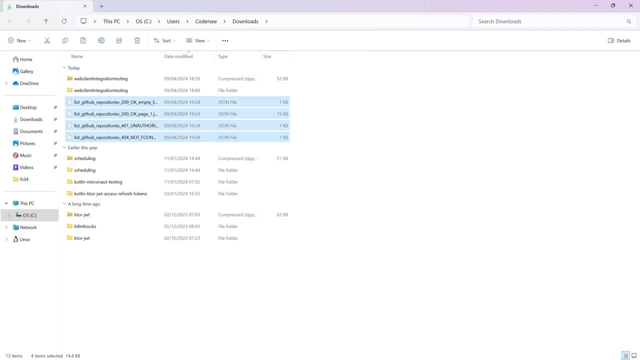 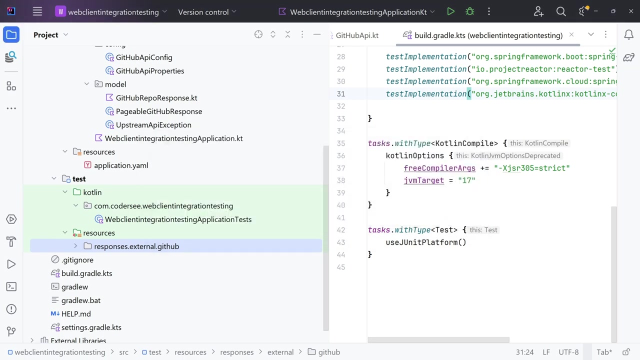 two remaining files. wonderful. Now let's navigate to the directory where they were fetched. Ctrl plus X to cut that. let's navigate to IntelliJ and Ctrl plus V right here. Let's hit OK and we can see that all of these files have been added. 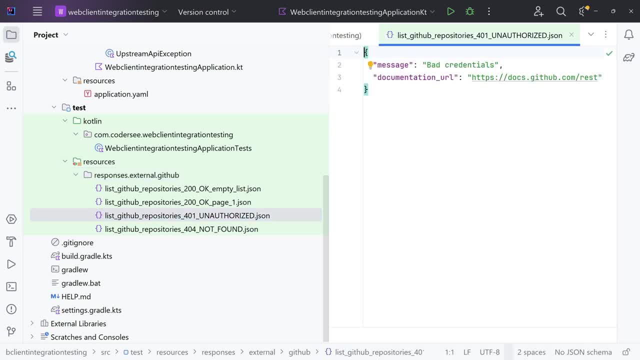 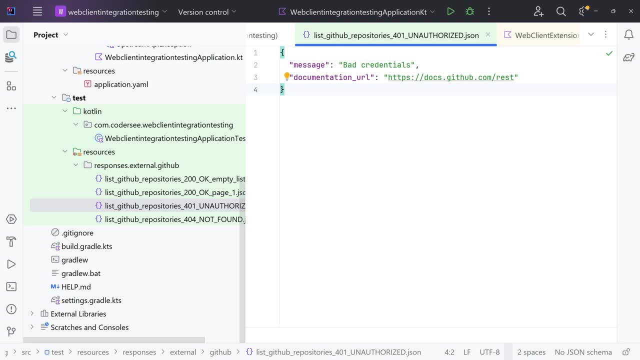 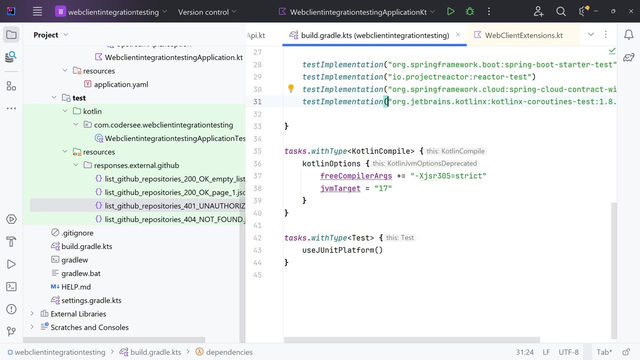 Let's take a look, for example, at 401- Unauthorized. we can see right here we have message blah blah blah about credentials and the documentation URL- wonderful. Before we start implementing test cases, I would like to prepare a util function that we'll use to read JSON files inside the test resources as string values to our test cases. 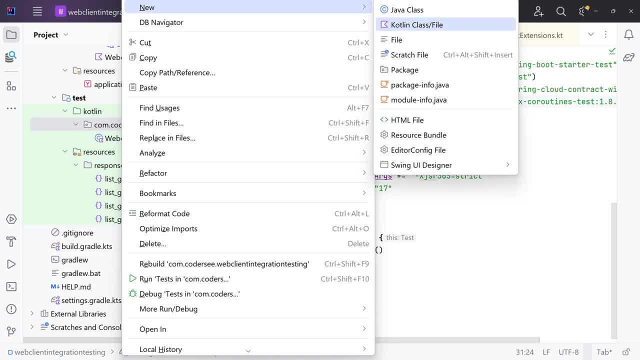 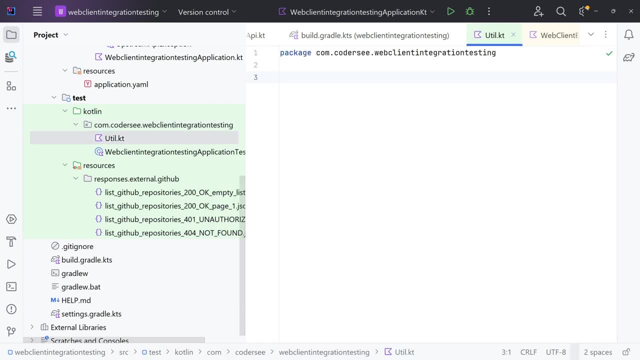 So let me click right here. new Kotlin class. This time I would like to go with Kotlin file and call it simply util. This will be test util. Let's add a new function called getResponseBodyAsString- fun getResponseBodyAsString- and I would like. 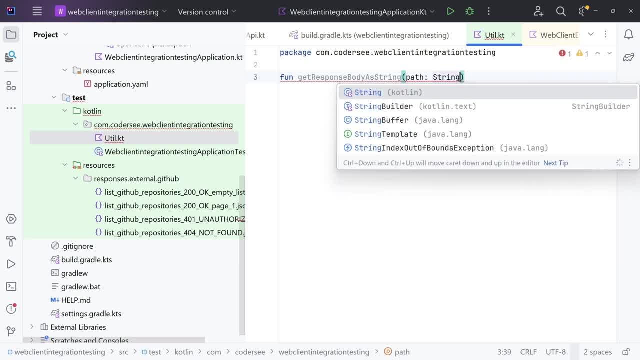 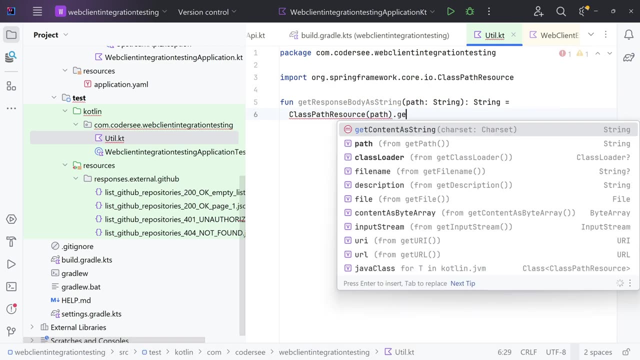 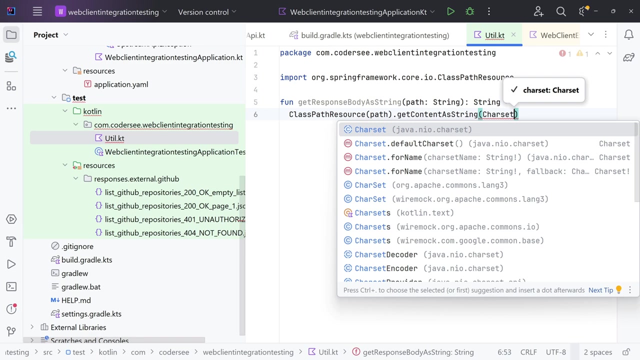 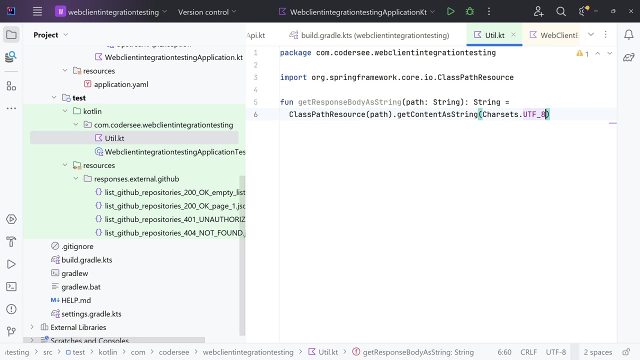 this function to take one parameter path of string type, and this will be referring a string value with our decoded JSON. Next three: let's use class, path, path, resource, pathgetContentAsString, and I would like to provide charsetutf8, excellent Ctrl-Alt-L. 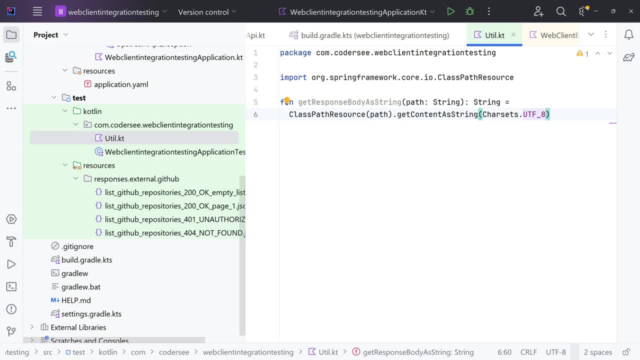 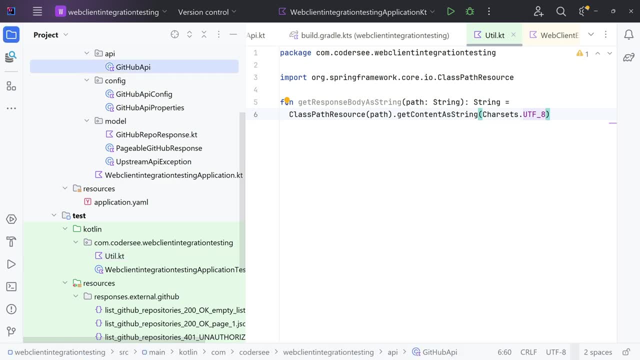 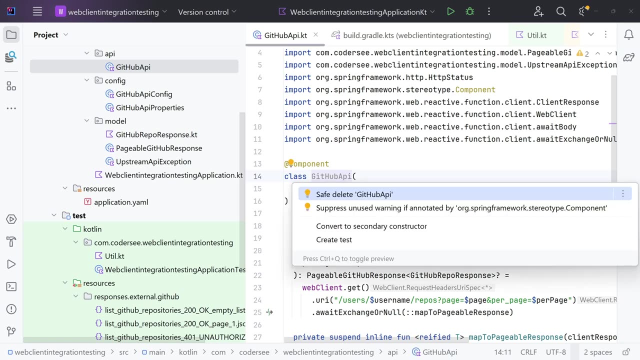 With all of that done, let's start implementing the GitHub API test class. So you can do that manually, or alternatively, you can go to GitHub API. Click on the class name: Alt-Plus-Enter. This is the shortcut that allows you to do a lot of things in IntelliJ IDEA. 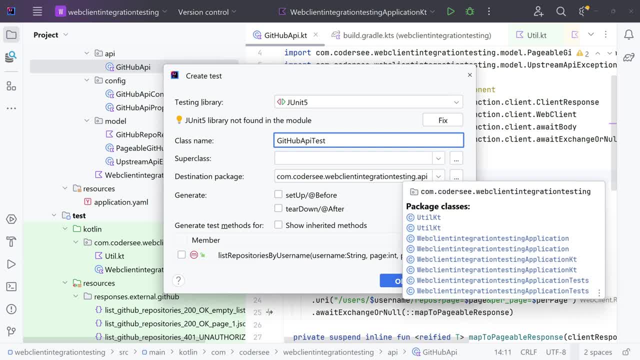 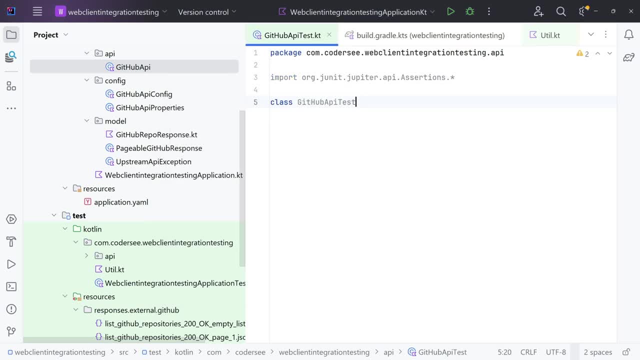 And hit create test. right here, The pop-up window will allow you to specify the class name and things like that. Let's call it the GitHub API test as the default one. The first thing I would like to do would be to introduce three constants: the test key. 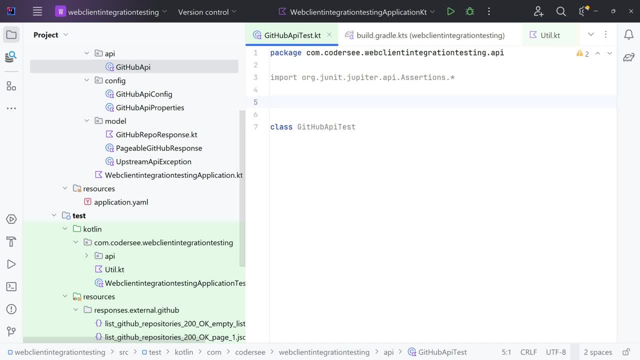 test port and test version And that we'll use in our case. private const val. test key equals test key Ctrl-Plus-D to duplicate and the next value will be test port 8082, Ctrl-Plus-D- test version test. 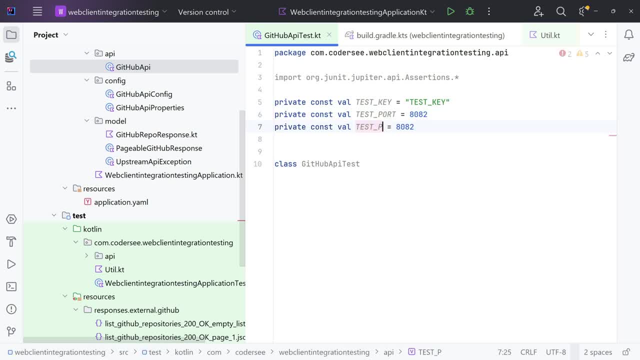 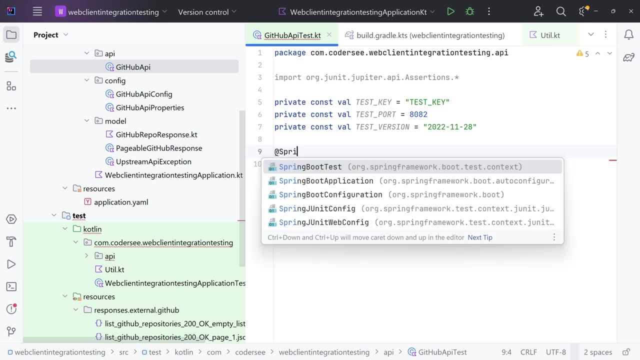 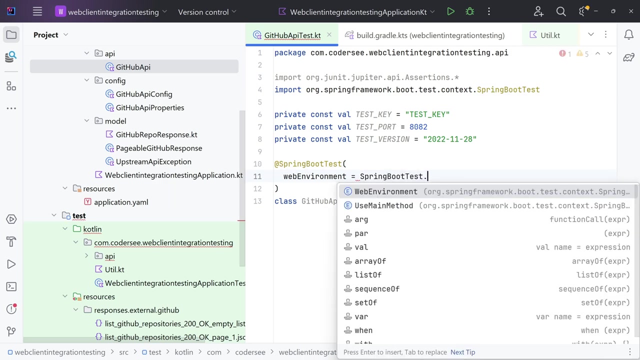 port, And that's it: 20,, 20,, 2, 11,, 20,, 11.. Wonderful. As the next step, let's add the Spring Boot test annotation: Spring Boot test annotation. And let's specify the web environment: Spring Boot test dot. web environment, dot. random port. 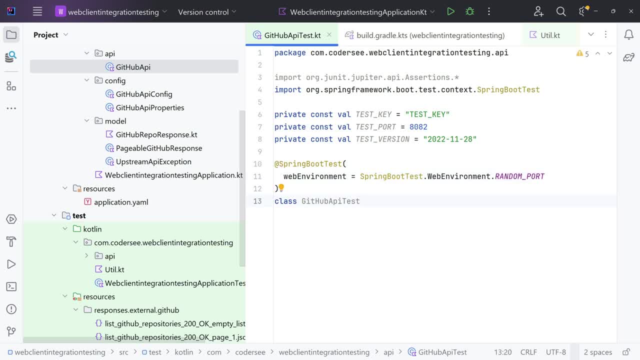 So, basically, we use this annotation for Spring Boot integration tests And this way a new application context will be created. In our case, we set the web environment with a random port value so that a reactive context listing on the random port is created. 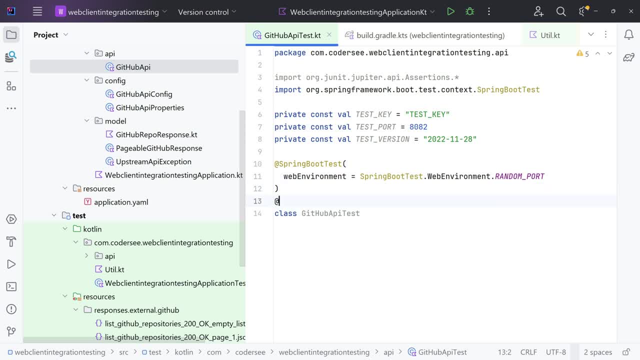 Nextly, let's add test property source, test property source, And right here we can provide the properties as an array properties, array of string values: API dot GitHub dot. URL. Remember that it must match the value. Match the value from our application YAML file. 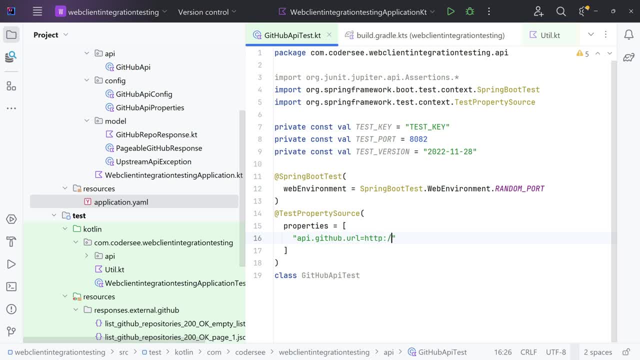 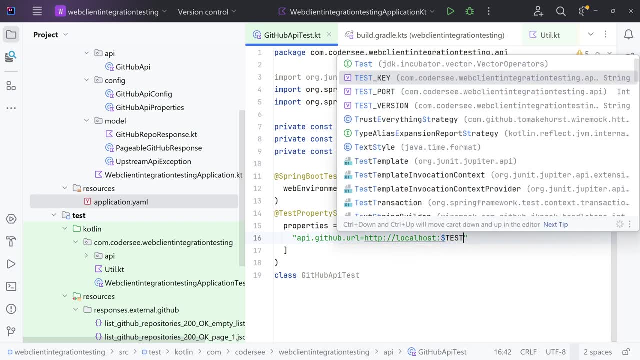 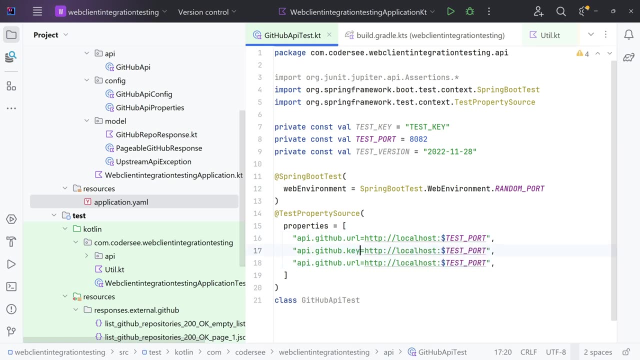 And right now equals HTTP slash, slash local host and the port will be test port. Let's add a colon Ctrl-Plus-D two times. First, I would like to add the key. The key will be nothing else than the test key. 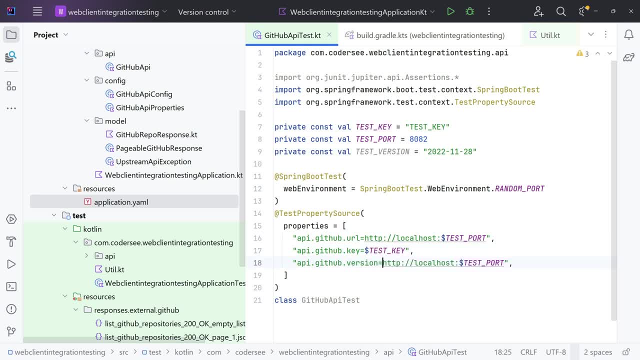 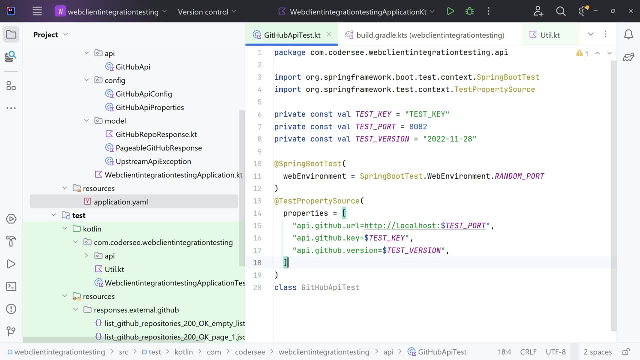 And similarly the version. And that's it. This will be the test version. Ctrl-Alt-L. wonderful. So, as you can see, this is the way we can provide the values for application properties, provide the properties for our application context. 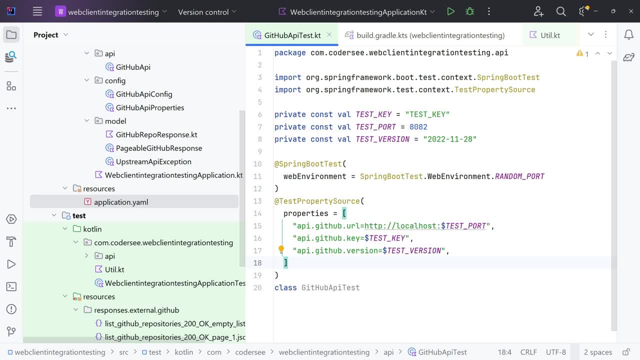 Lastly, let's add the auto configure wire mock. Auto configure wire mock And the port equals Test port. So thanks to this one, the wire mock server will be started as a part of application context. Wonderful. So as the next step, let's inject the wire mock server. 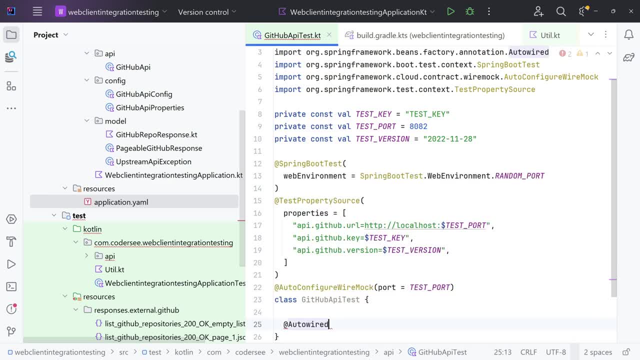 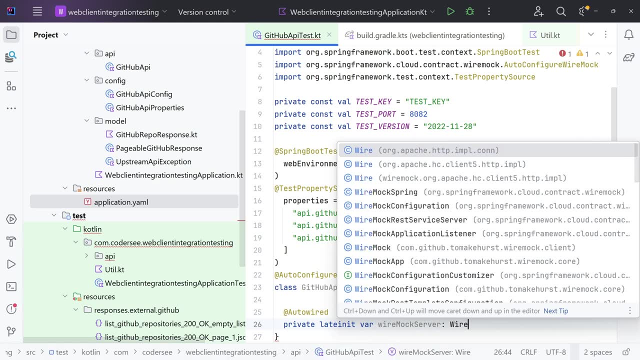 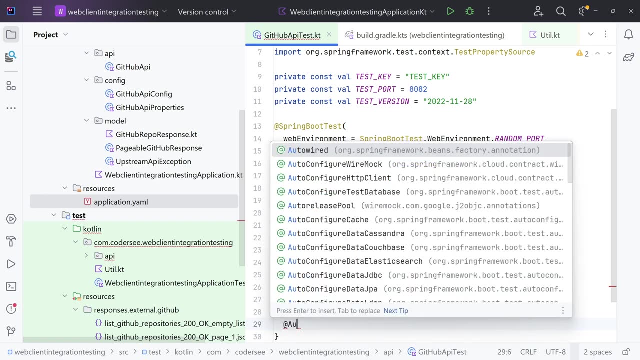 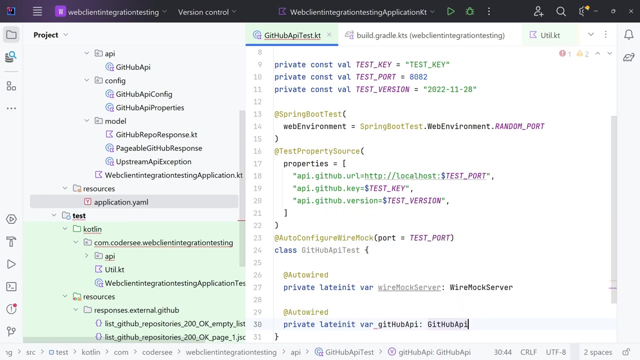 Auto auto wired- Wired- Private Late- init var- Wire mock server Of type wire mock server. Okay, Next let's inject the GitHub API Auto wired, again private late init var- GitHub API of type GitHub API. 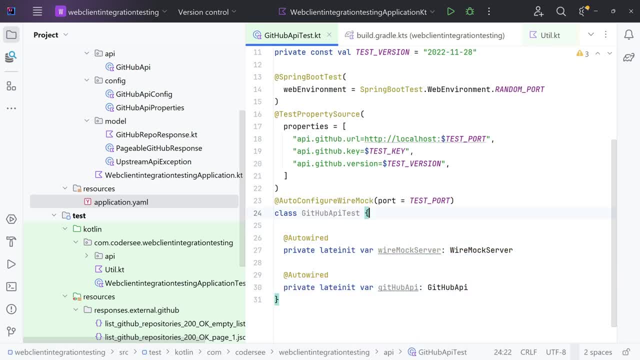 And you can see right now that we can do that, just like we would inject a simple bin in our codebase. Lastly, let's add three properties: the page, the per page and some random user names. So private var page first page. 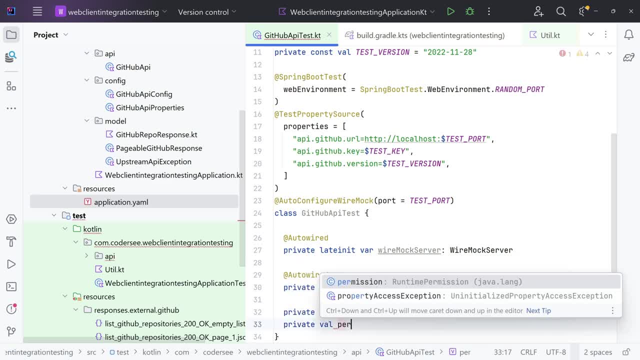 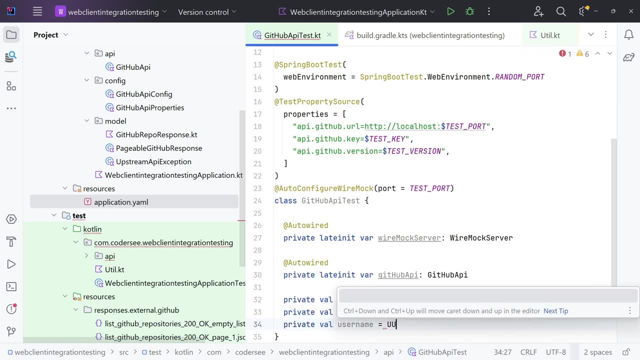 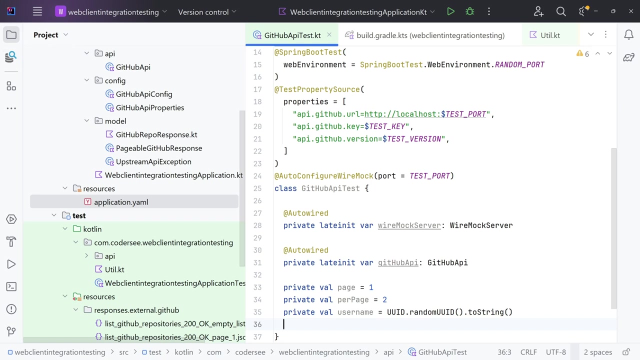 Private var page- First page. Private var per page will be two And private var username equals UUID- random UUID- two strings. So simply, every time the GitHub API test classes instantiated, instantiated, the random username will be generated. 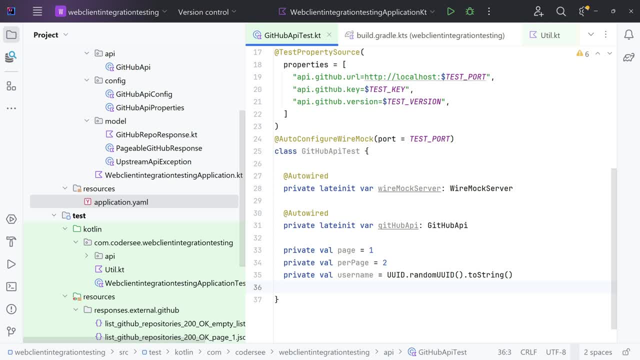 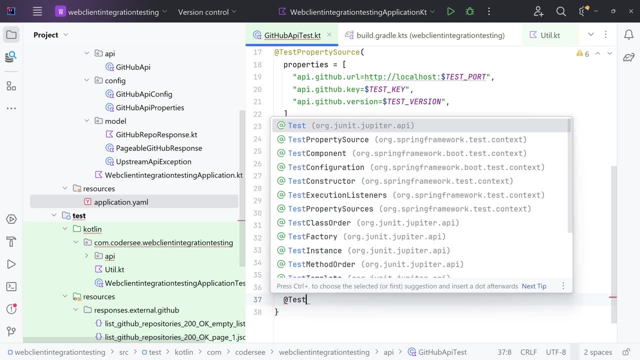 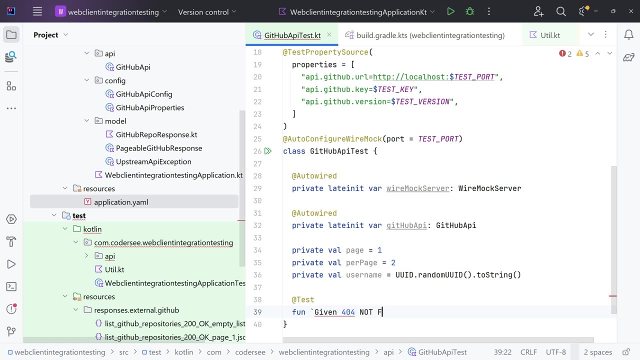 So at this point we can start with the 404- not found case. So let's add a new test. I will use the given when name approach of naming Test found: given 404: not found. response when fetching repository by username, then should: 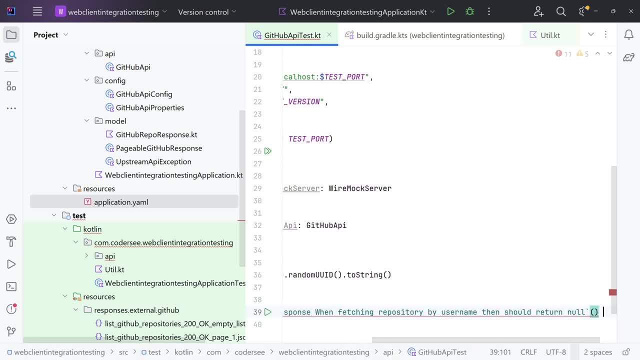 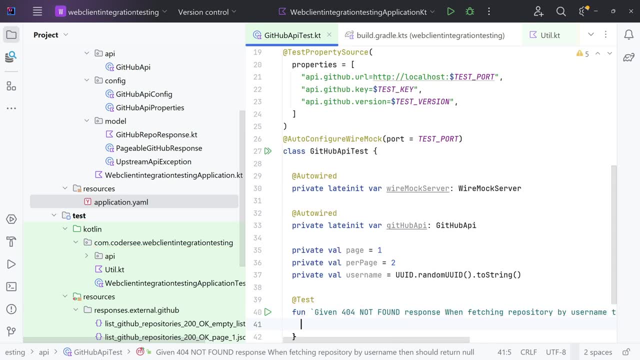 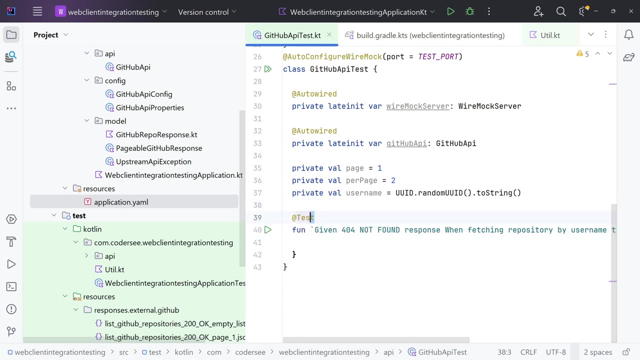 return null. Let's close that Wonderful And let's use the run test. Run test- excellent, because we are dealing right now with coroutines. So at this point we can see that we simply annotate the test just like every JVM needs. 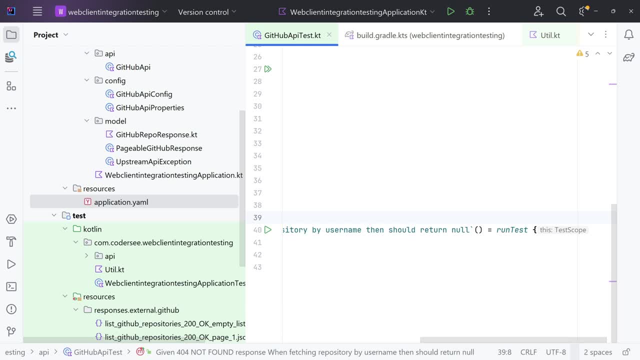 test and we use the run test. Long story short on the JVM. this will be working the same as the run blocking block. Nextly, let's add some stubbing for wiremog, which is nothing else than the ability to return. can't HTTP response for request matching criteria. 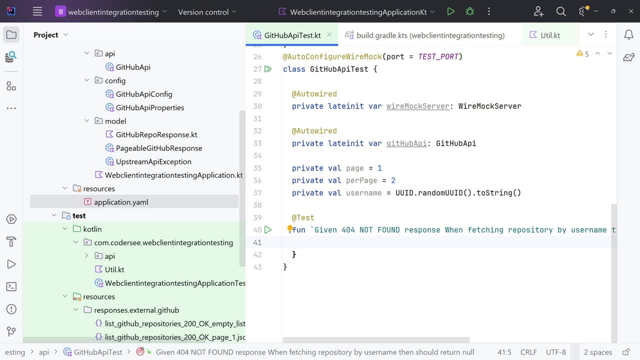 Simply said, whenever an outgoing request that matches our criteria is made, a mocked response configured with will return is returned. So let's start with given, to clearly divide our code here. wiremog server stub for- and. right now I would like to add a stub for the request to GitHub API. 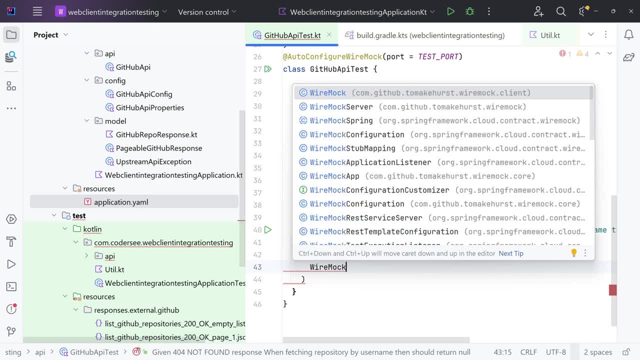 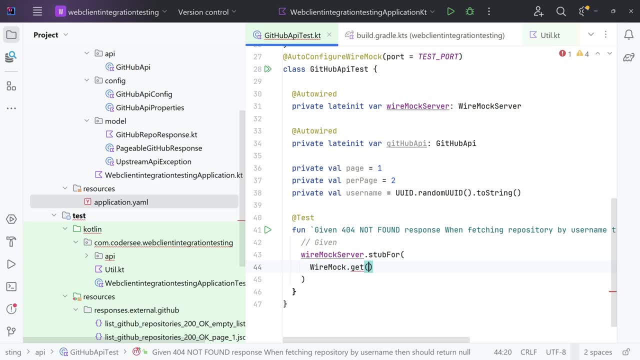 And this was a get request. Wiremog dot get and I would like this URL to be equal to particular URL. So wiremog dot URL equal to, and right now we specify the URL And this was slash. users username repos page equals URL. 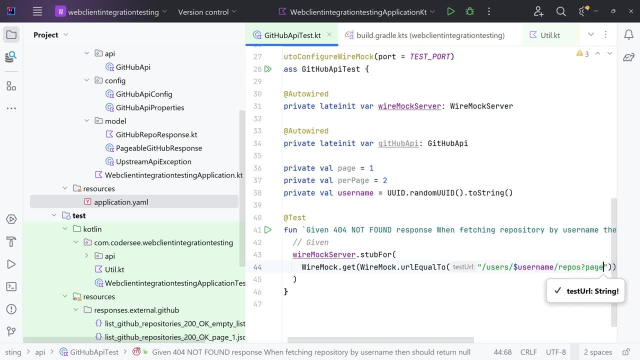 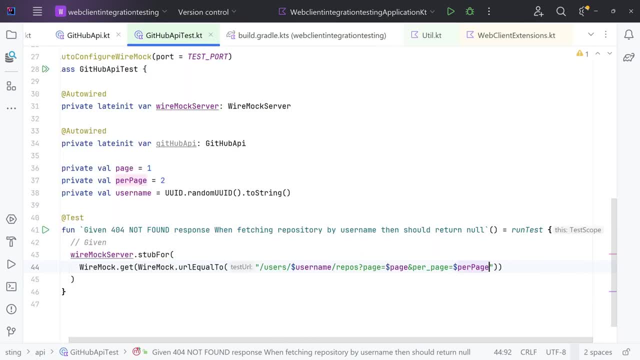 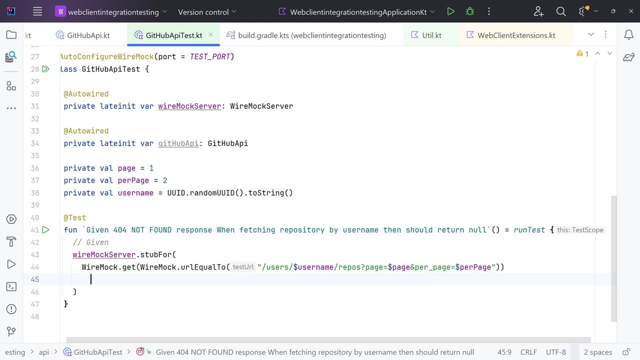 So we can see that with this line of code- let me close this sidebar- we can see that this line of code will match the stub for every request outgoing to the slash users, with the following parameters: Nextly, I would like this stub to work only for particular authorization Requestasser. 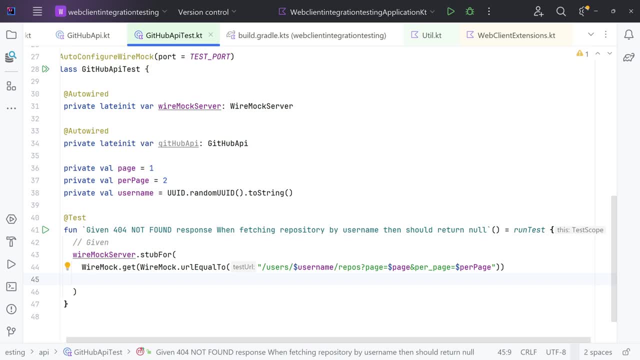 header api version and the accept header. so, with header authorization, let me double check authorization. okay, wire mock equal to and the value. i would like this to be better. test dot key ctrl plus d to duplicate. and let's match the another header, x, dash github, dash api. 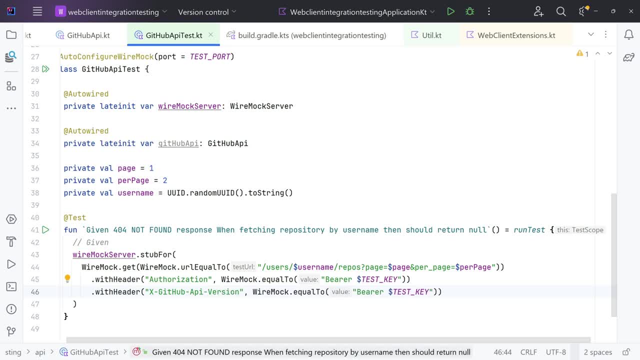 dash version. i would like this one to be equals to test version. ctrl plus d, the accept header. and again this one will be equal to application slash, vnd, github plus json. so again, whenever a request to a particular url- a get request, of course, sorry, with these headers- will be made, we would like to return a particular response. so right now, 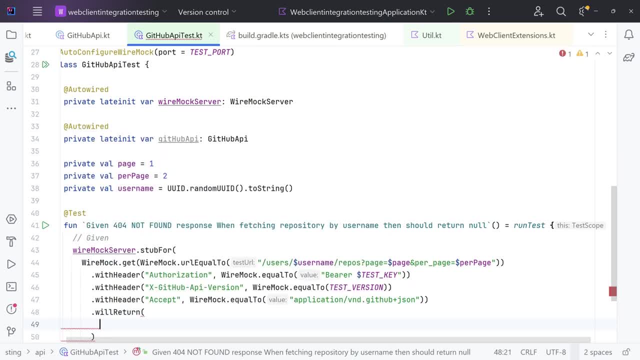 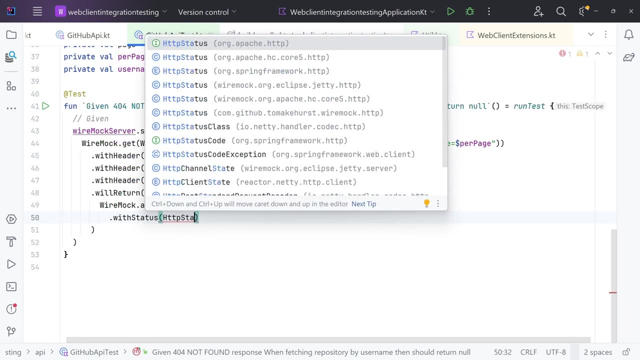 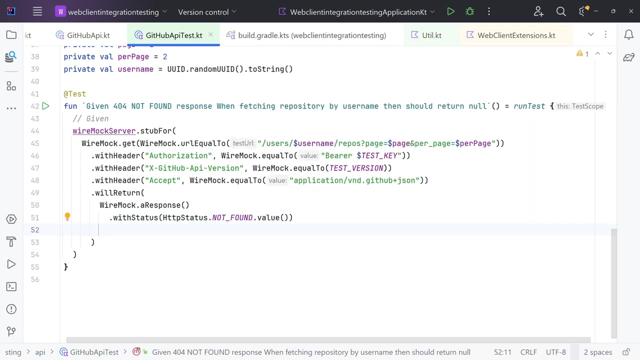 dot will return and will build our response wire mock dot. a response with status. i would like the status to be not found. http status not found value with header: content type dot. with header: http headers dot. content type application: json chart set equals utf dot 8.. 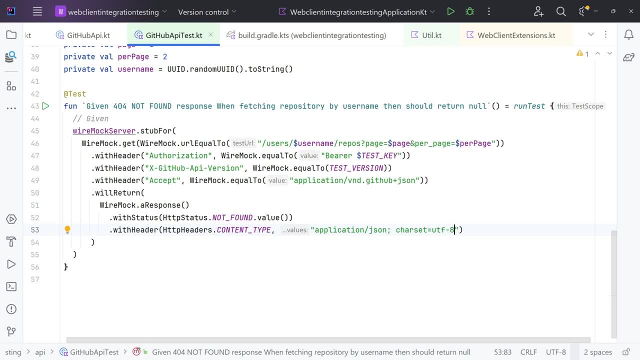 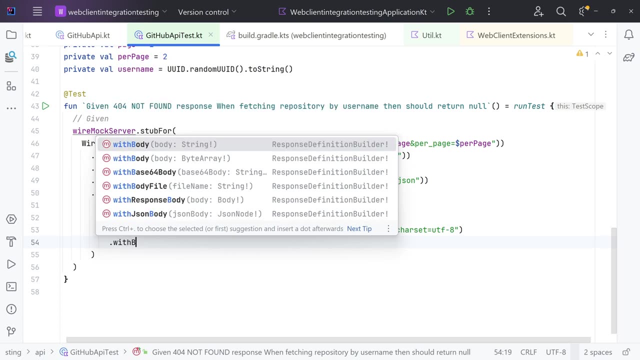 if you are wondering, how do i did i figure out this header? well, basically, from querying the api. As I mentioned previously, we want this to be as close to the real call as possible And right now I would like to provide the body, so withBody. 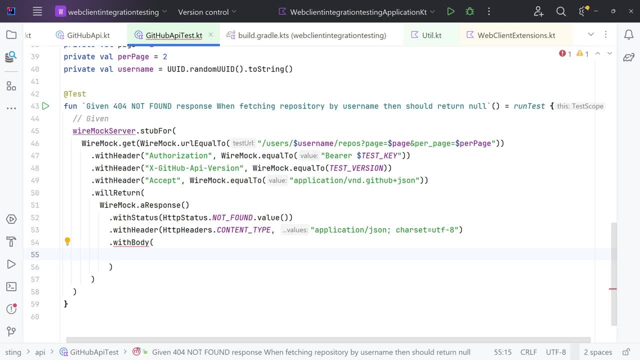 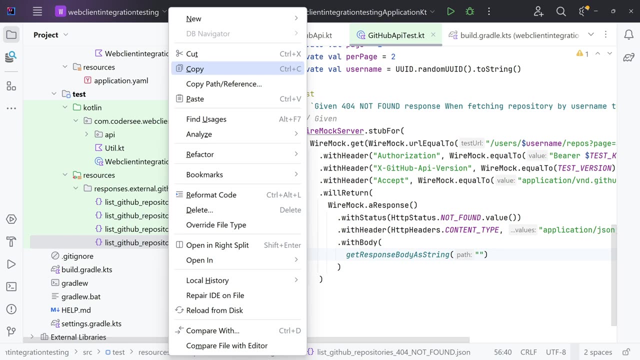 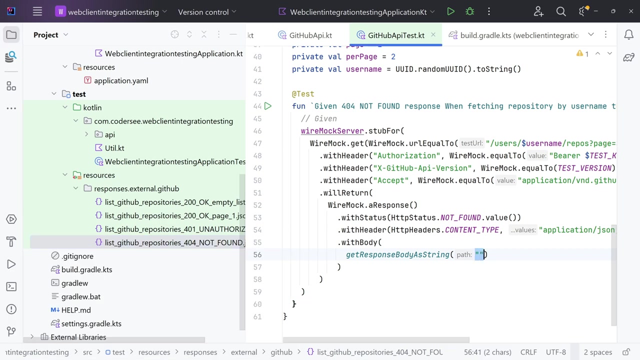 And the body. right now let's use the function that we implemented previously, so getResponseBodyAsString, and we need to provide the path. so this will be done the easiest by simply going right here, and let's use this one copyPathReference, and right here we'll use this. let me double. 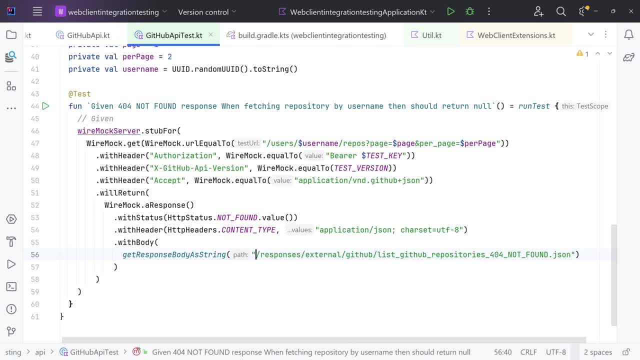 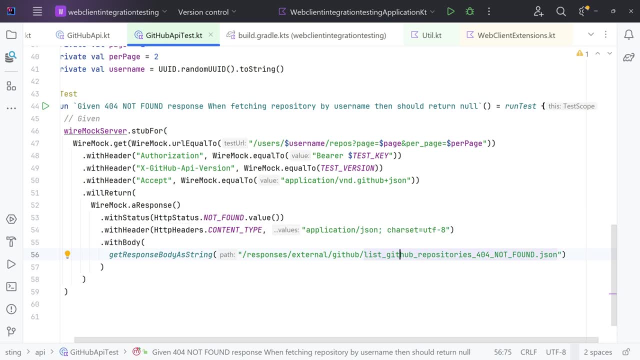 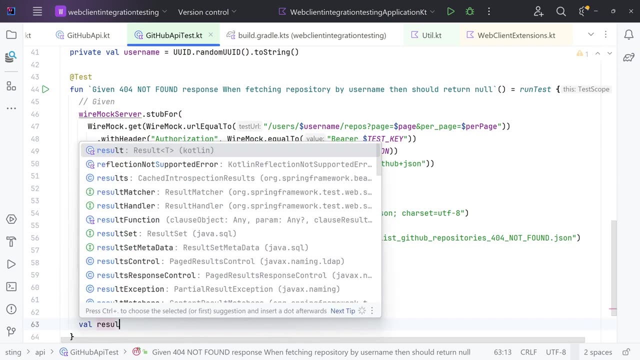 check. However, we don't want the resources, so this will be responses- external github- and we'll be navigating to our file. Wonderful, With that done, we can simply invoke And then, well, result equals github API list repositories by username and we'll provide. 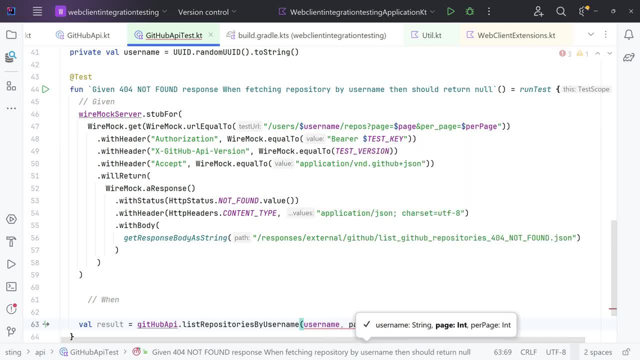 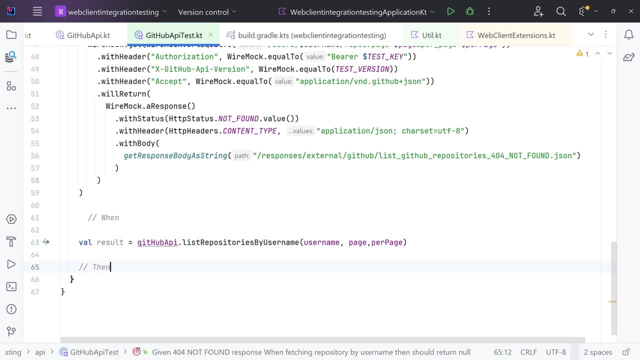 the username, the page and the per page argument. Let me scroll down a bit, then. ctrl-alt-L, maybe to format in the meantime. And, lastly, I would like to simply assert that the result is null, because that's what we implemented previously. 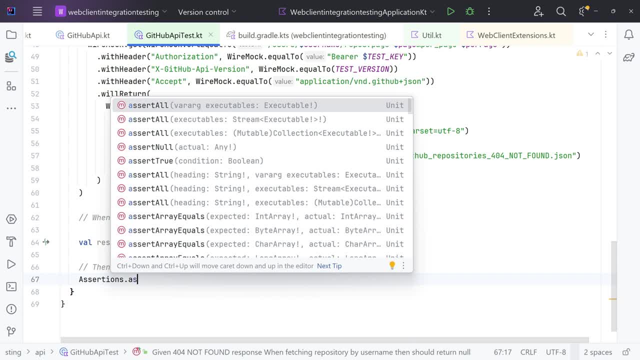 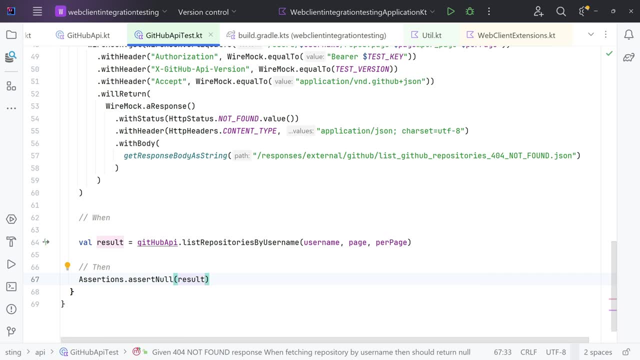 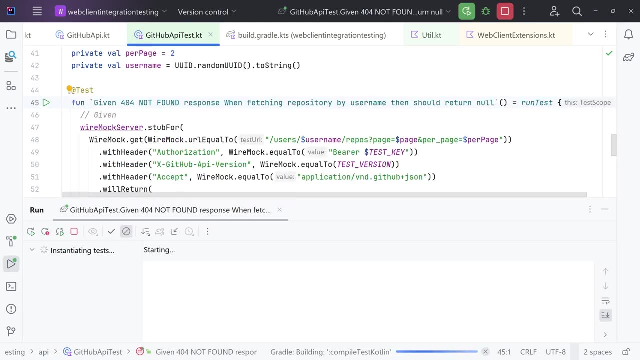 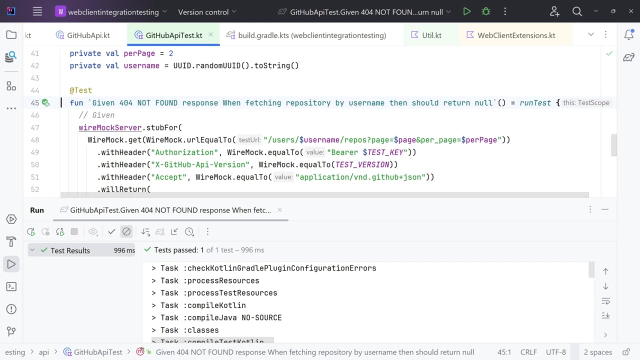 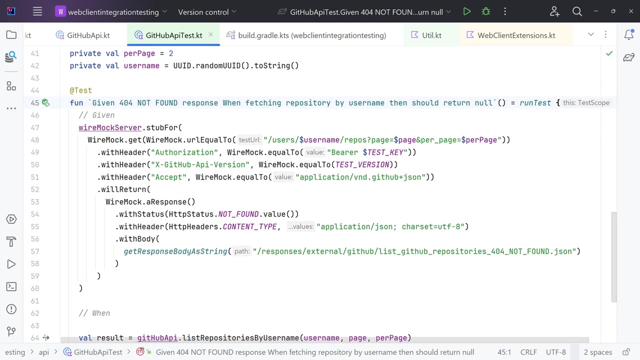 Assertion Assert No Result. Control-alt-L. and let's run our test. And wonderful, we can see that our test passed. so let's rephrase what we learned. right here We can see that We're working with wiremock. 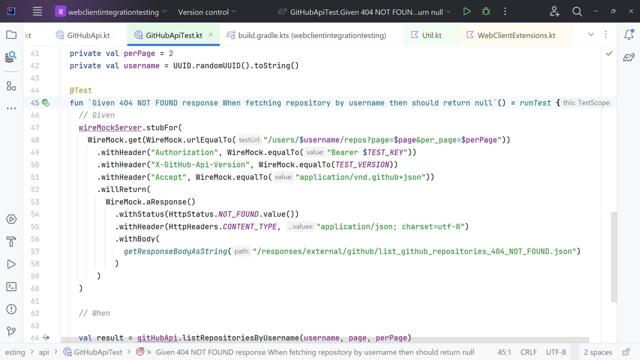 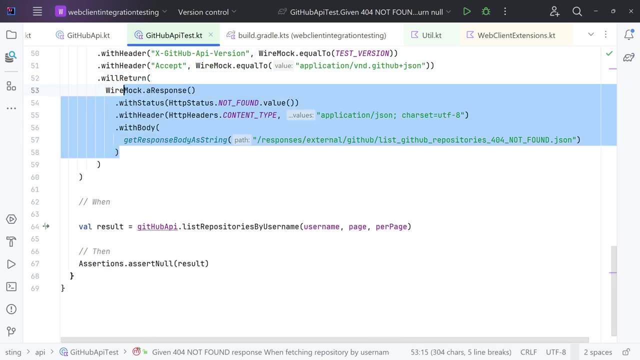 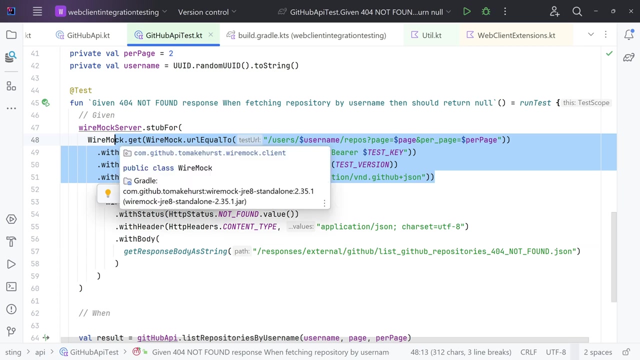 This is pretty similar to any other mocking library. We provide the conditions for which the mock should be created. So whenever we make a get request to a matching URL with matching headers, the particular response will be returned. If any of these does not match well, then the test will simply fail. 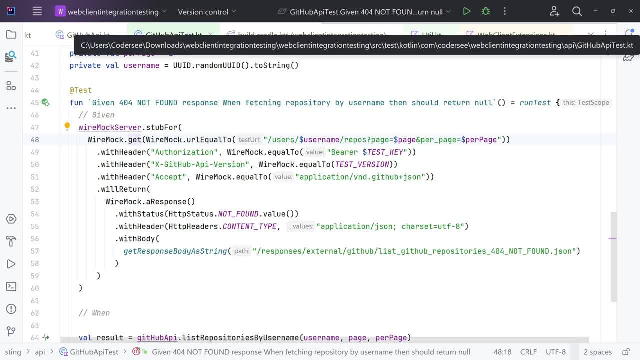 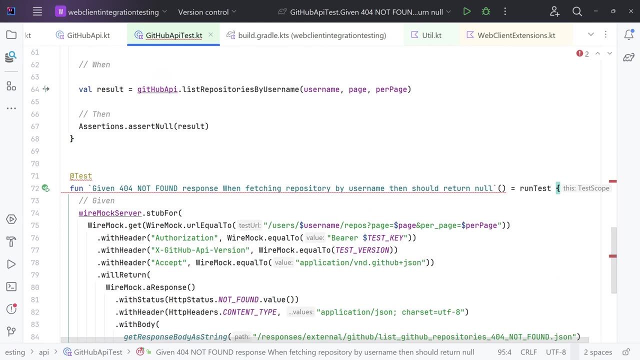 So with all of that being done, we can basically copy this test and adjust that to another case. I would like to test 401- Unauthorized, which would throw the upstream API exception. So let me copy all of that And let's change the name. 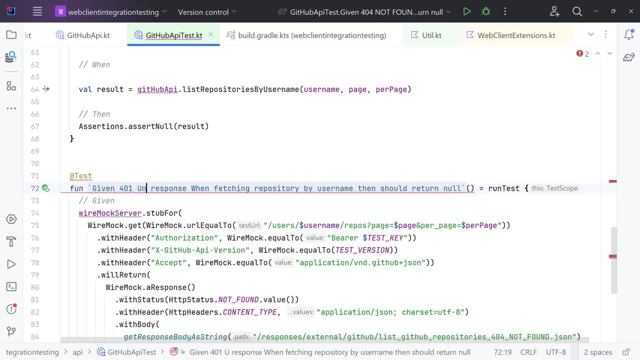 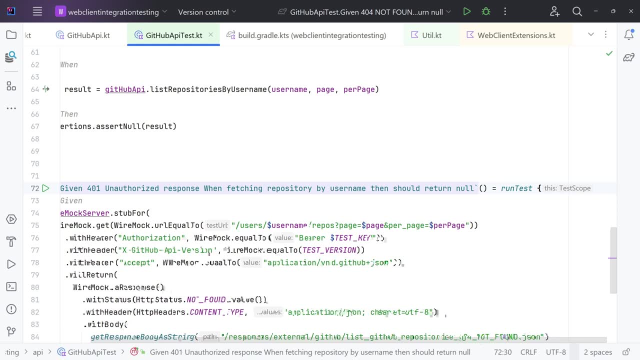 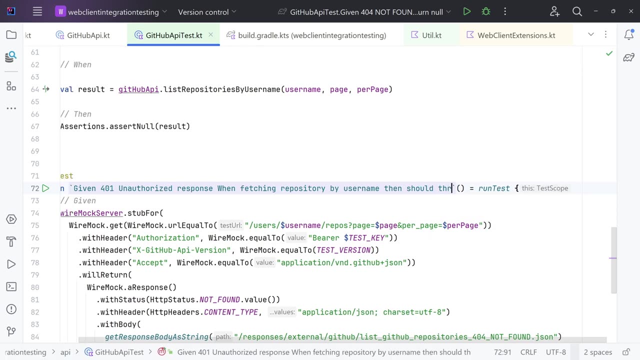 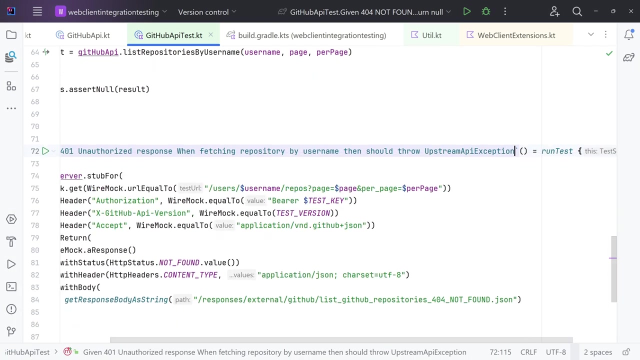 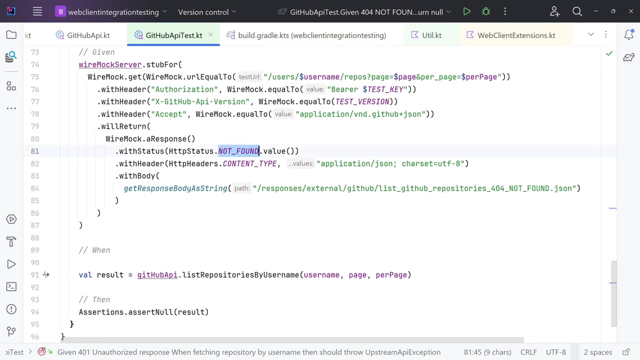 Given 401- Unauthorized response when fetching repository by username. Then should throw upstream API exception. Then should throw upstream API exception Again. we'll be running the test. We'll be stubbing, But this time the response will be slightly different. First of all, the status will be 401- Unauthorized. 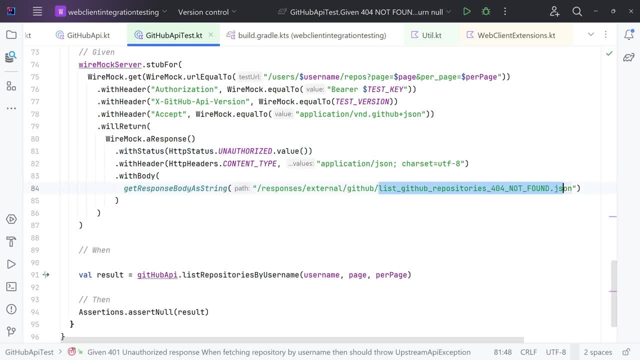 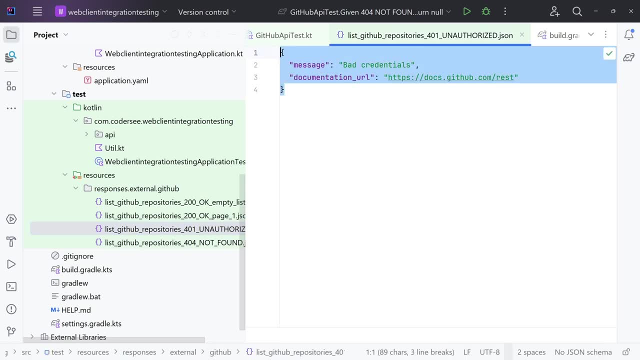 The header value will be exactly the same. However, this time we'll be referencing to other file. Let me copy the file name: 401: Unauthorized. as I have shown previously, bad conditions. Right here I can copy the name with Ctrl plus C. 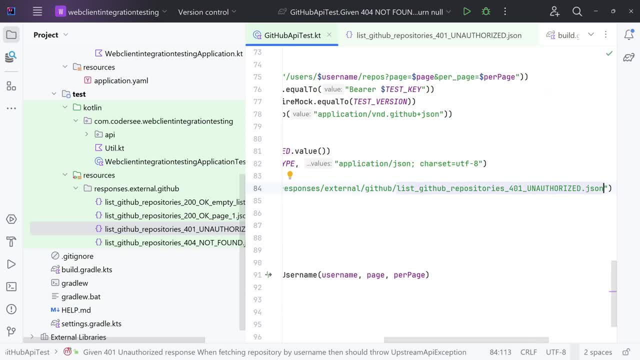 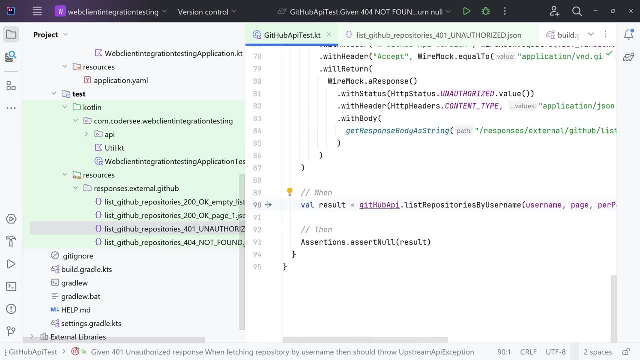 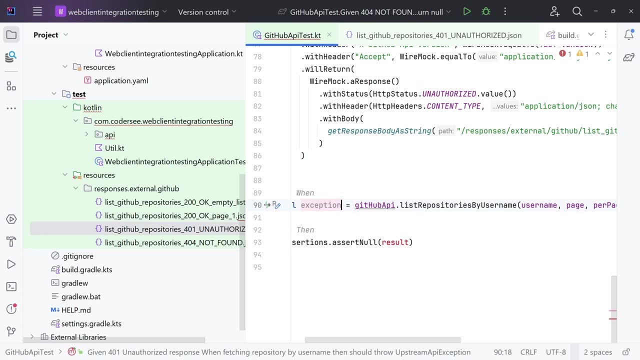 And get back to the test And provide this value right here. Wonderful This time. instead of result, I'm interested more in the exception itself. So Instead of result, let's call it exception. github API. Let's hit Ctrl plus X to cut the value. 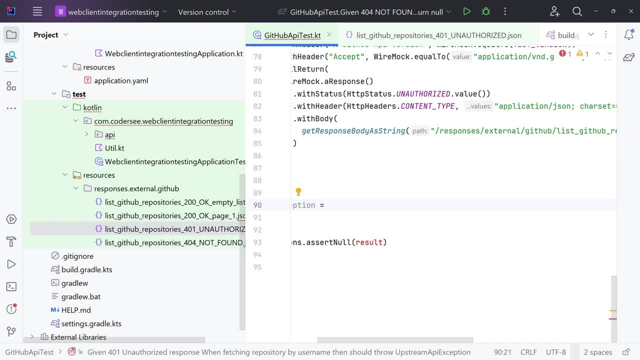 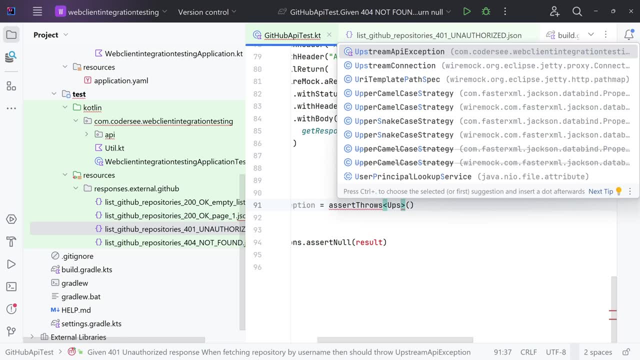 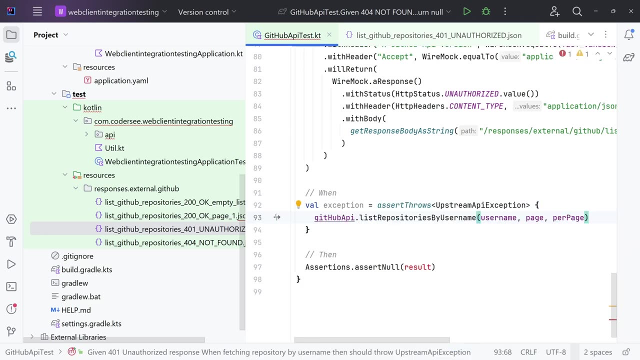 And this time I would like to assert that it throws the upstream API exception. Assert: throws upstream API exception. Upstream API exception. Let's open up brackets And invoke our function And we can see that the exception is not in it. So 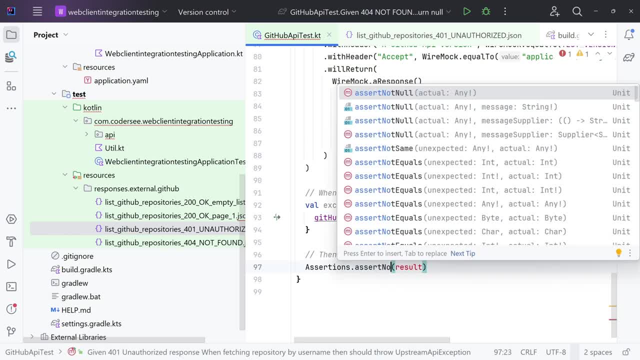 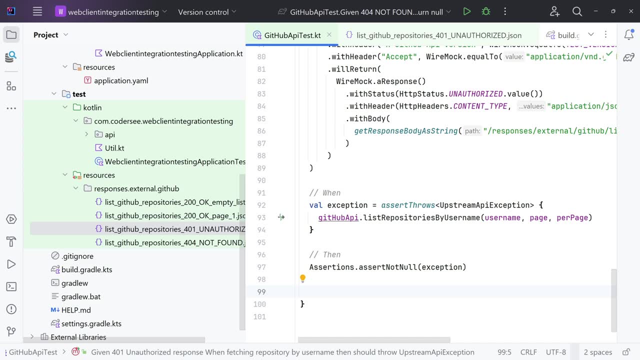 Lastly, I would like to assert that this is not null. I would like the exception to be thrown. So Assert, Not Null The exception. And lastly, let's simply assert the exception and the status code: So Assert. 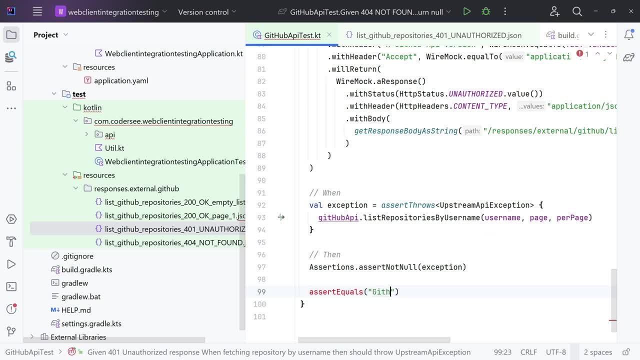 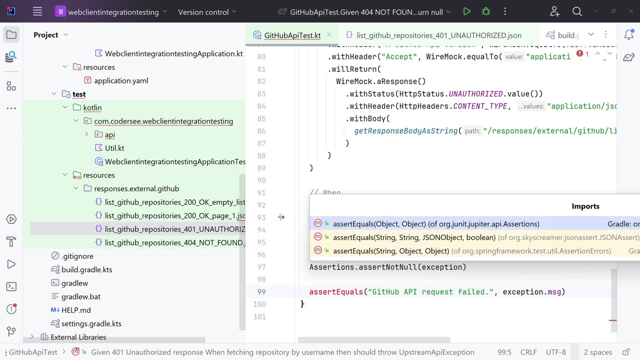 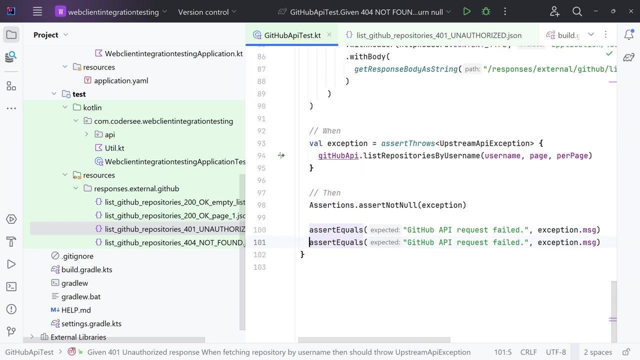 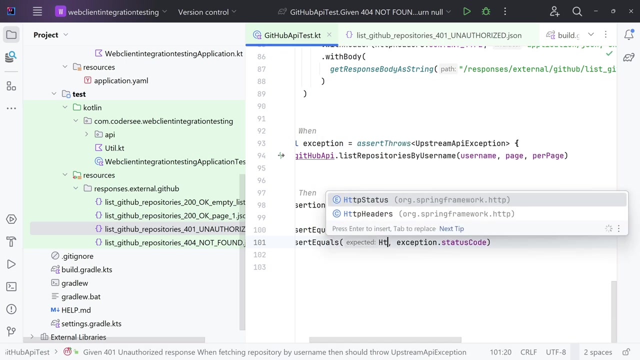 Equals. Github API Request Failed. What No Failed With dot. Exception, Dot Message. Alt plus enter And let's import the correct one from orgjunitjupyterapiassertions: Ctrl plus D And exception. status code needs to be equal to unauthorized. 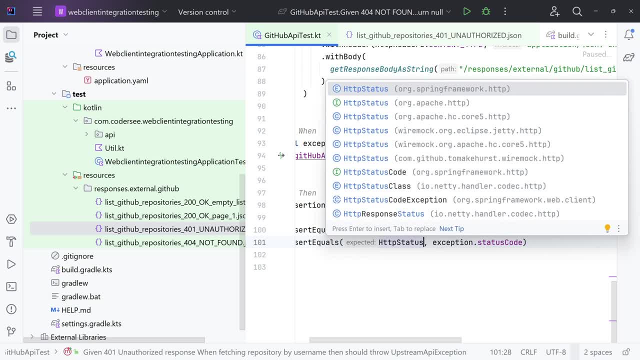 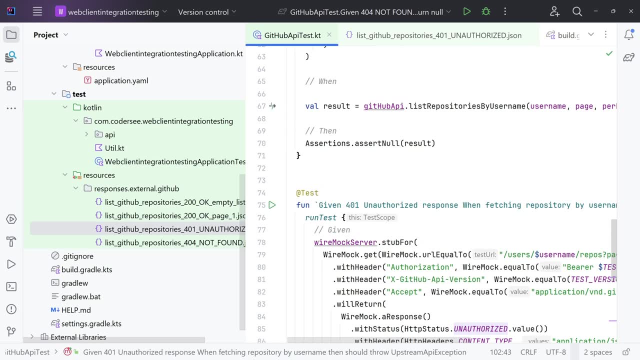 Http Status. Coup From status From springframeworkunauthorized- Ctrl Alt L. Now Let's simply run this test. Wonderful, We can see again that this test passed. So This function is useful whenever you are working with any code that needs to throw the exception. 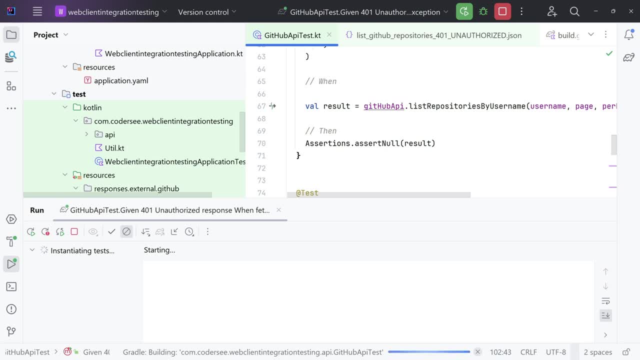 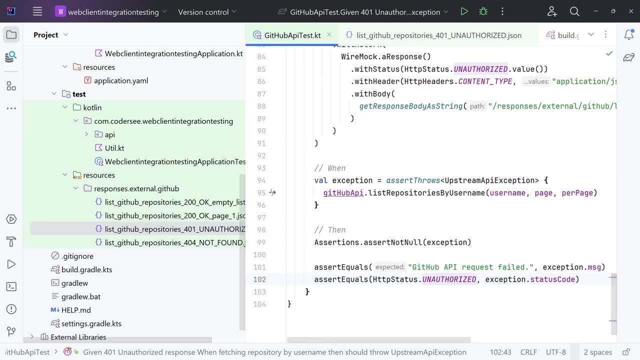 To Not only assert that the particular exception is true, But Also To Assert That The Exception Is True. So Let's run this test. Wonderful, We can see again that this test passed. So 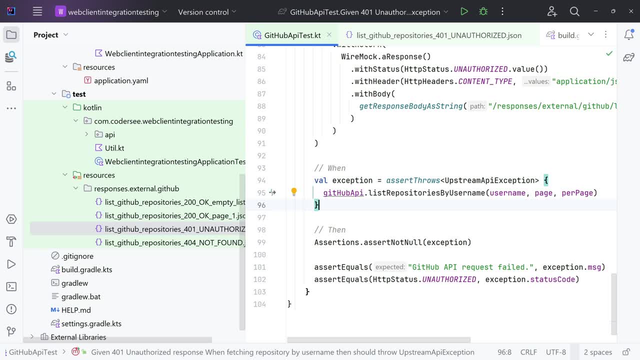 This function is useful whenever you are working with any code that needs to throw the exception To Assert That The Particular Exception Is True, But Also To Get The Object Of That. 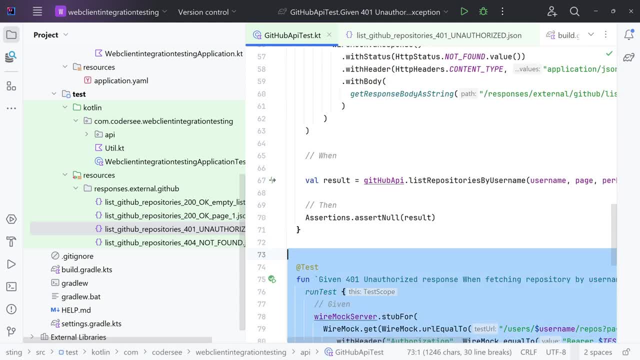 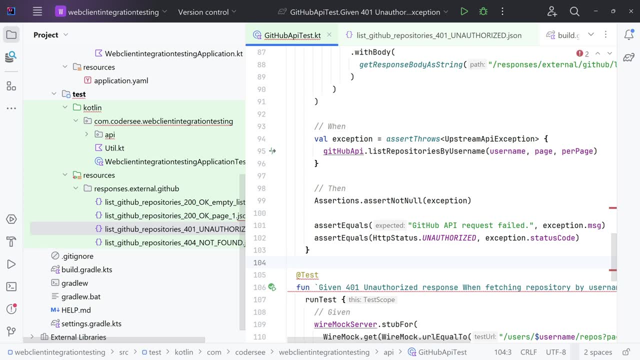 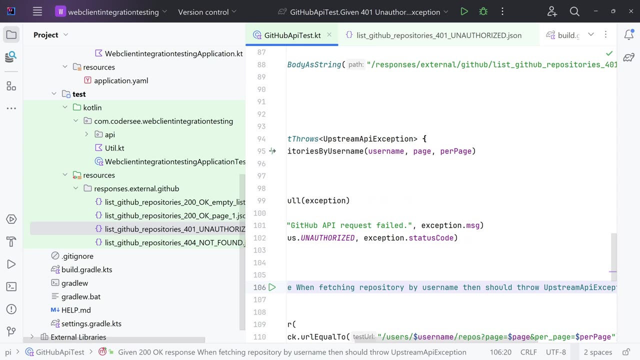 Exception. With that done, Let's verify that we can get 200 OK with empty list. So Again, Simply Copy, Paste Or Ctrl Plus D To Make Response When Fetching Repository. 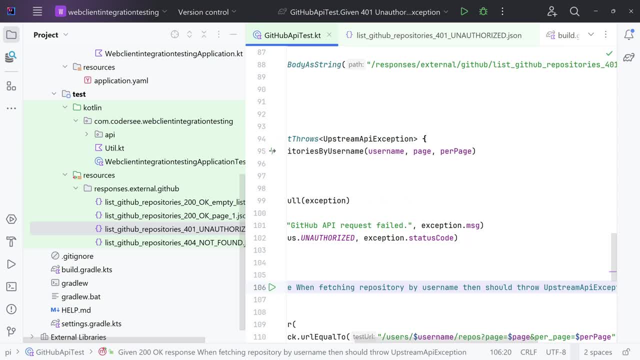 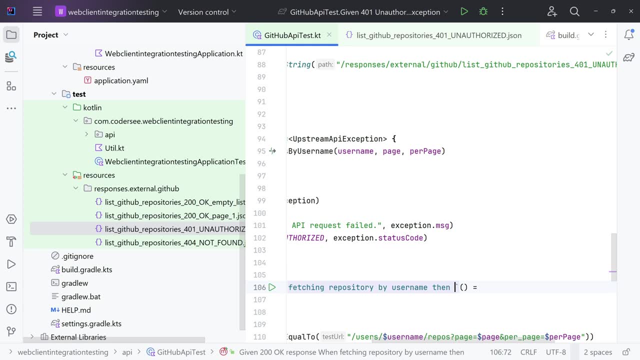 By Username. Then Should Return Repository With Correct Properties And Has Next Set To False, So Let's Write This Explicitly. Then Should Return Repository With: 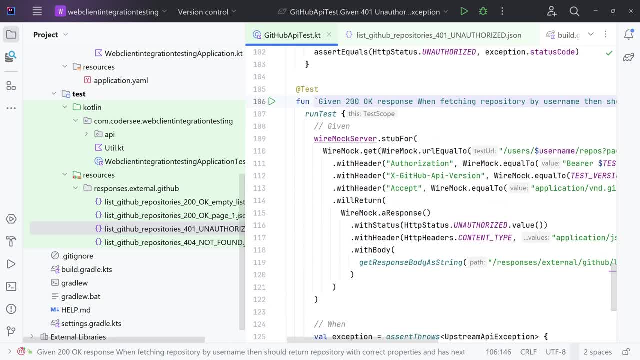 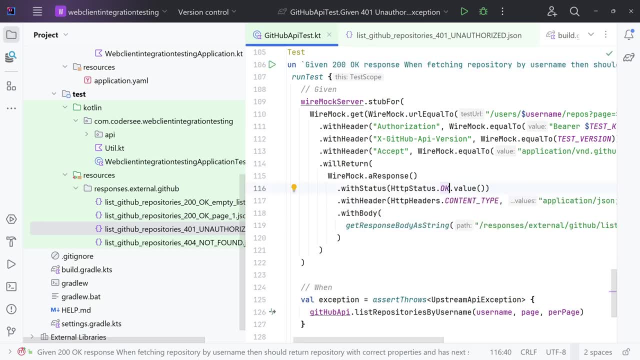 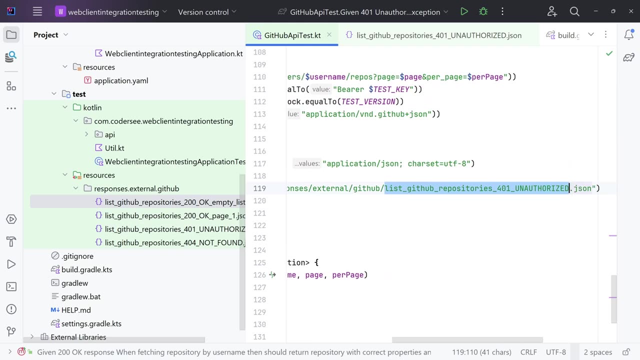 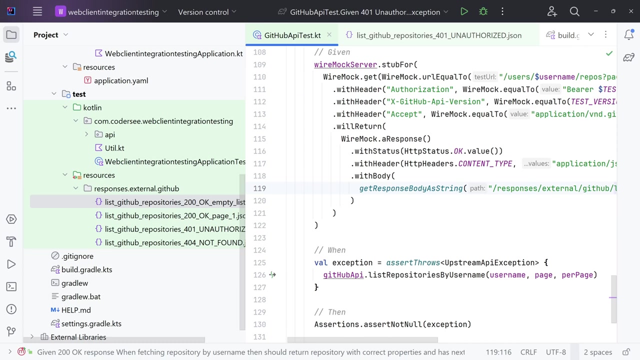 Correct This Time. Whenever We Are Getting This URL, We Would Like To Return Status Code: OK, 200, OK. The Same Header And This Time The 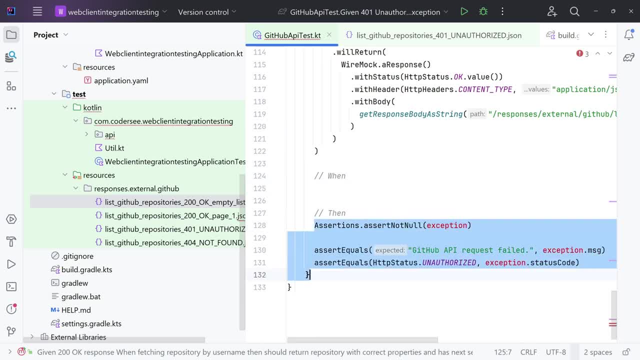 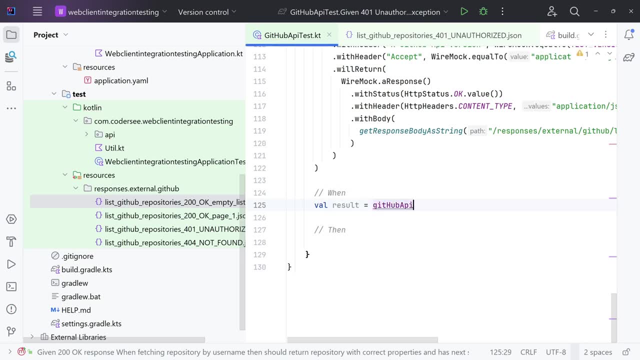 Response: Barrier String Will Be Repository With Correct Properties. Val Result Equals GitHub API List Repositories, User Name Page And Per Page. And Lastly, I 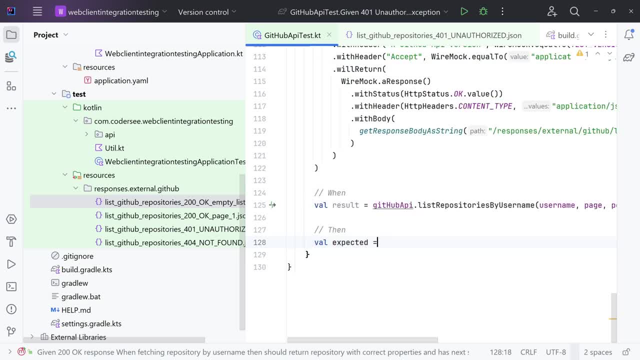 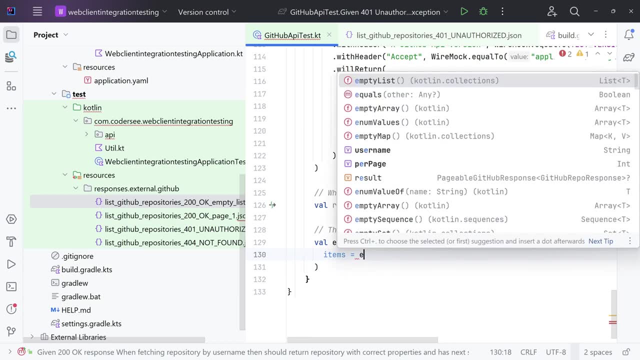 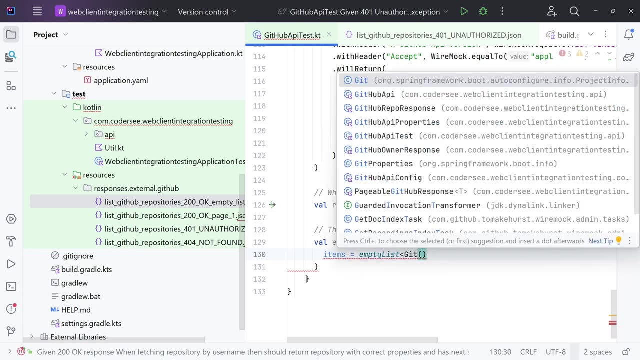 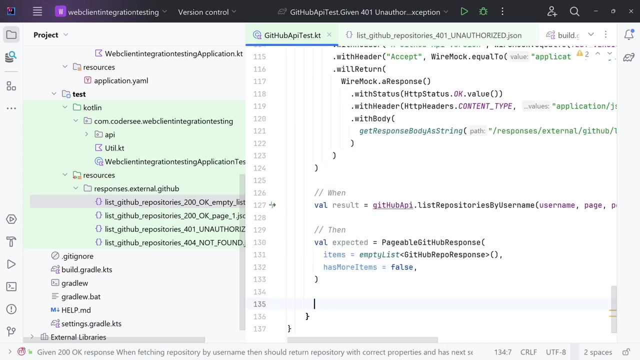 Would Like To Assert The Expected Pageable GitHub Response Is List Of GitHub Repo Response Empty List Of Type GitHub Repo Response And Has More. 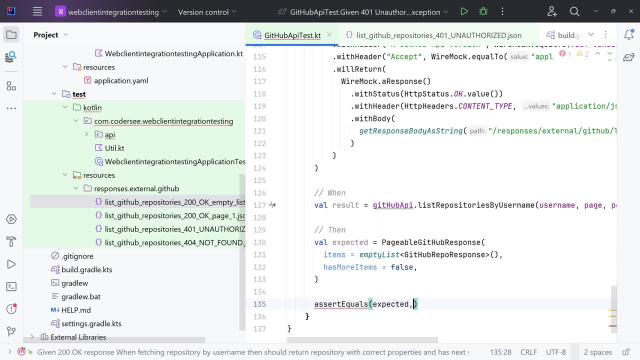 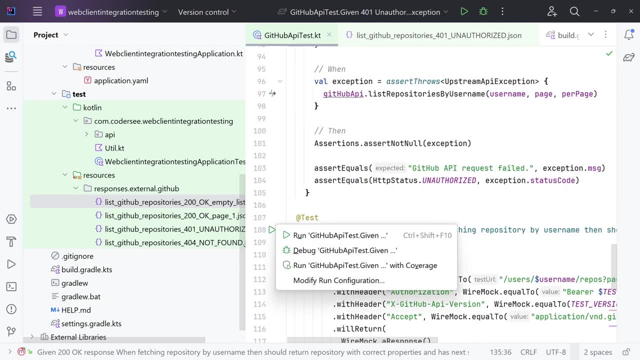 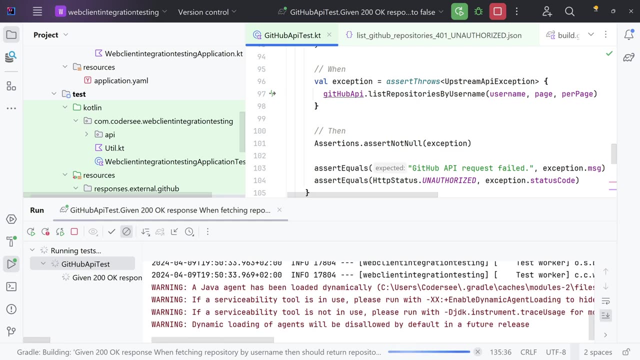 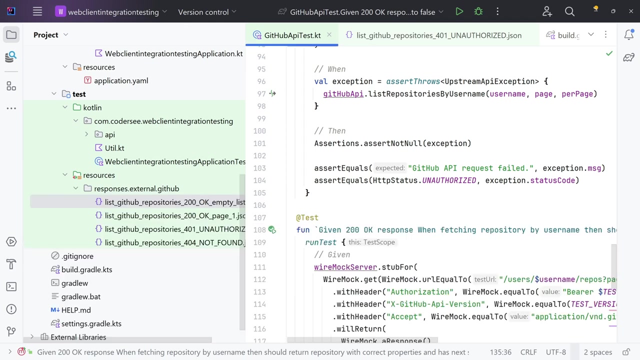 Will Be Set To False. Lastly, Assert Equals Expected And The Result Control Alt L As The Next Test Case, Let's Figure Out The 200.. 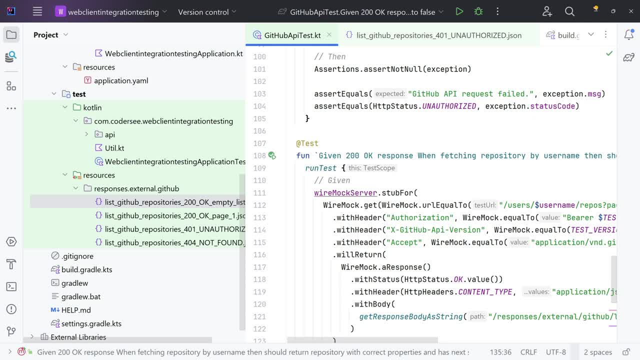 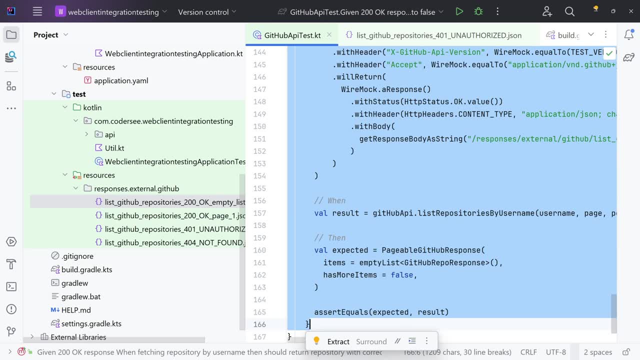 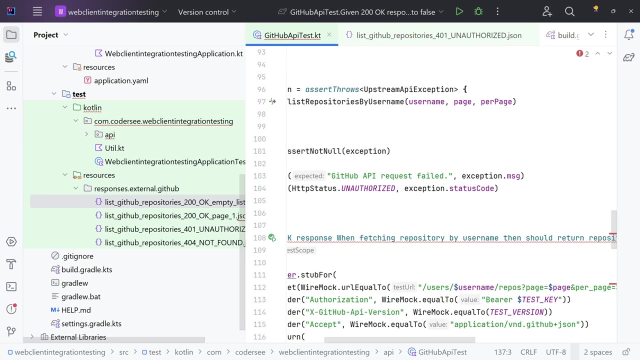 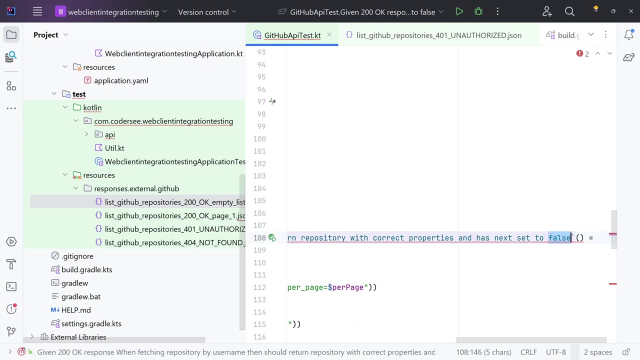 Okay With Has Next True. So Let Me Copy This Control Plus D: Let's Hit Enter, Give It 200.. Then Should Return Repository With Correct. 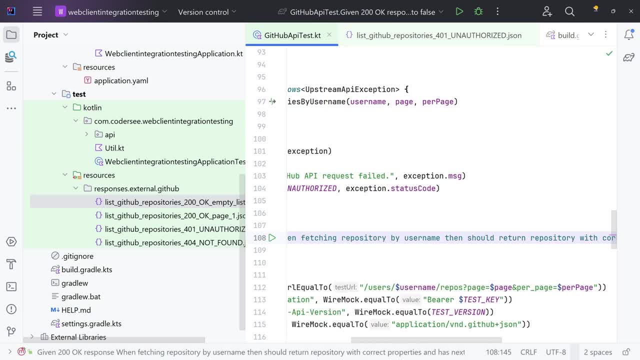 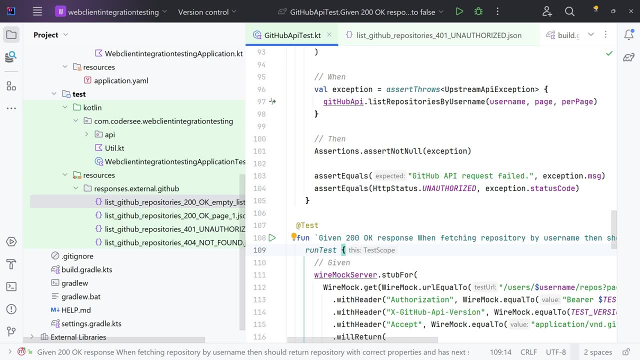 Properties And Has Next Set To True Instead Of False. And In Order To Fulfill That, Well, We Need To Add The Link, And Let's. 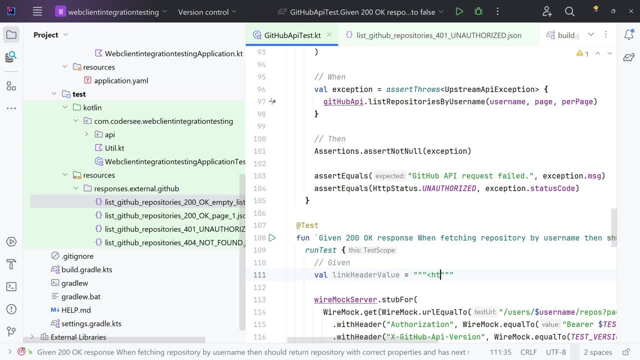 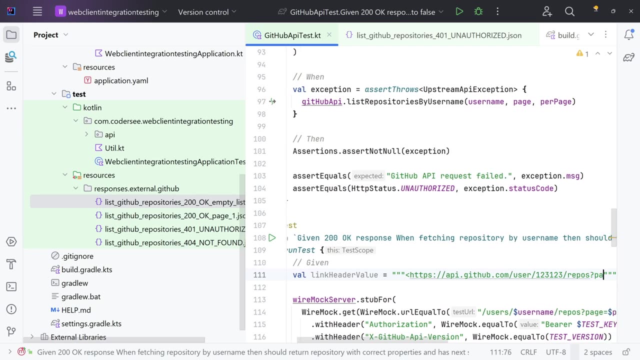 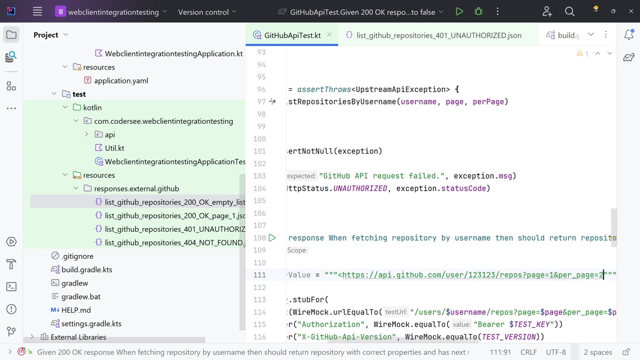 Use That Https Slash Slash API, Github Dot Com Slash User, Slash Some Id Slash Repos Page For Example One, And Per Page Equals To: 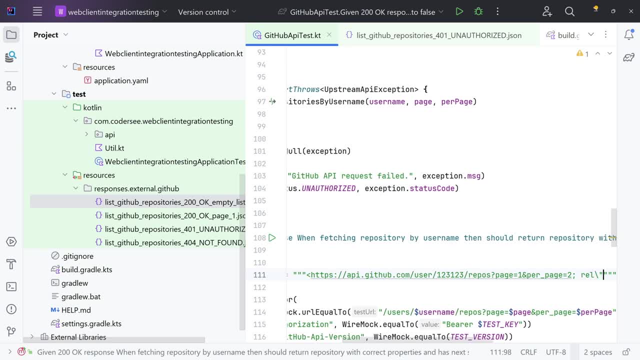 Well, It Has Equals, Equals Next, Wonderful. Let Me Close That In The Meantime. Basically, Again, This Is The Copied Value That I Saw. 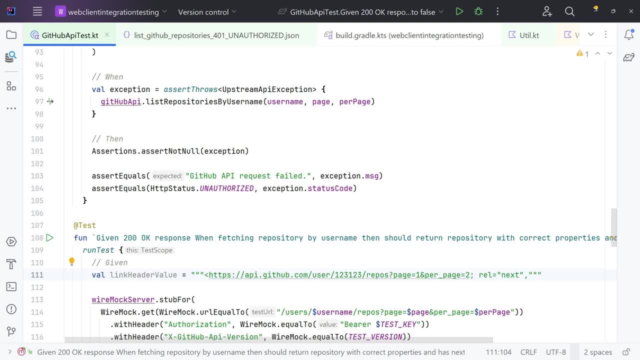 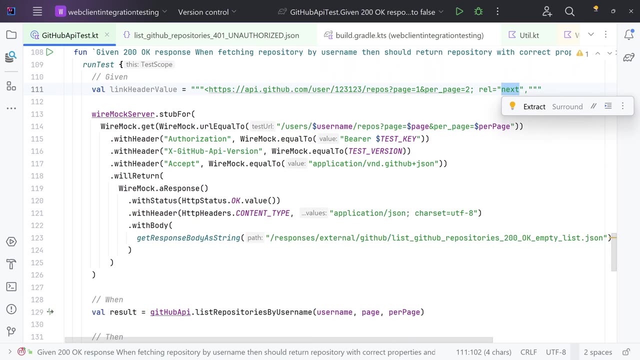 But Technically, To Test That Case You Could Simply To The Real Cases As Possible. So Right Now, Our Response: Return The Ok, Value Return. 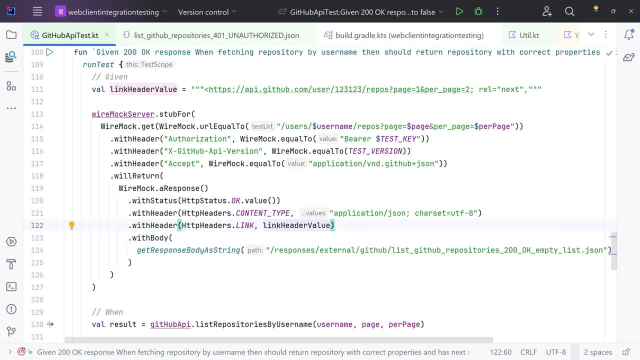 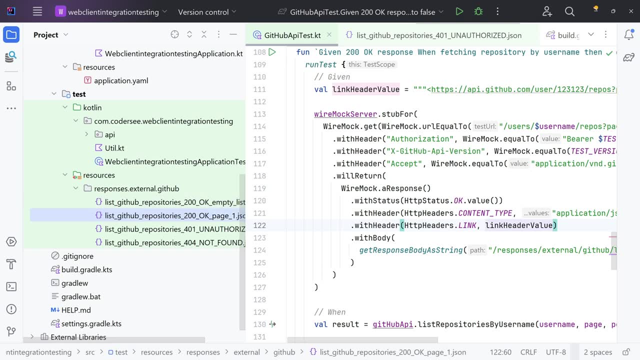 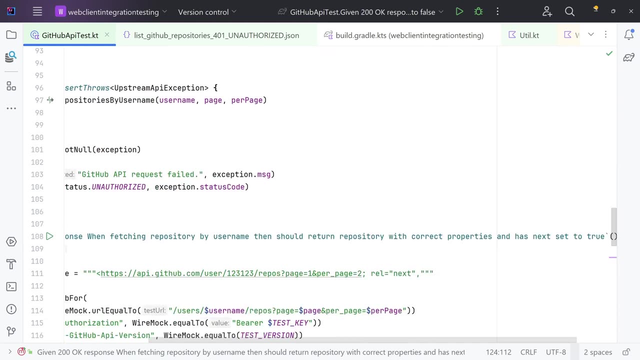 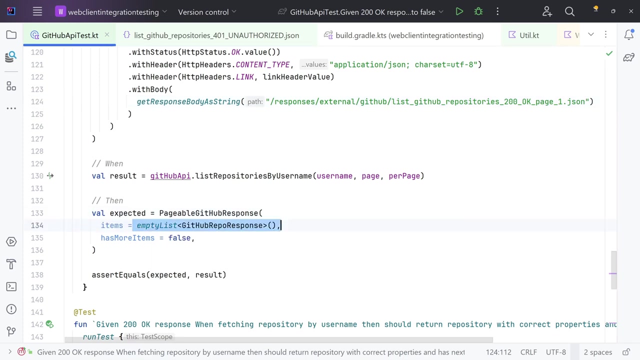 The Content Type. But Additionally It Will Return The Link Header With The Json List. GitHub: Blah Blah Blah, Page One Json And This: 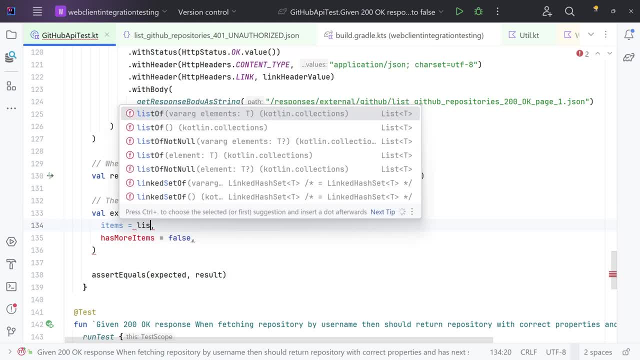 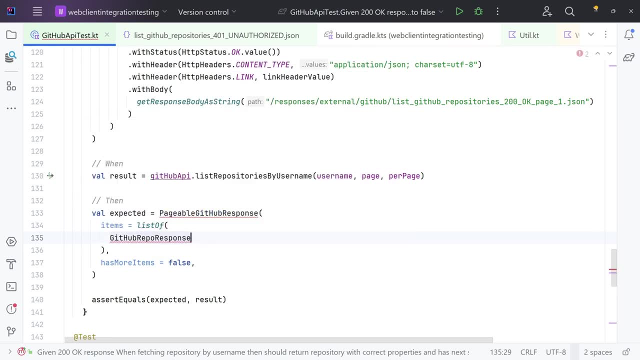 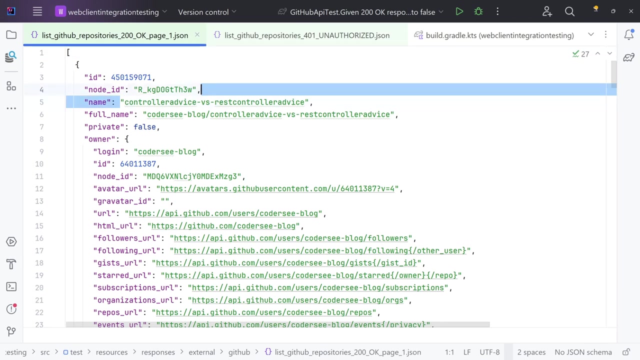 Time. This Will Not Be The Empty List, So I Need To Simply Provide The List Of This File. You Can Hit Control And Keep It. 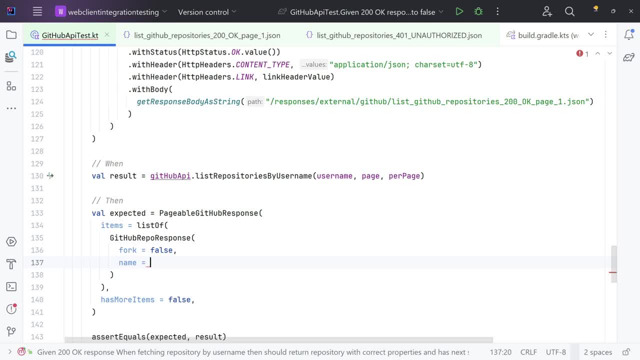 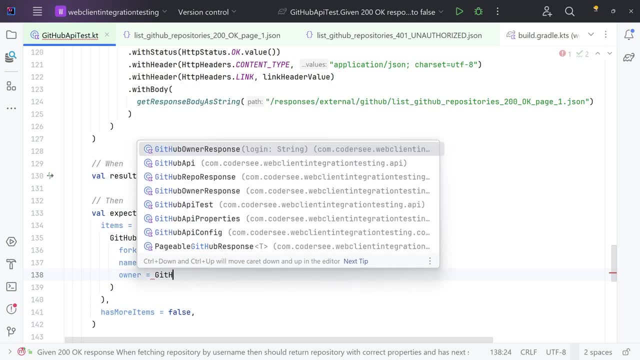 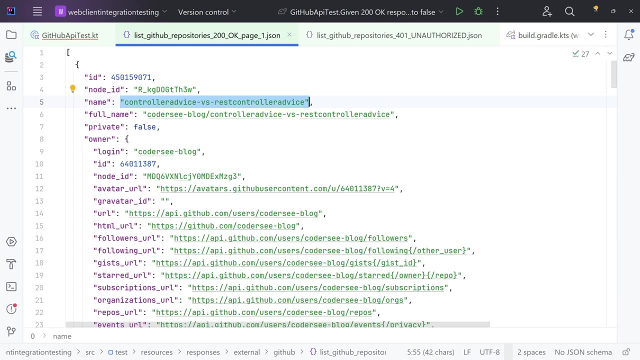 Pressed Left Mouse Button And You Will Be Navigated Right Here. To Make Your Life Easier, Simply Copy This Value. You Can See The. 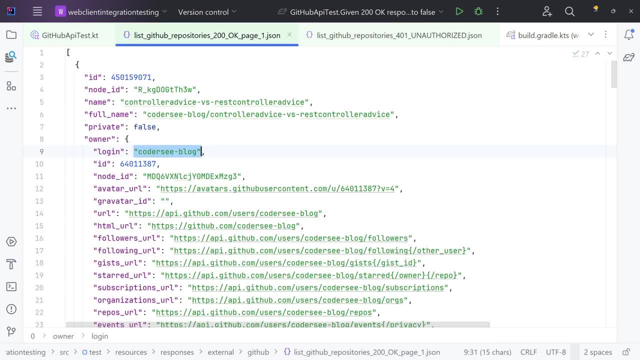 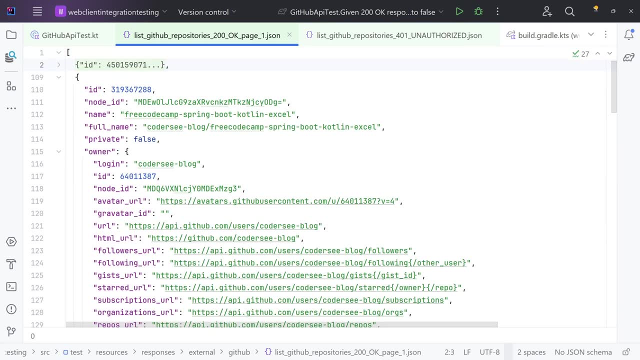 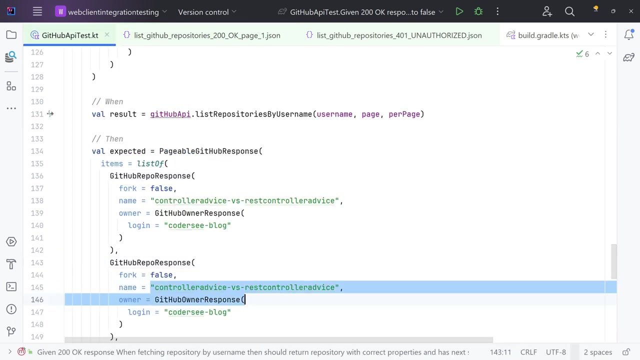 Login, So I Will Copy This Value, And That's All For The First Thing In This List. We Have Two Things: This One And This. 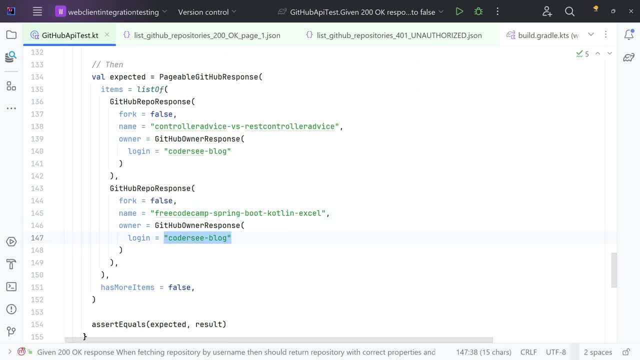 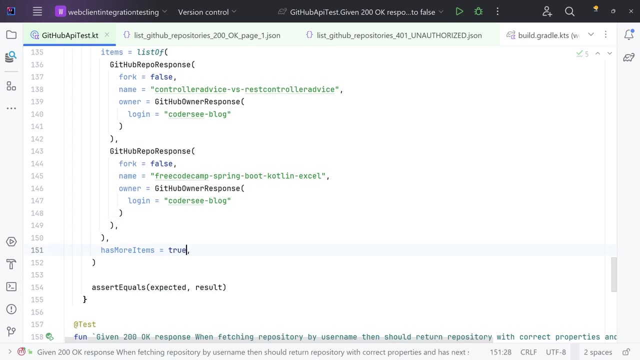 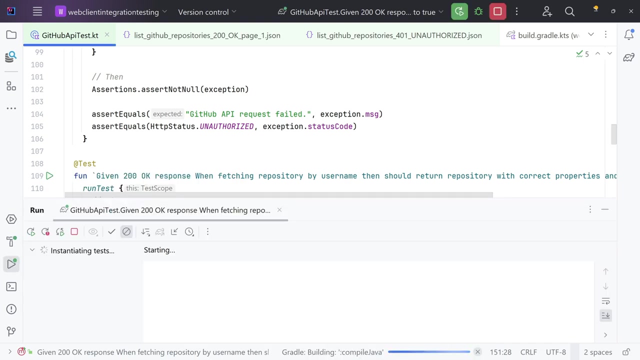 Let's Copy It Here And The Login Will Be Exactly The Same. Let Me Check Whether This Is Fork, Fork, False. And Yeah, This Is.